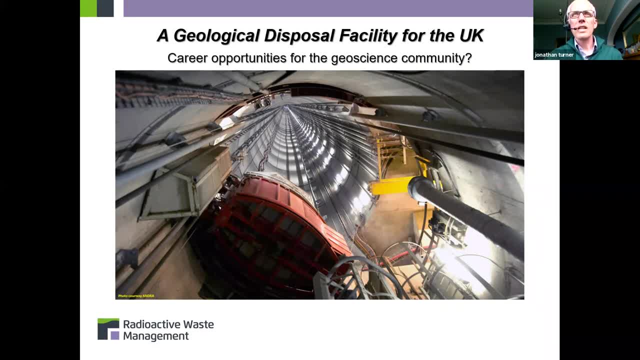 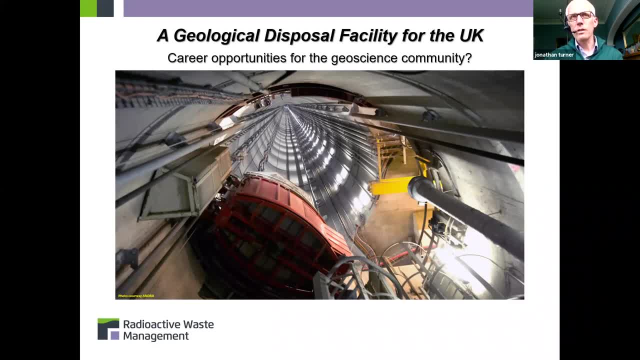 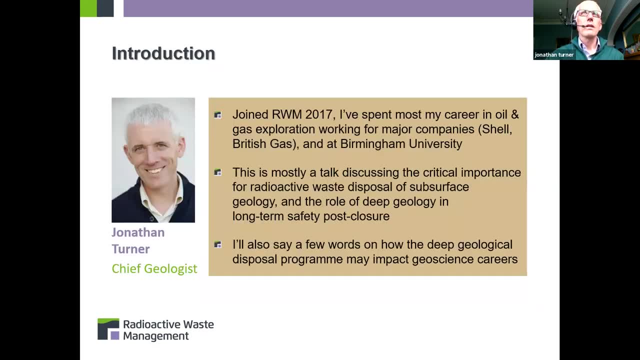 The The R well, and what hasn't gone well? so lots of interaction with overseas waste management organizations. there we go. uh, i think ray's really done my introduction. uh, for me, that's me, jonathan turner. i'm presently chief geologist for rwm, and most my career has been in oil and gas either. 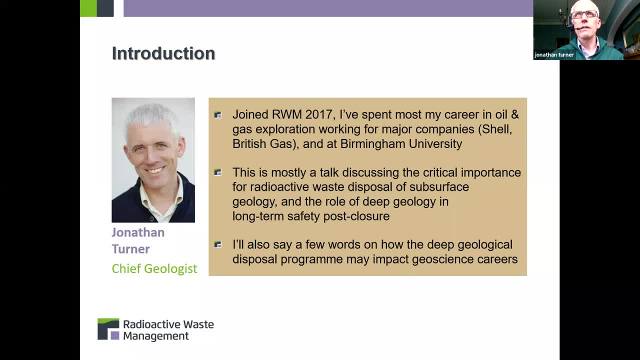 working for big plc's like shell and british gas and, as ray said, i spent about- actually about 15 years working at birmingham university. i'm going to be talking tonight about the deep geological disposal program and understanding, or helping you to understand, the critical role of geology and 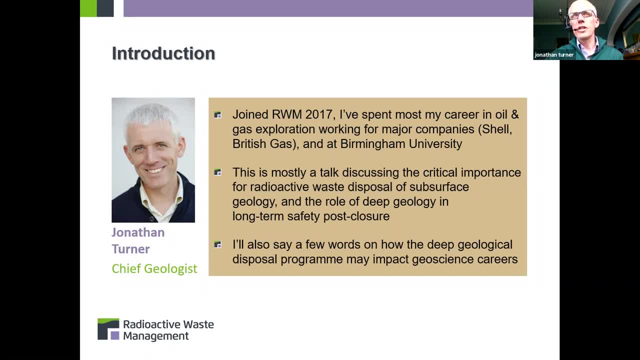 in ensuring the long-term safety of a gdf- and that's the acronym that i'll use- geological disposal facility, the long-term safety of a gdf after it's been completed, filled, decommissioned and effectively. we've walked away and and thrown away the key and then write it there and i'm just going to say a few words on how the deep geological 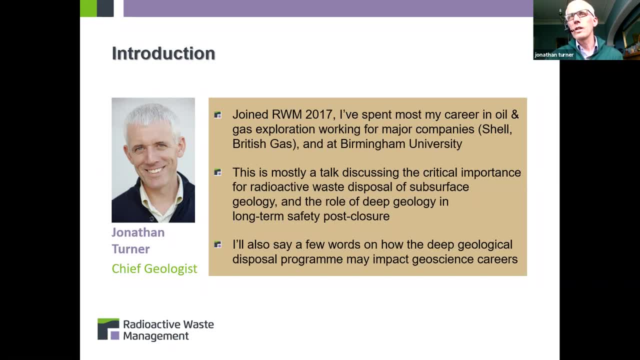 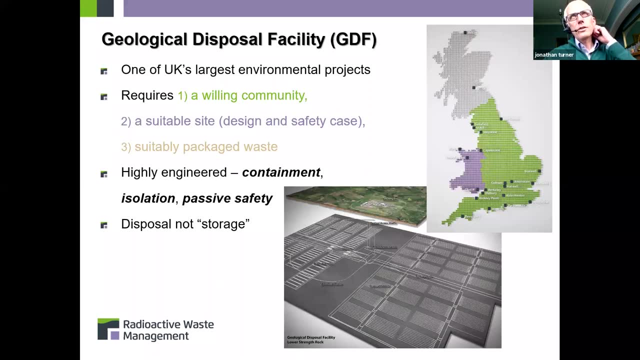 disposal program implicate its implications for geoscience careers. let's start with uh, with an introduction. i've said that i'll use the the acronym gdf. let's just start with the map up in the top right there. and in the days before the uh global pandemic, when we went to 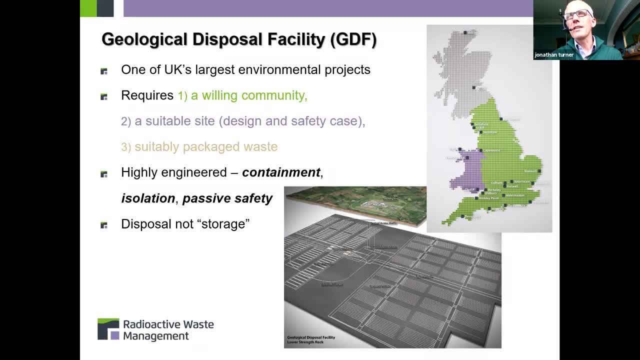 events like the big bang science fair at the nec and the new scientists live event at the excel center in east london. we had really nice display and one of the sort of graphics that we had that really surprised people was that map there which shows where the uk's 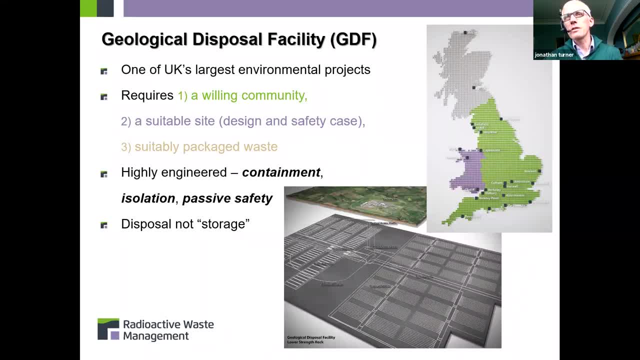 radioactive waste inventory is presently stored, because this talk is all about disposal. you know, i'm drawing a really a strong distinction between storage, which is a temporary solution, and deep geological disposal, which is a permanent solution. and you can see, i'm just going to be talking tonight about england and wales, but you can see that, okay, living where? 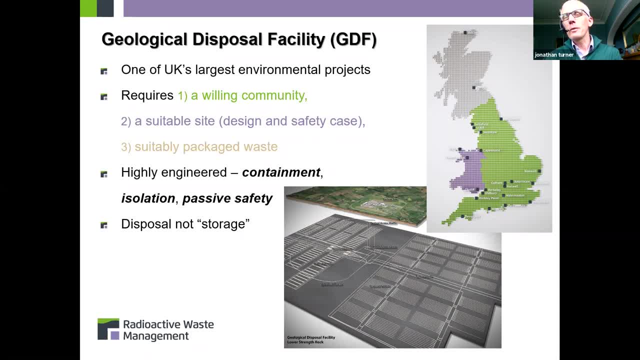 at least where i live in the in the west midlands is probably about as far as you can get from storage facilities, but there are plenty of places around the country where spent fuel and other types of nuclear waste are presently stored above ground, waiting for the time at which we have a facility in which that material can be safely disposed of. 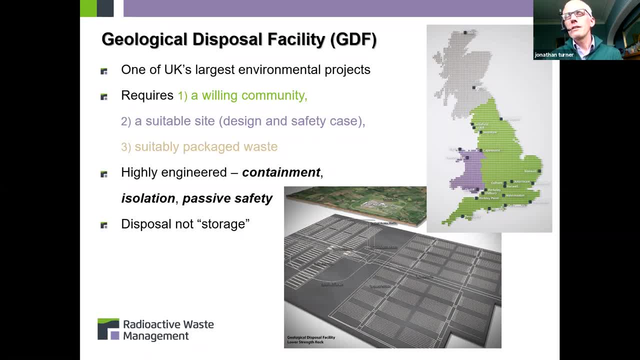 most of the waste is at sellafield and certainly if you took a straw poll of lay people sort of out in the street went down to the ball ring. most people have heard of sellafield and then they haven't heard of most of the other facilities that you see here. i think it certainly surprises people. 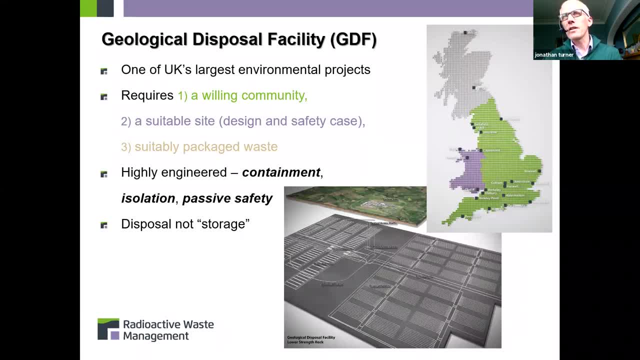 to see that there's about 25 sites, i think it is around the country. about 70 percent of the inventory is at sellafield, another 10 is at dune ray, hms falcon, on the far northern coast of scotland there, and then the uh. the rest is. 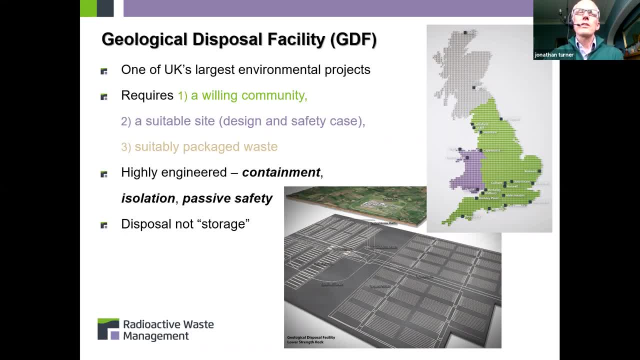 is distributed around the country. so i said right at the start of this talk that, um, i described this as being an environmental project and radioactive waste management is part of the nuclear decommissioning authority family of companies. but we consider ourselves to really be delivering an environmental solution to something that, uh, you know radioactive waste, which has been 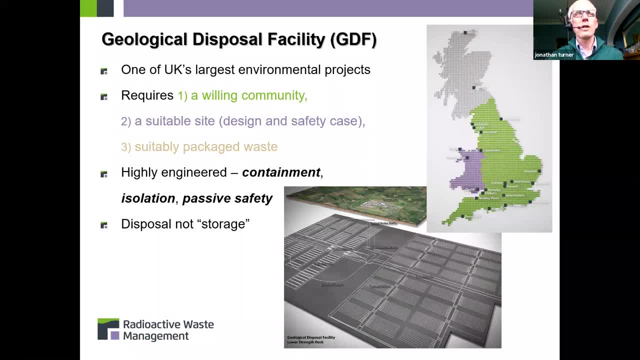 accumulating really for something like 70 years, right since the end of the second world war. the uk has been involved in the nuclear business- both the weapons program and also early development of commercial delivery of nuclear energy into the electricity grid- right since the outset, right since the advent of this technology. so 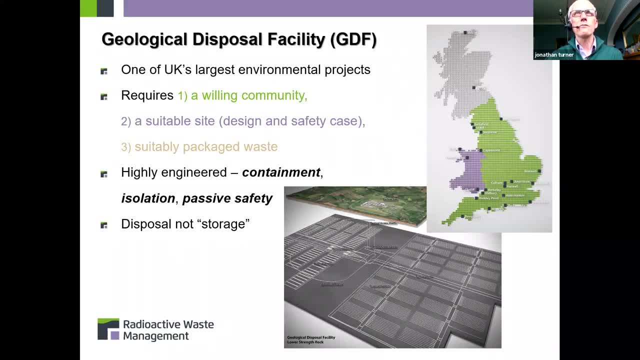 that's what gdf is about. it's about an environmentally responsible solution to disposing of this legacy waste, and there are three key ingredients that are required for us to be able to deliver a gdf. this is a consent-based process that's absolutely enshrined in government policy. 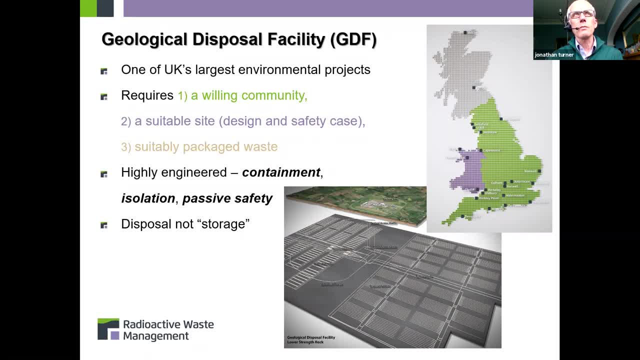 a gdf is not going to be foisted onto any community. this is about communities sticking up their hand, wanting to in the first place, wanting to find out more about what is entailed in terms of hosting a gdf within their area. so a willing community. 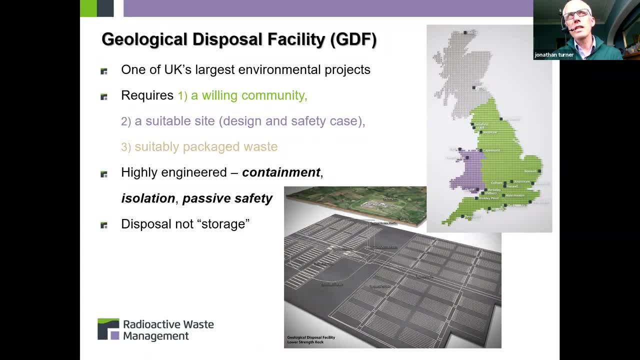 is the first key ingredient: a suitable site. what do i mean by that? i mean, not only is this a potentialJoey's point of view, but it's a great resource for everyone and it really can be used as a tool to help us to be able to deliver green energy to the. 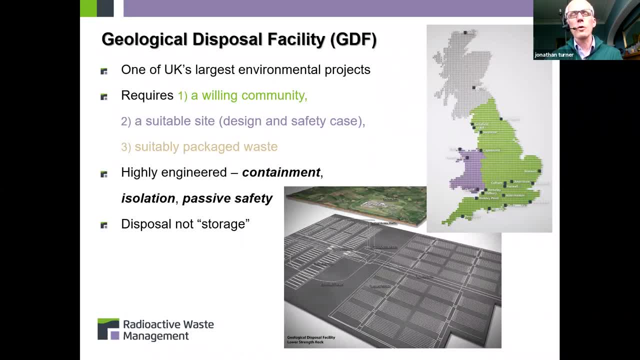 environment and the environment of the community. so i think that we can have that in our building, but then also it can be used as a resource to be able to deliver and maintain the sustainability of the棚ardly-cultivated waste and also uh to provide for our community as well. so as a resource. 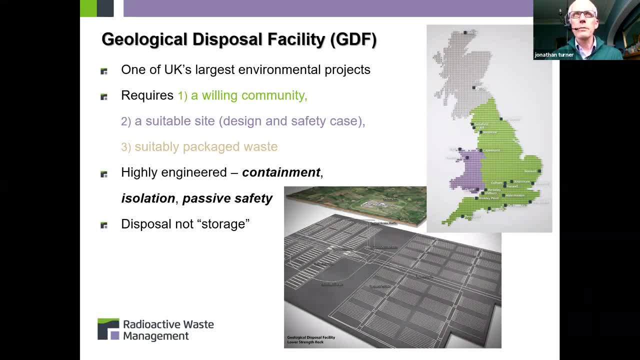 work with the rest of the nuclear decommissioning authority estate, in other words, the waste producers, the people who are right now packaging different types of radioactive waste. it's critical that we work with them such that, when the time comes for us to take their waste underground and 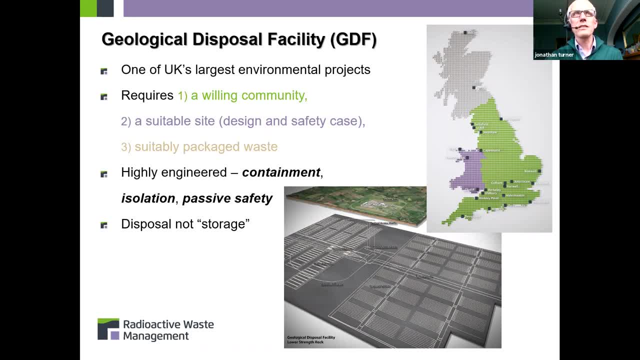 dispose of it. we understand that their waste is suitably packaged such that it can work with the engineered barrier and what we call the multi-barrier- and I'll talk more about that a little bit later- in other words, that that suitably packaged waste is safe to be disposed of in the GDF. I've talked. 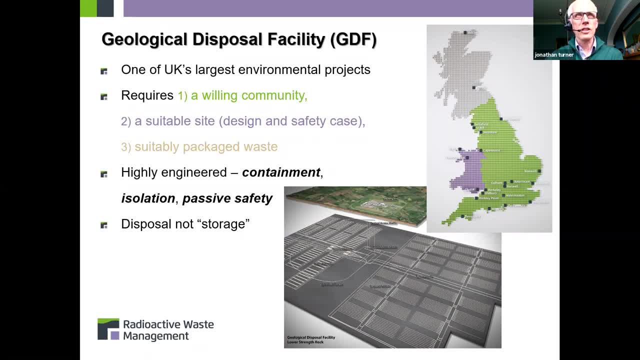 about disposal, not storage, and drawn a strong distinction between those two there. and then for me there's three sort of by words that I associate with a GDF. I mean it could be in a whole variety of different geologies, it could be onshore, it could be offshore, it could be between 200 and 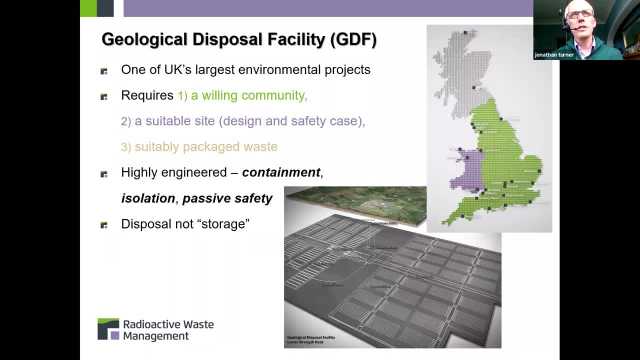 1000. meters depth. so until we have a willing community, we necessarily have to keep our options open. but however the GDF ends up looking, it will need to satisfy these three or two key requirements really. firstly is containment, and what I mean by that is an ability to contain radionuclides such that they 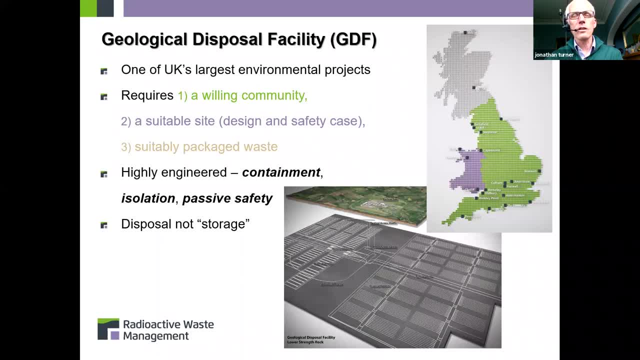 can't migrate to the surface or into the near surface environment where they could harm people and the environment. and secondly is isolation: Isolation both from future generations and even future civilizations, possibly inadvertently mining or drilling into the GDF, and also isolation from surface processes like 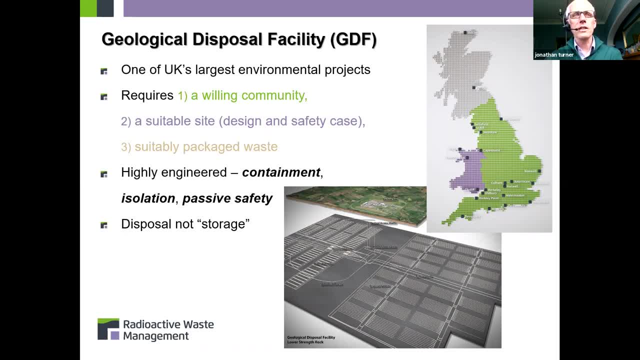 glaciations and earthquakes, and I'm going to say a lot more about that just a little bit later in the talk. The third point, the third word set of words, that's in bold. there is passive safety, and this is just to make the point. I've already mentioned that there are a number of different. 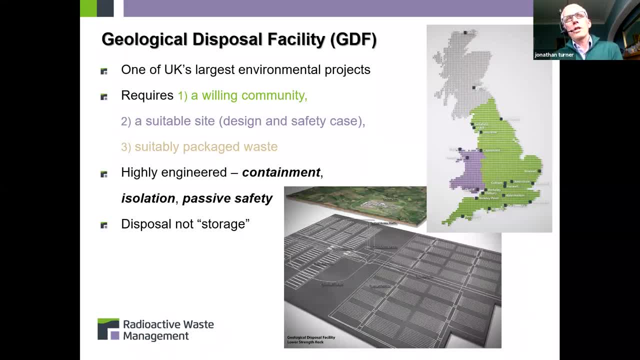 ways in which the GDF can be used to contain radionuclides. The first one is to be able to monitor the length of the what we call the post-closure safety case, in other words, the post-closure period of time over which we will need to demonstrate to regulators. 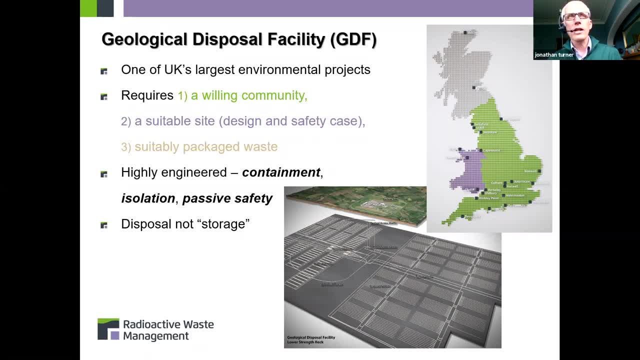 that the GDF can safely contain those radionuclides is of the order of hundreds of thousands of years, up to a million years. now there's no technology, there's no monitoring technology that can be put in place that can obviously run for that kind of period of time. 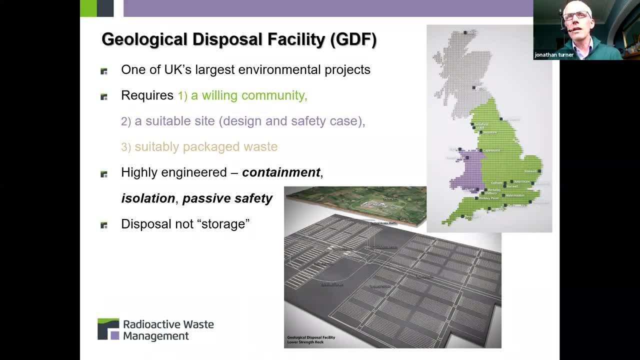 and therefore the assumption is that the GDF won't need monitoring. the assumption is that it will be so well engineered. it will need to be so well engineered that once we have backfilled it and decommissioned it and remediated the surface site, then it won't need any further monitoring. 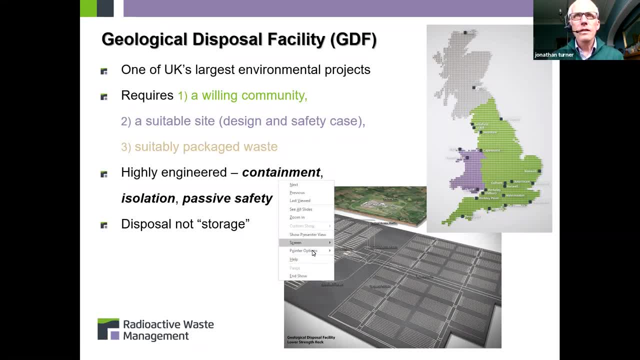 If I just get the pointer up, that's great. okay, so the sort of cutaway perspective view that I'm just pointing out with the pointer here just gives you a feel for how a GDF could look. and do bear in mind that until we have a, you know that that first key ingredient, the willing community, the whole, 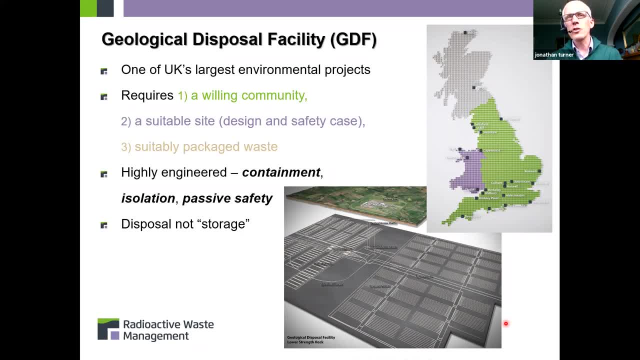 variety of different configurations that it could take on, not just dependent on geology but where it is. could be offshore, could be off the coast, could be beneath the land. but this just gives you a feel for what it might look like. I'll say a little bit more about surface site in the mid in a minute up. 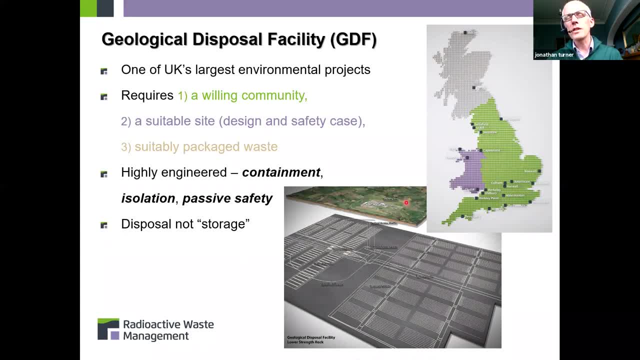 to two square kilometers, But we could make do with one square kilometer, almost certainly served by a rail head, although if it was on the coast it might also be served by port facilities where some of the waste could be transported in, and access to the GDF underground might be via vertical shafts or a drift this sort. 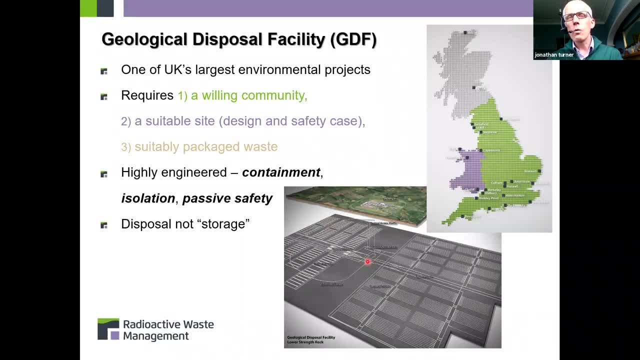 of ramp that you can see winding down here, one of the two of those, or possibly both of those, we don't know. once again, you know, I emphasize that the need to keep options open until we have a community, until we're working with a community, until we're able to converge on a 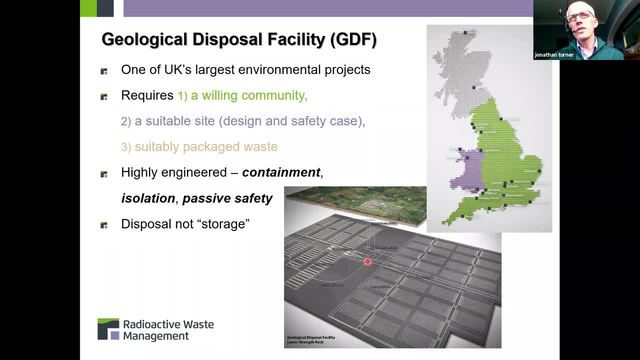 solution based on real site-specific information: the footprint of the layout, the footprint, the GDF itself. about 20 square kilometers and you can see it divided into two halves here. so the larger half half on the right is the volumetrically smaller portion of what we call high heat generating waste. 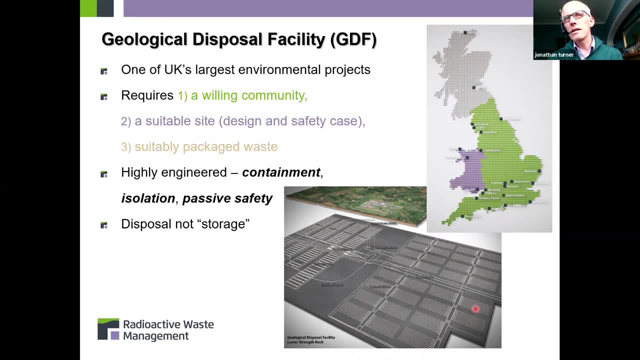 and I'll talk a little bit more about this in the next slide. It occupies only about 20 percent of the volume of the inventory, but the larger part of the footprint of the GDF because it generates heat. it needs to be spaced more widely in order to allow the geology to wick away the heat. 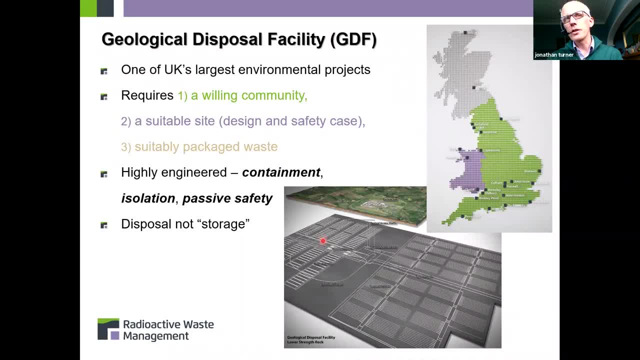 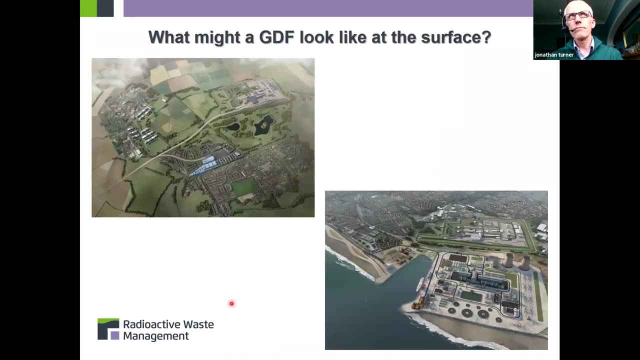 and then, on the left hand side, the volumetrically dominant proportion of the total inventory, which is what we sort of group into what we call intermediate level waste, ie non-heat generating waste, which can therefore be spaced a lot more closely. Okay, so I said I'd just give you a feel. 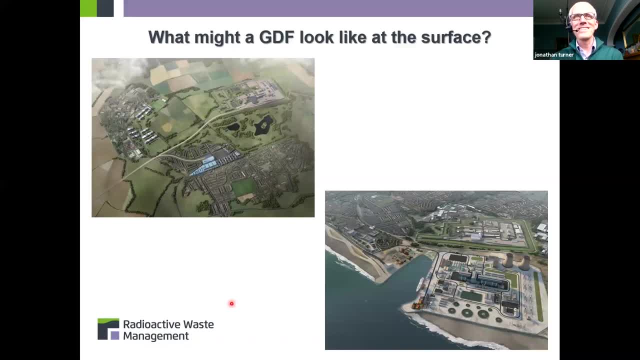 and again, clearly, these are- these are artists, impressions, cartoons, if you like- for what the GDF might look like at the surface. it could be inland or it could be on the coast, it could be possibly as shown here. Here's the the GDF surface facilities and it's shown next to a reactor, here up to two square. 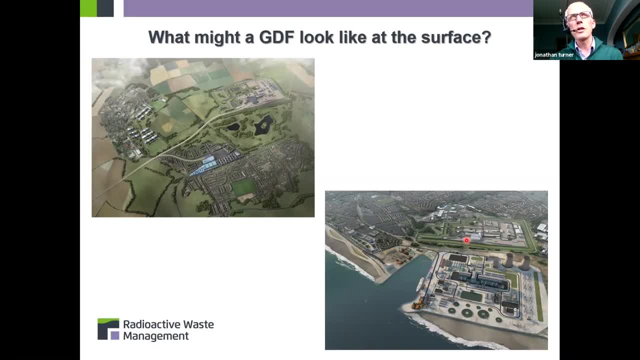 kilometers doesn't need to be that big. I think we would be pushed to go at less than a square kilometer. so about the size and complexity of the facilities that you see at the entrance to the channel tunnel down in Ashford and, of course, after, the GDF itself will operate for something? 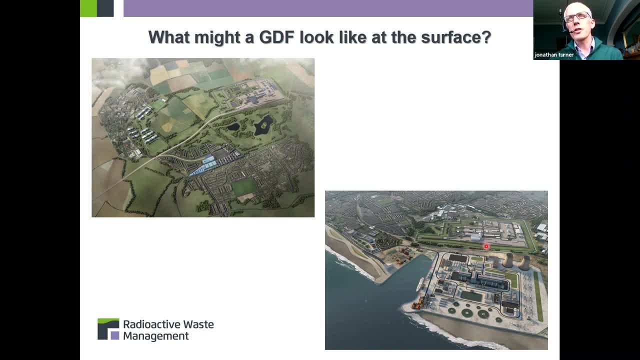 like a hundred years, And after it's been decommissioned, then all of these facilities will be removed and it will be remediated, much as is happening with the Winfrith experimental reactor down in Dorset near the Jurassic coast, which is being returned to the sort of original heathland landscape there. 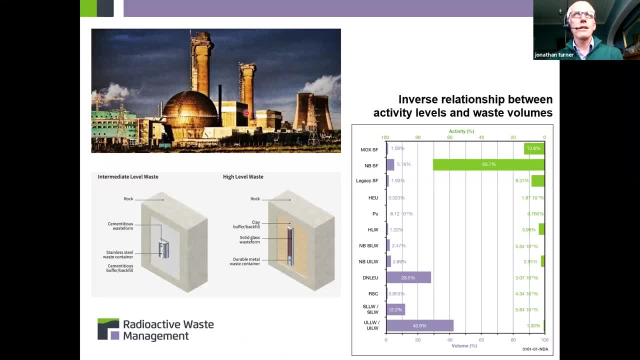 Okay, well, I talked about Sellafield already and no apologies for showing a photo there of Sellafield on a particularly foreboding site. Now, if you look at the background of the building in the foreground you can see the two towers. here are plutonium stacks. 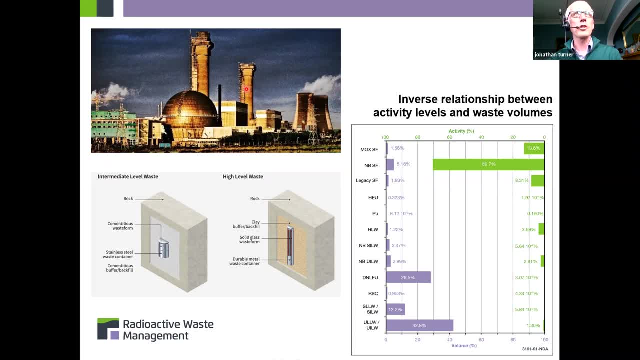 I think both of them- certainly one of them, possibly both of them- have been demolished now. One of these was the source of the 1957 fire. In the foreground you can see one of the earliest experimental gas cooled advanced gas cooled reactors, and then on the right here steaming away. you can tell that this picture is fairly old. 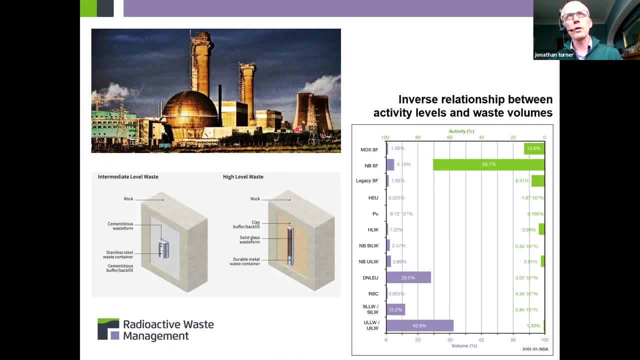 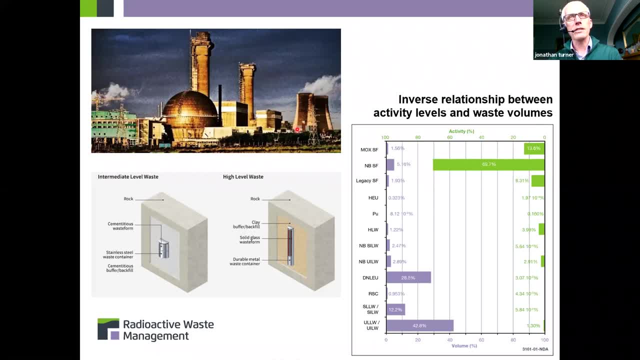 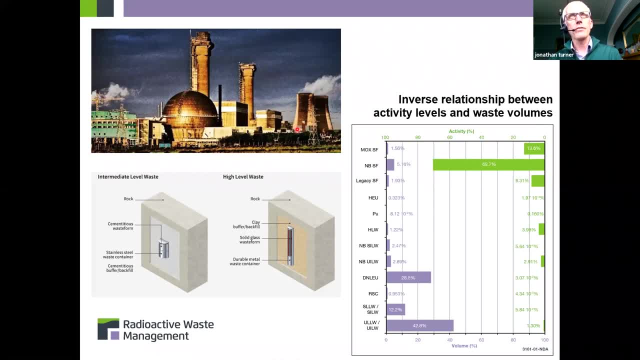 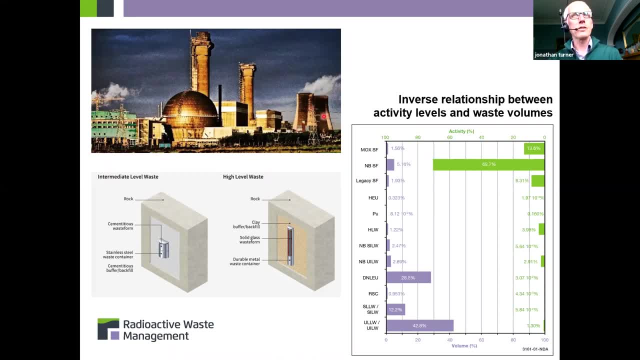 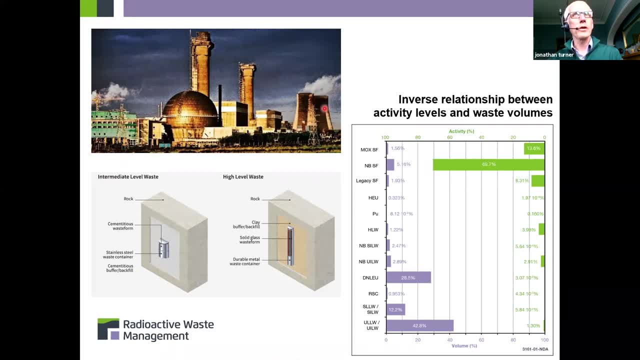 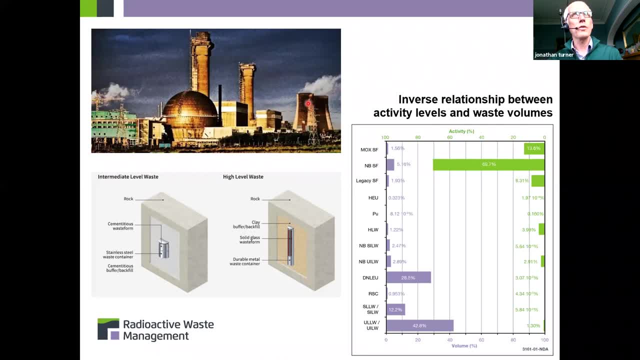 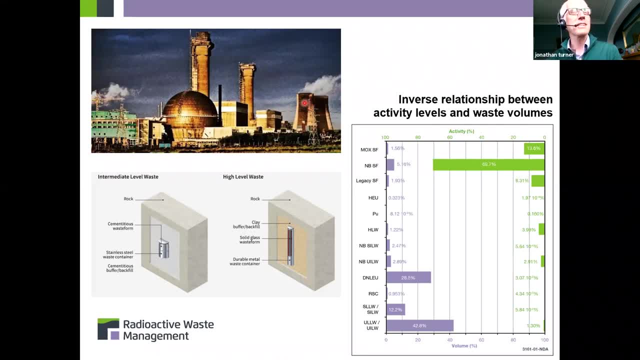 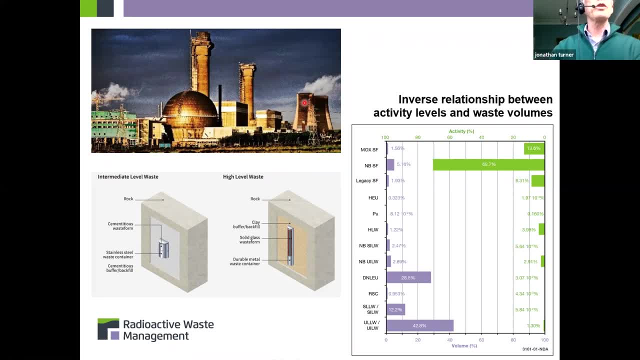 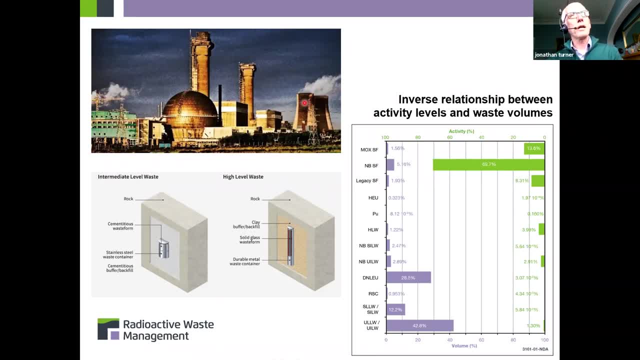 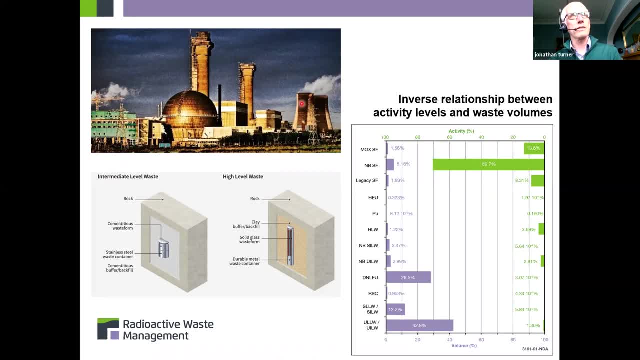 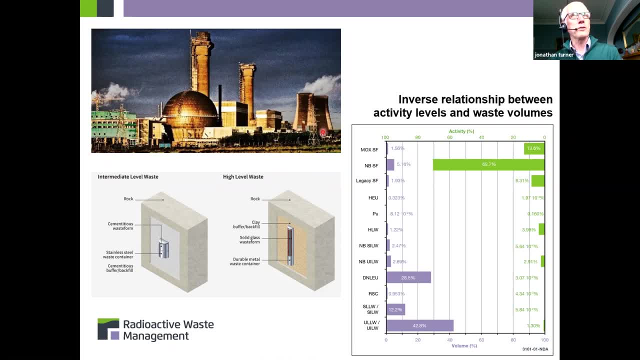 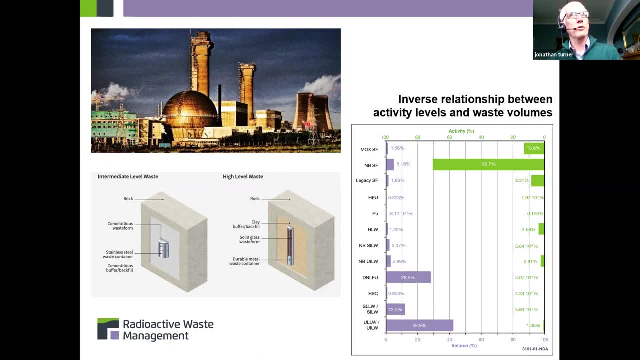 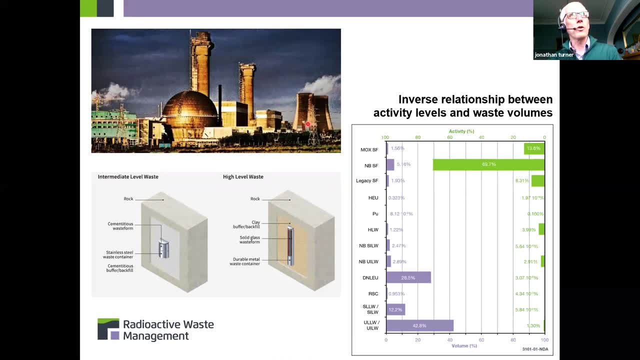 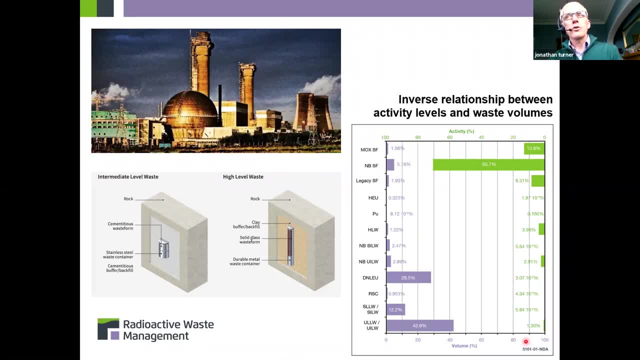 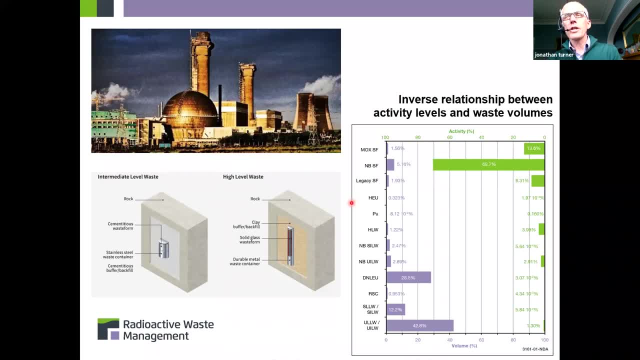 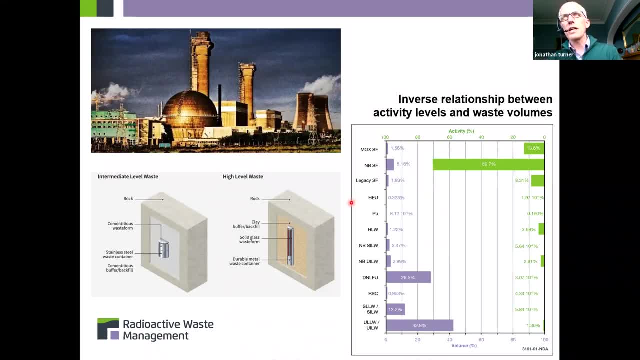 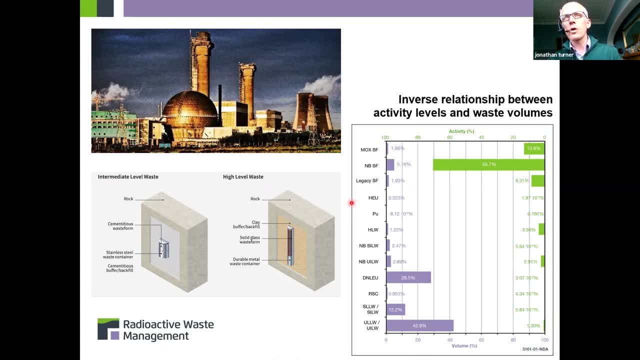 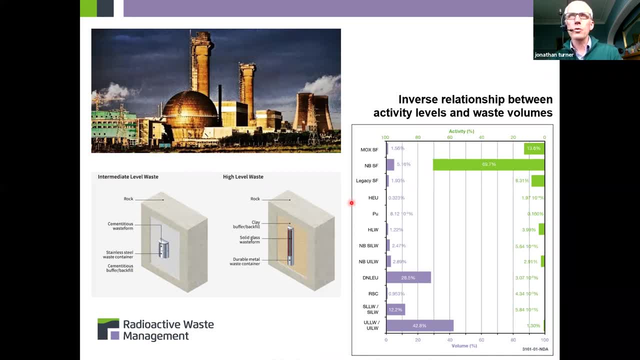 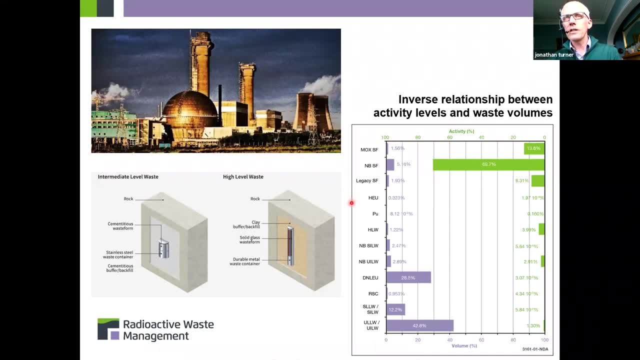 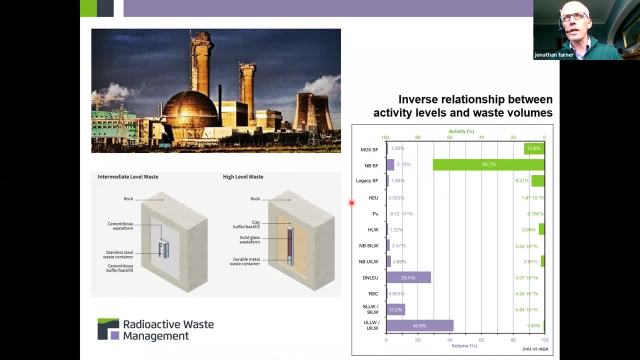 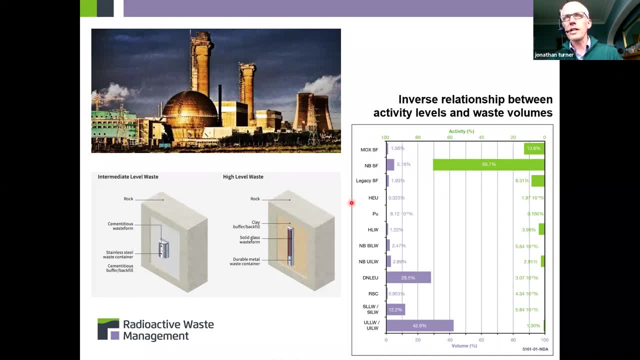 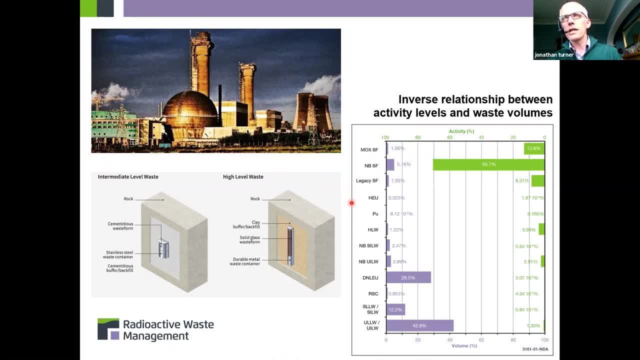 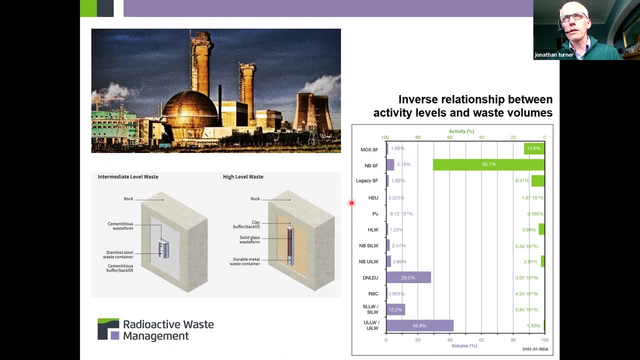 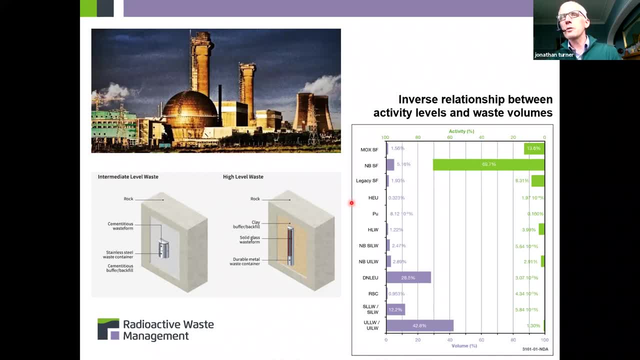 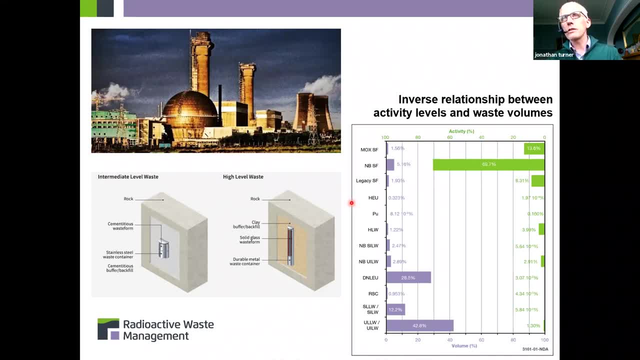 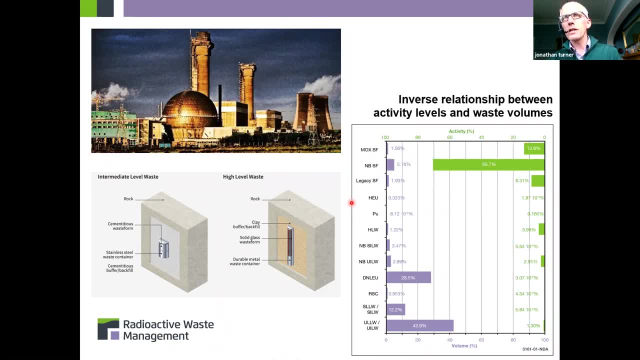 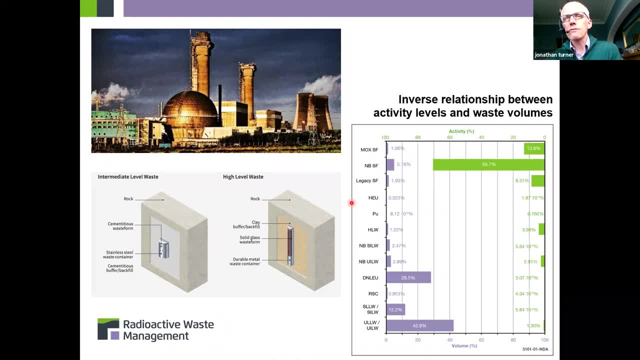 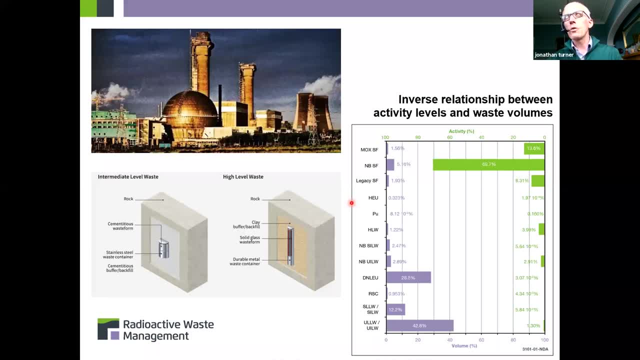 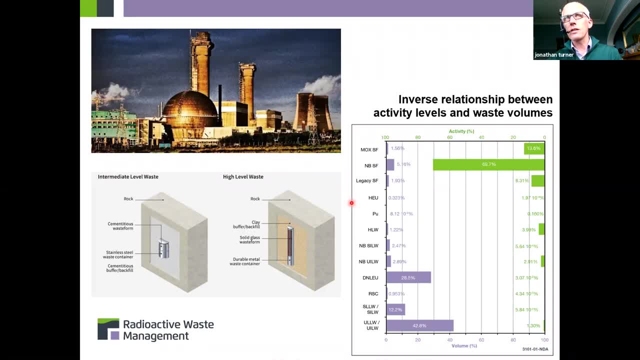 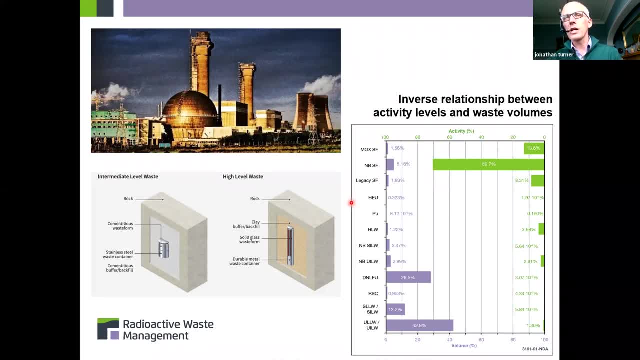 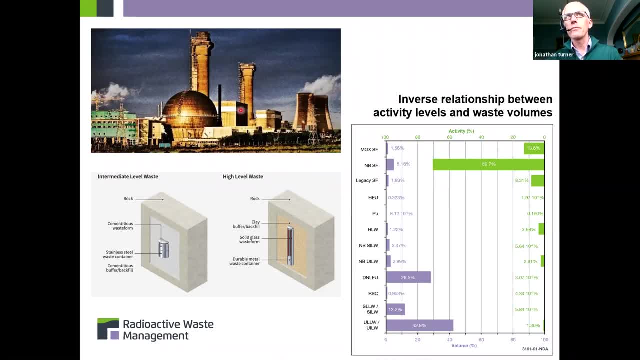 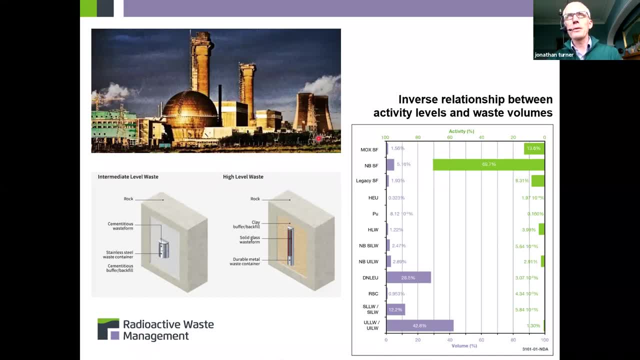 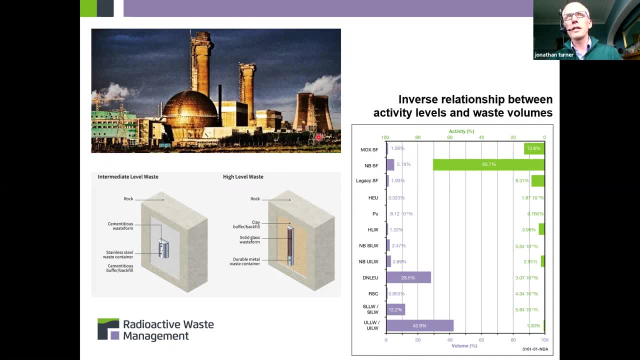 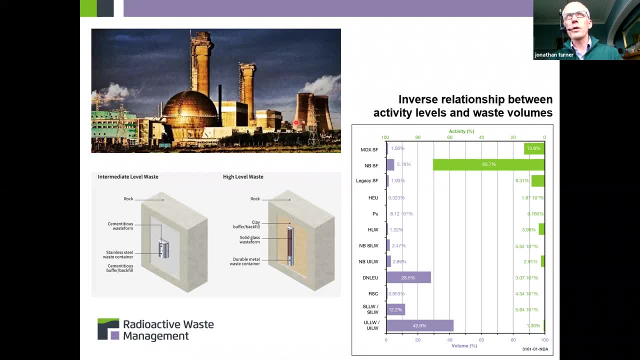 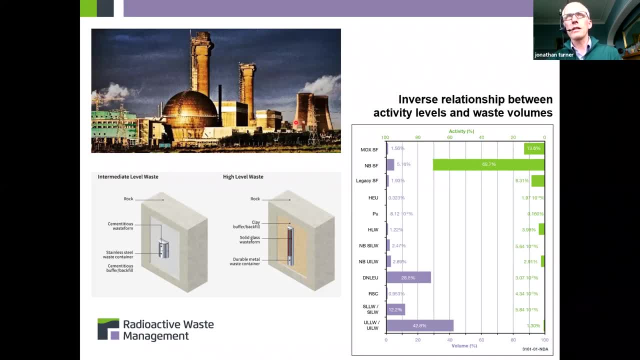 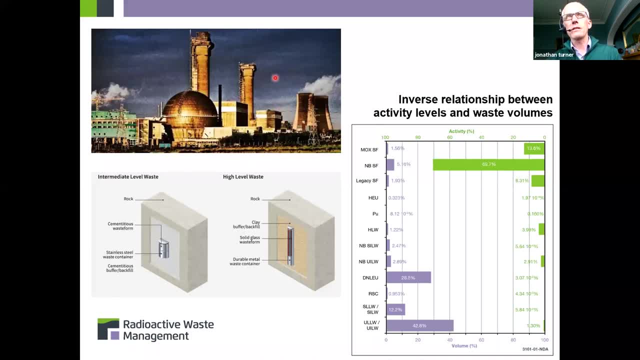 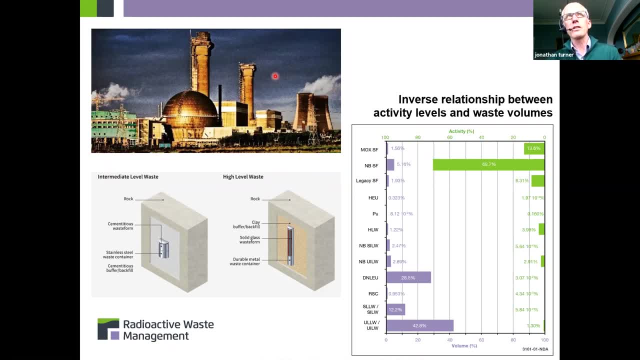 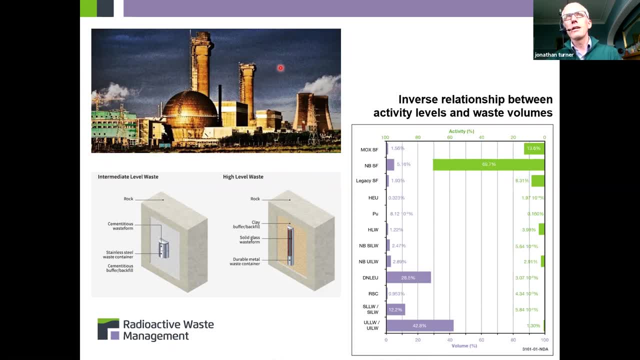 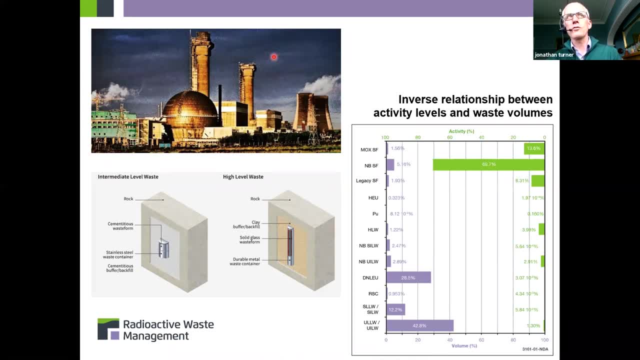 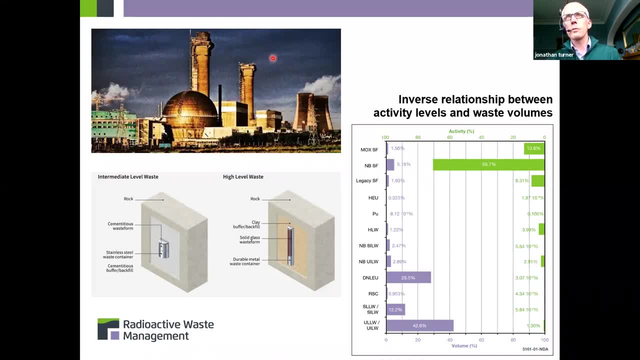 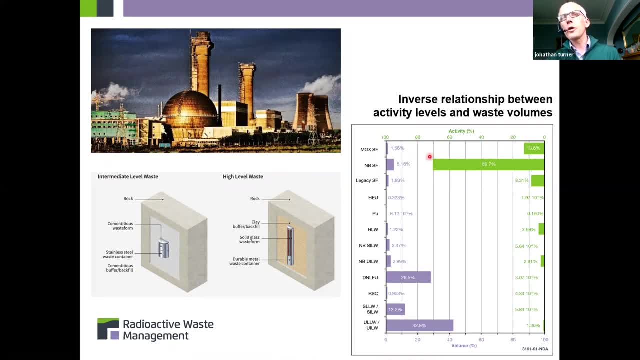 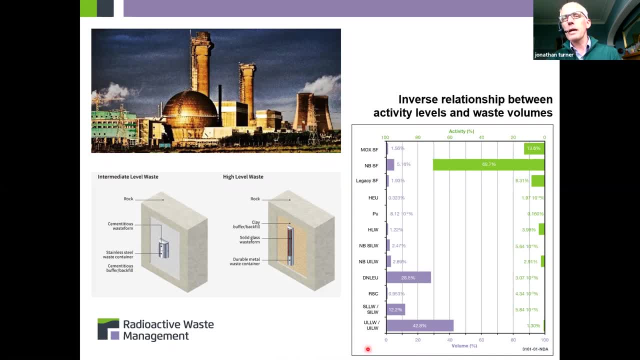 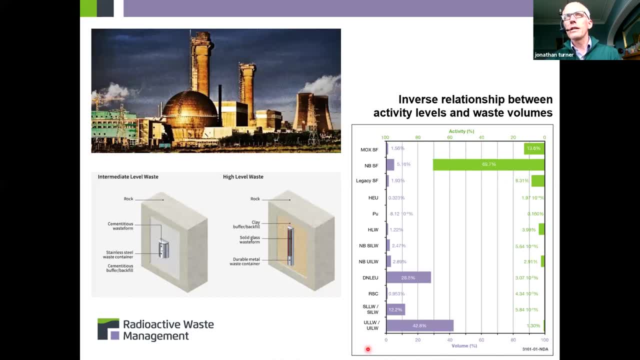 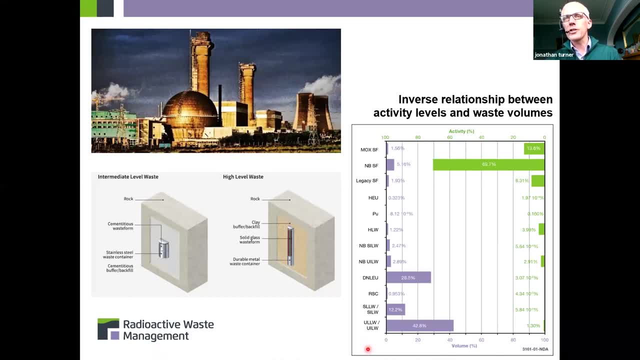 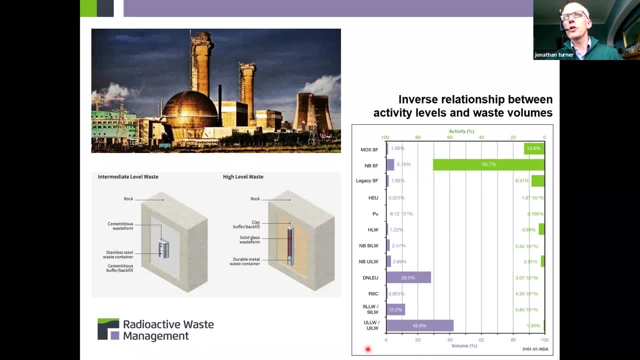 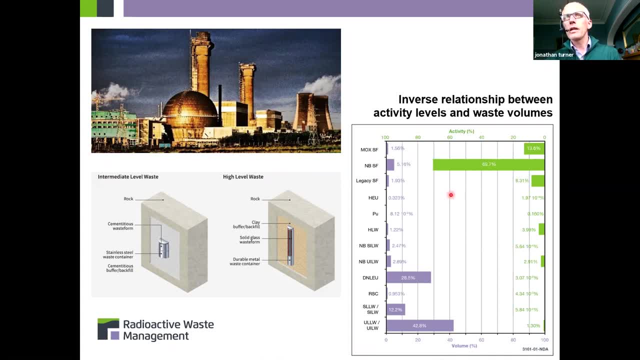 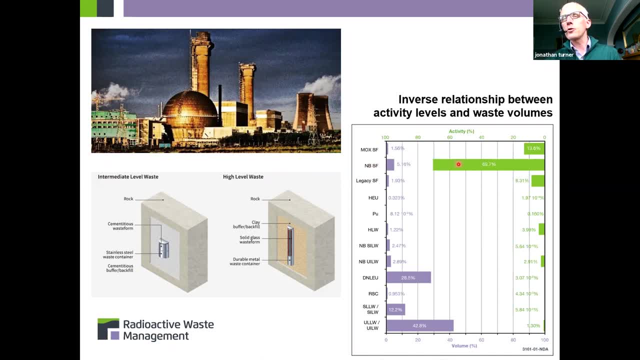 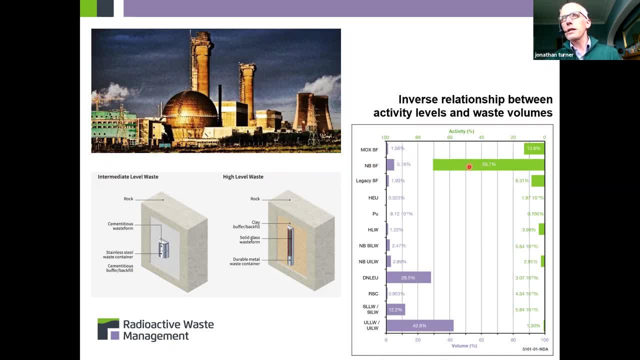 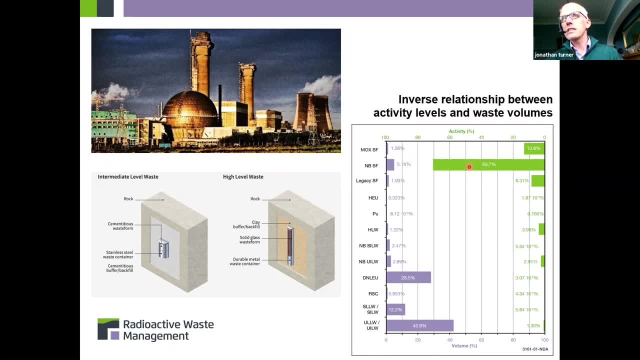 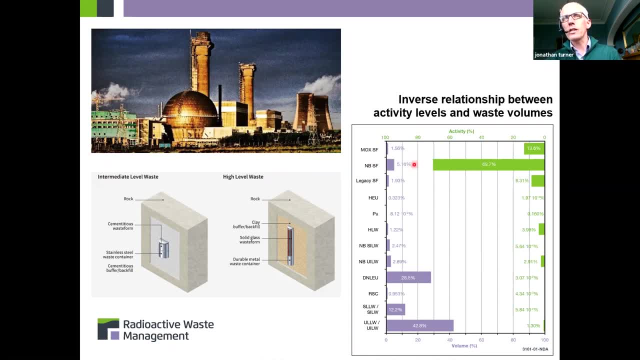 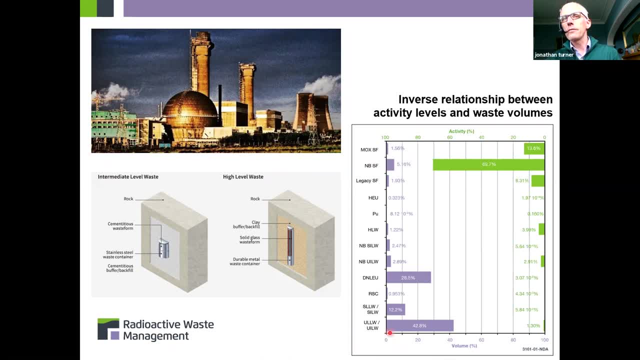 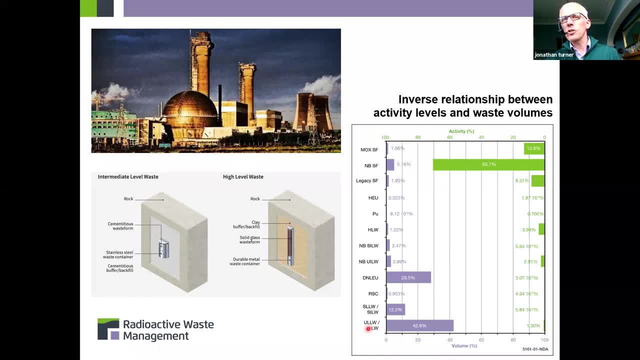 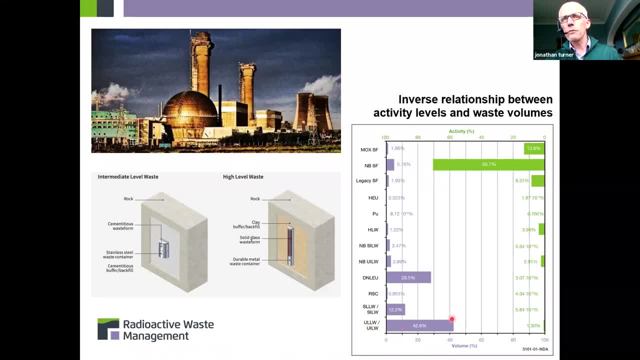 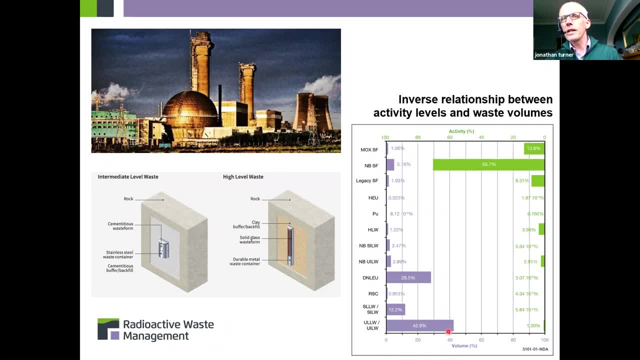 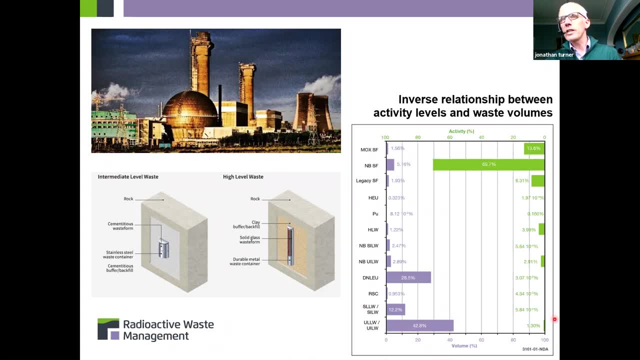 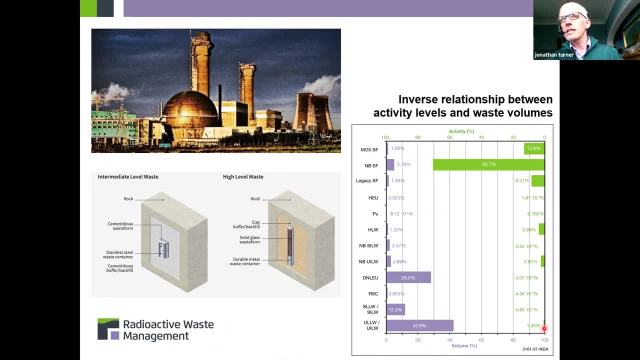 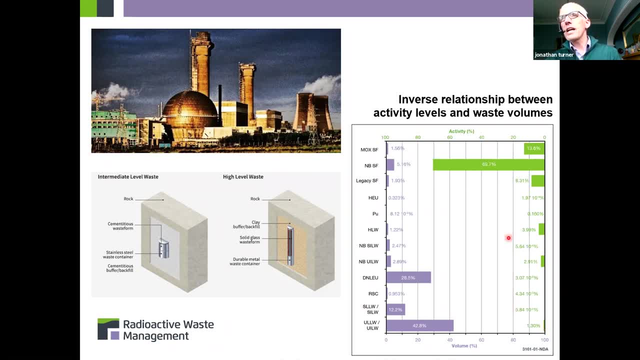 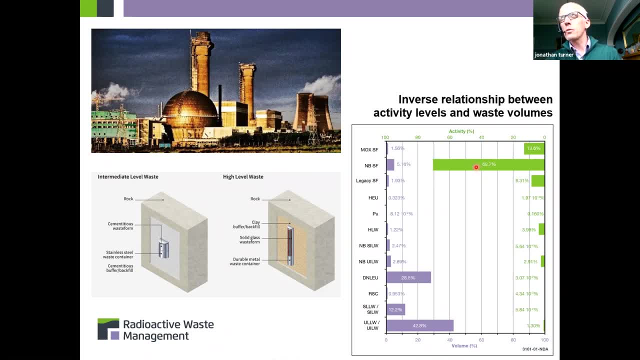 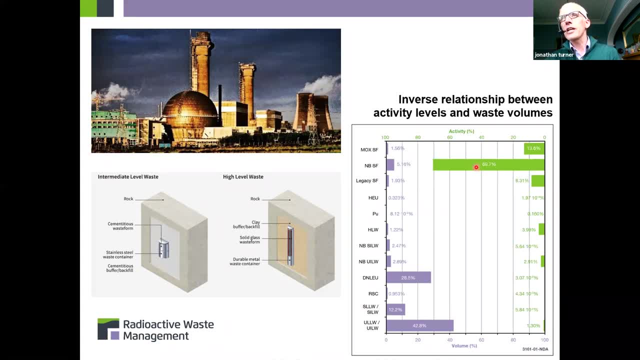 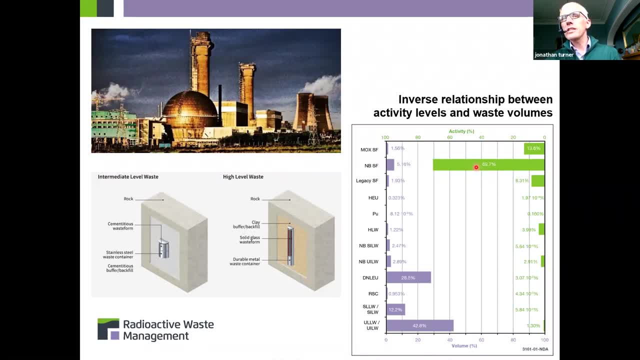 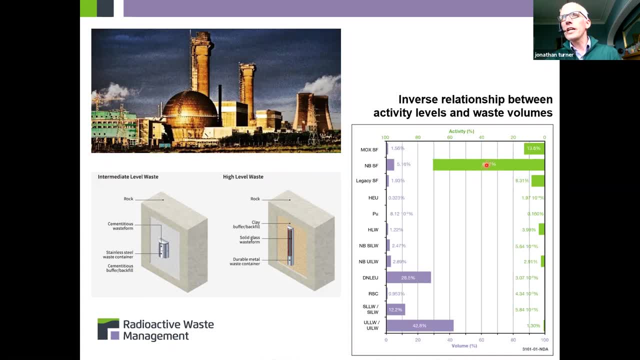 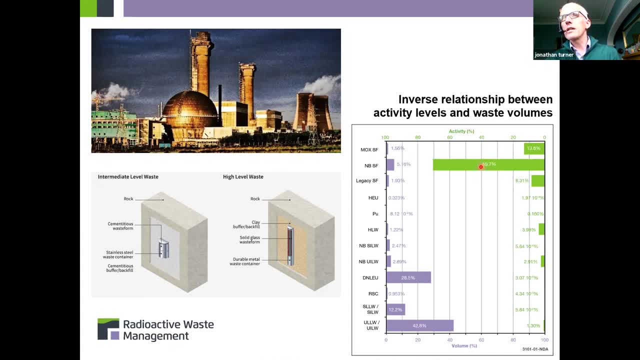 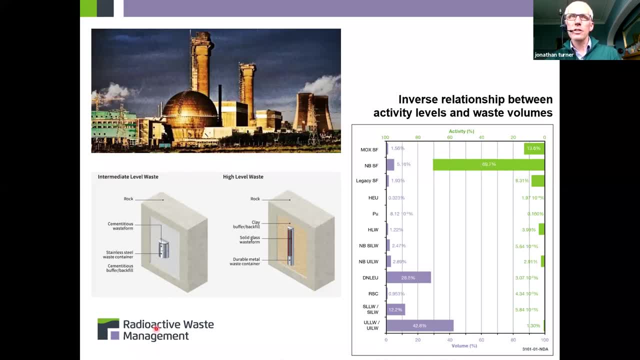 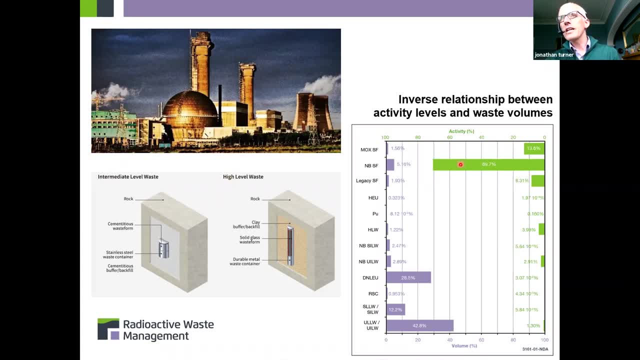 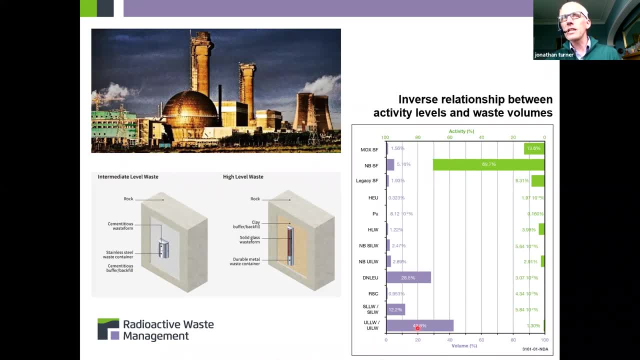 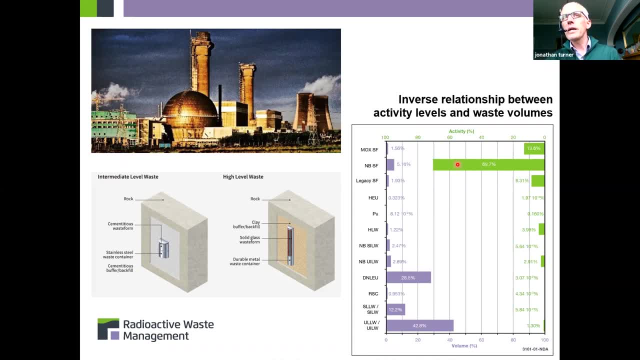 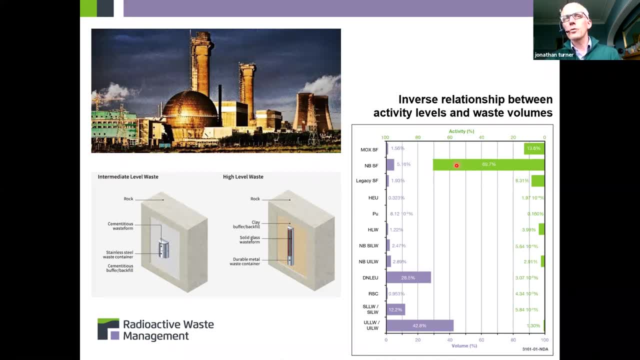 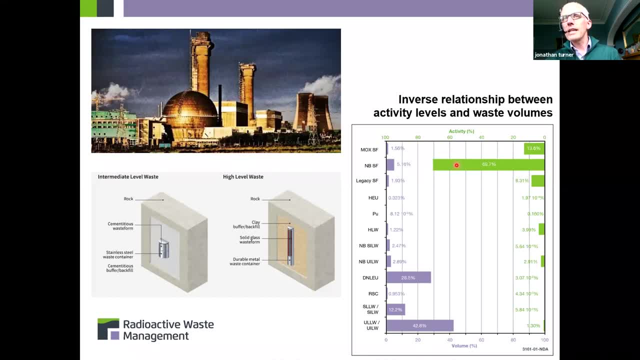 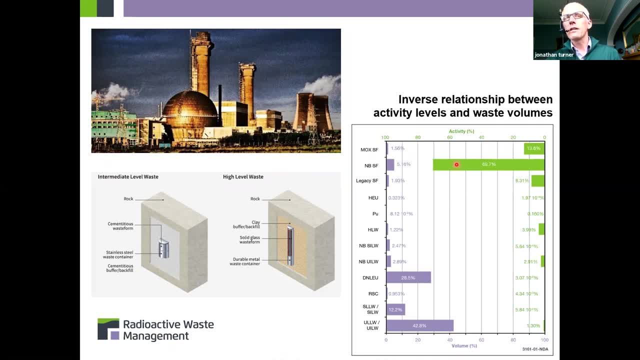 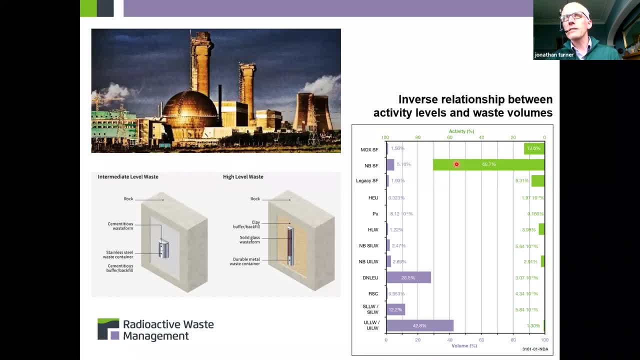 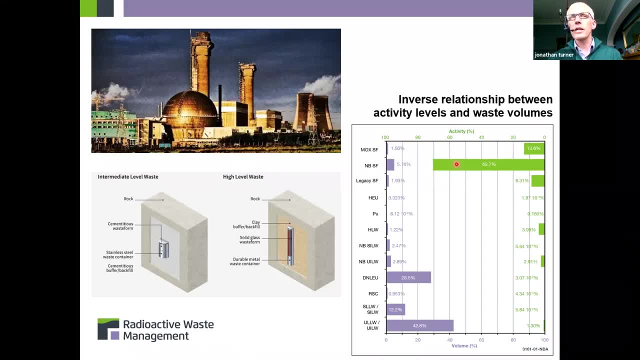 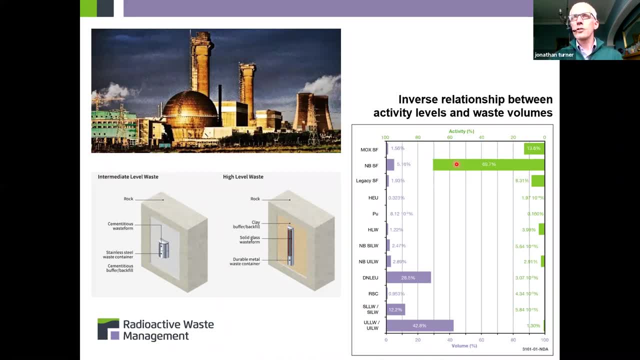 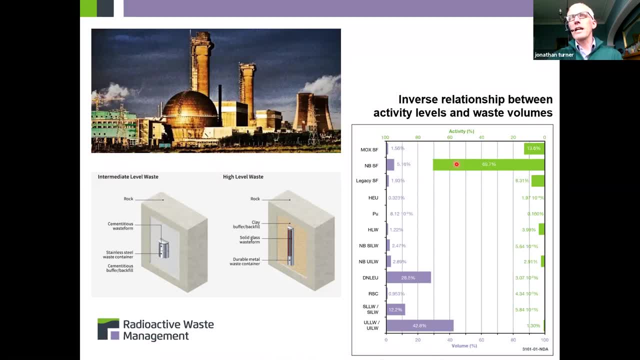 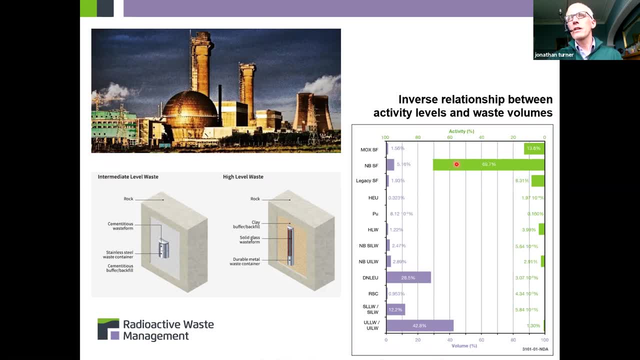 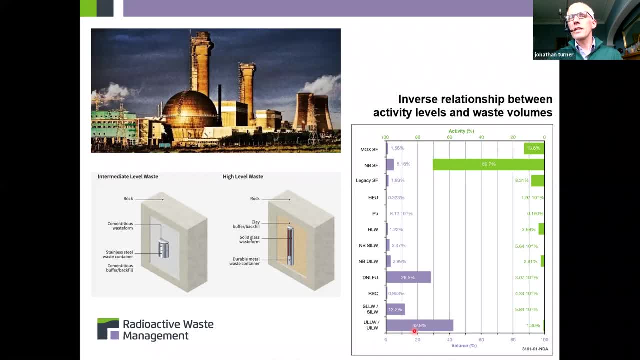 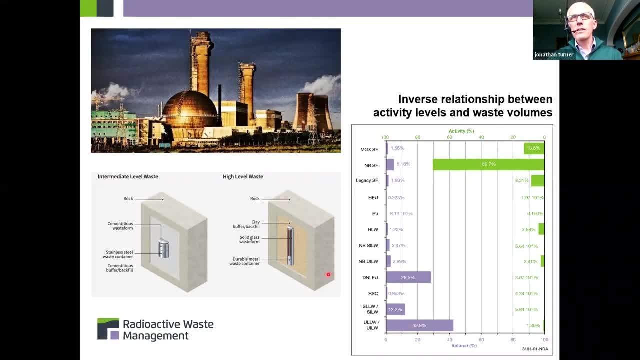 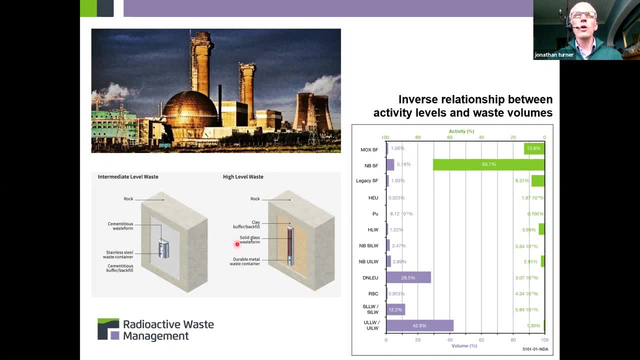 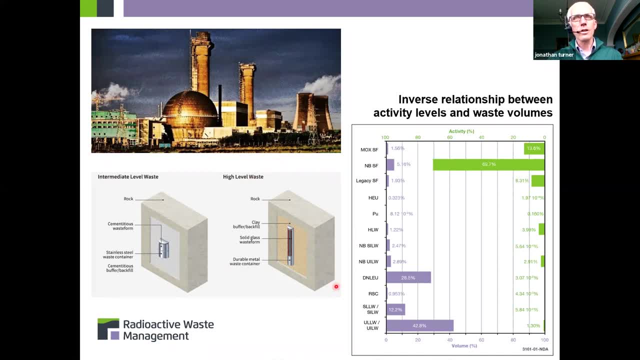 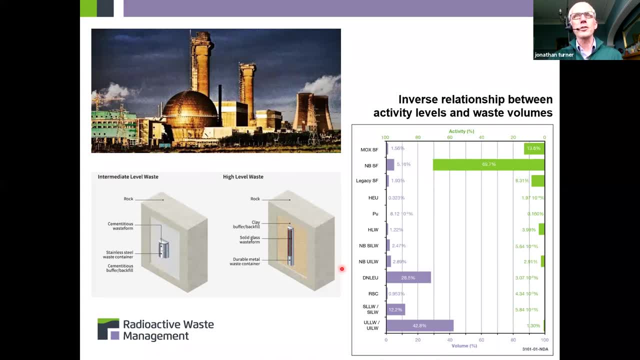 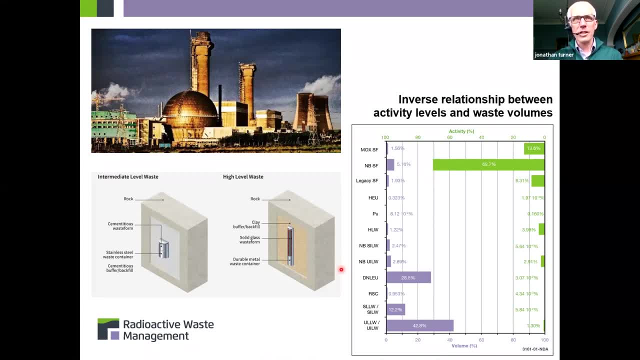 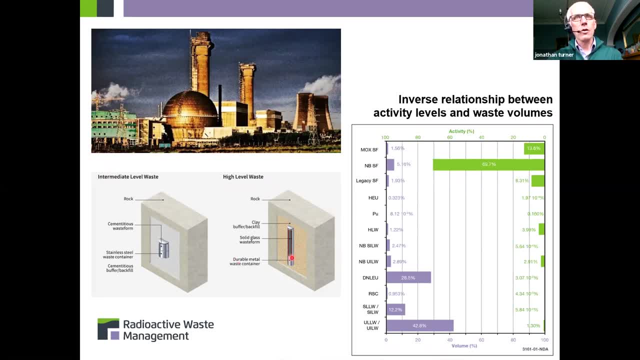 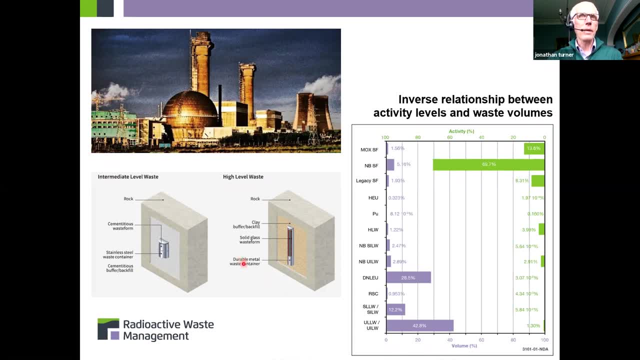 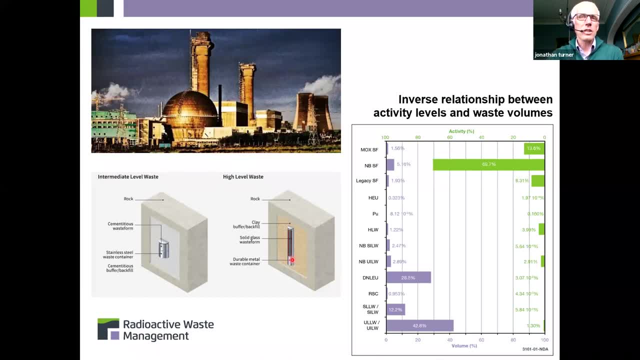 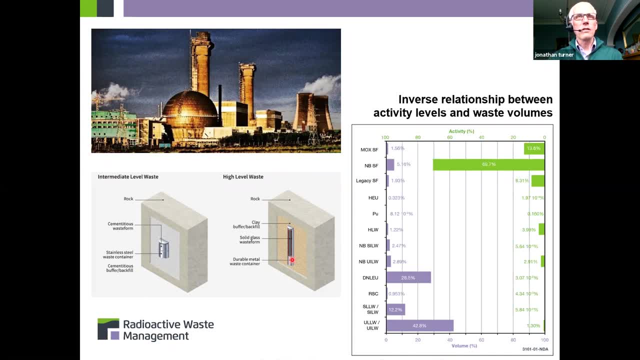 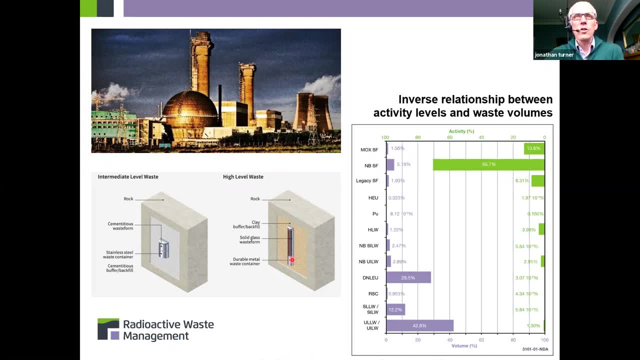 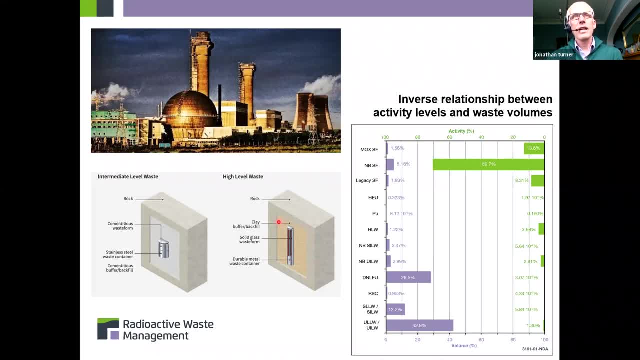 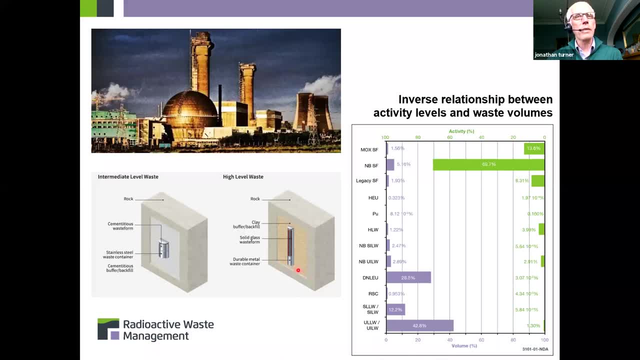 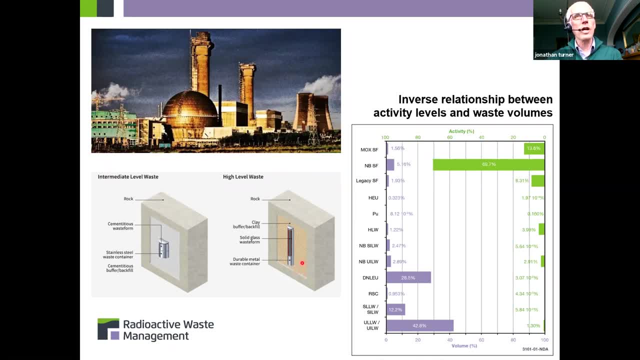 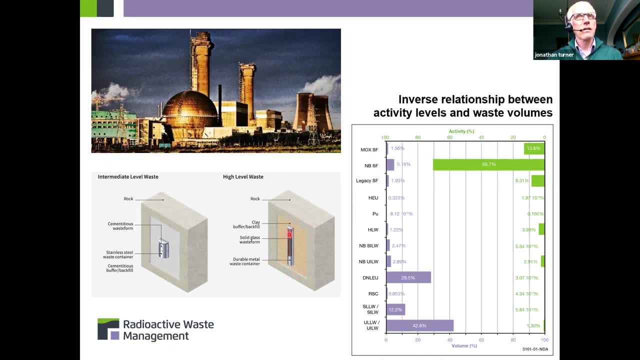 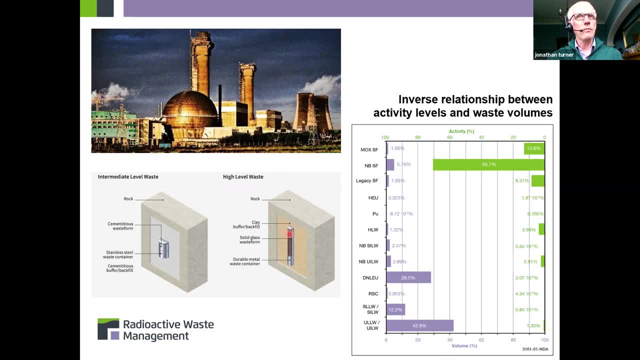 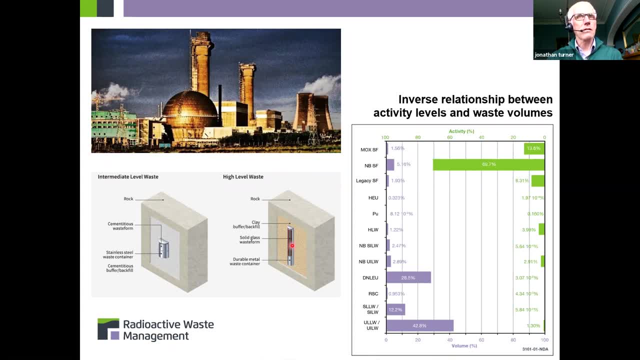 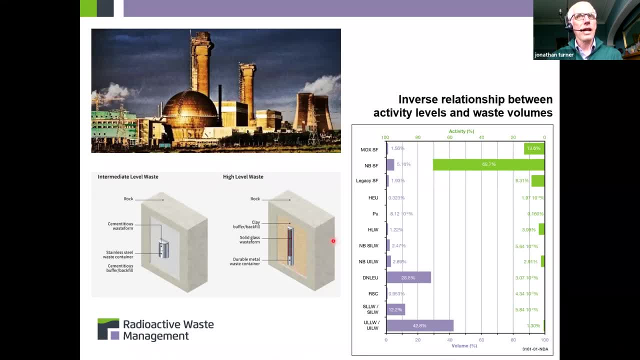 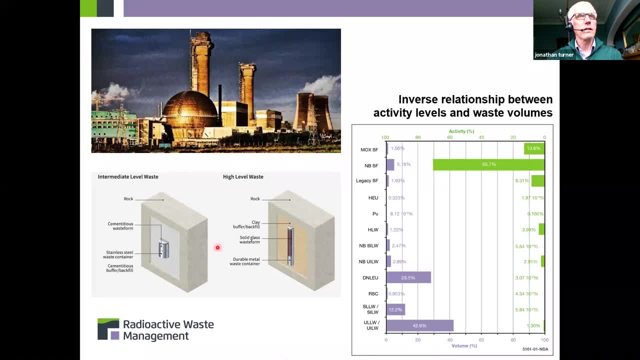 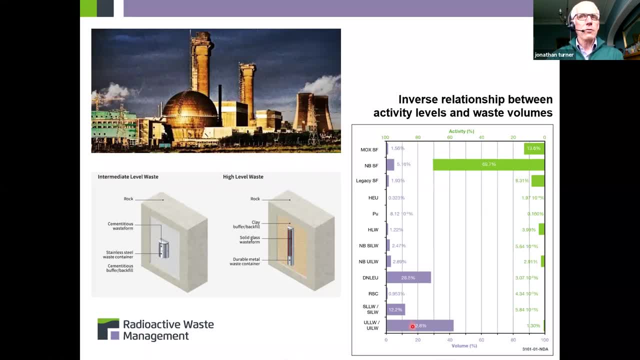 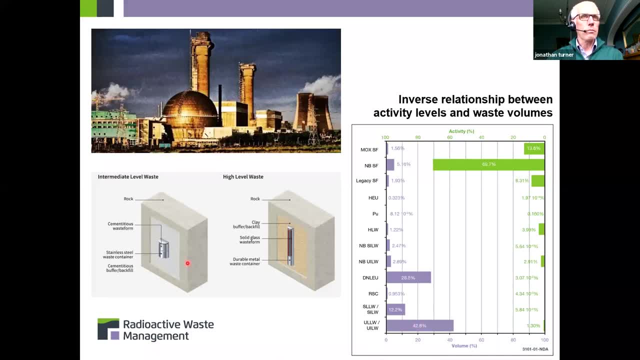 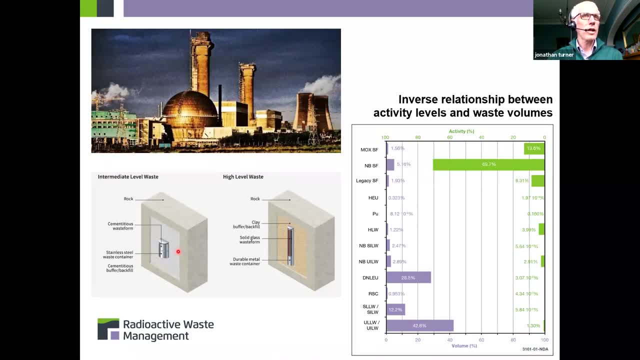 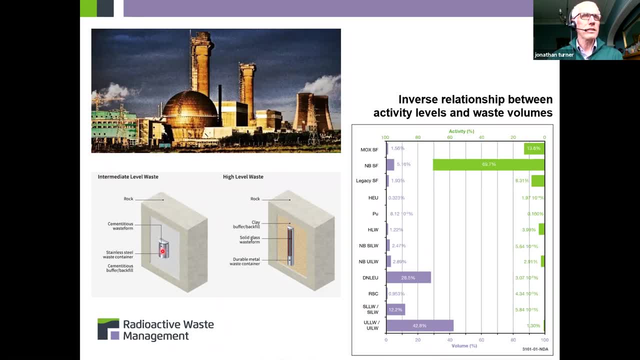 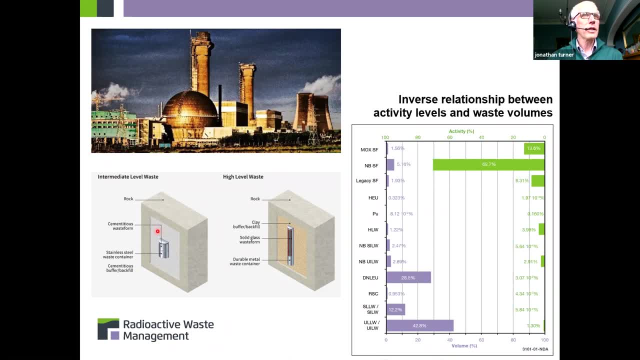 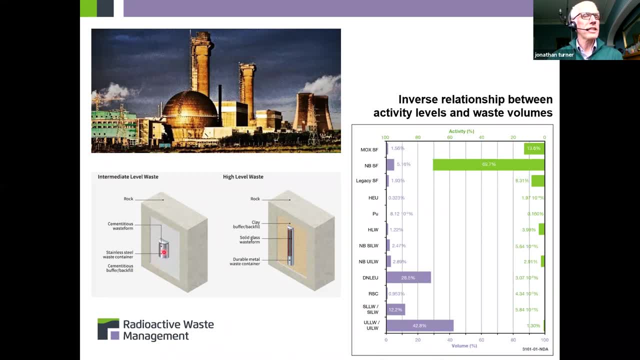 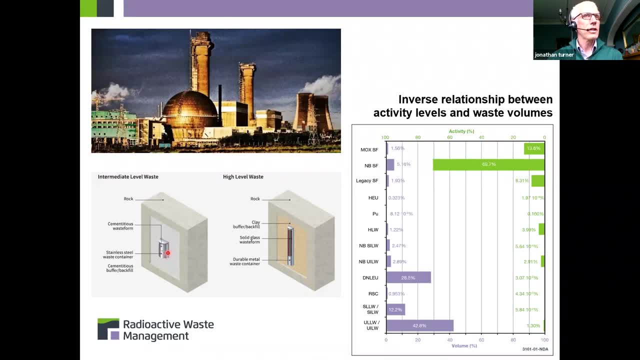 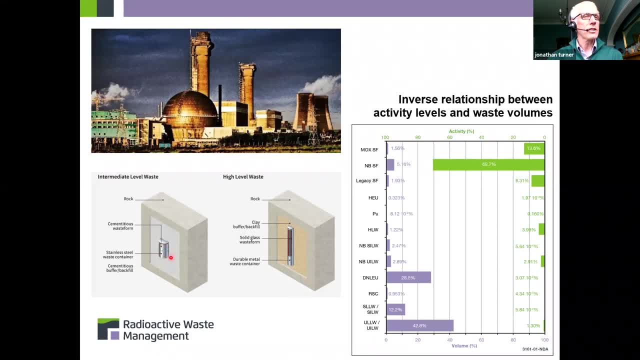 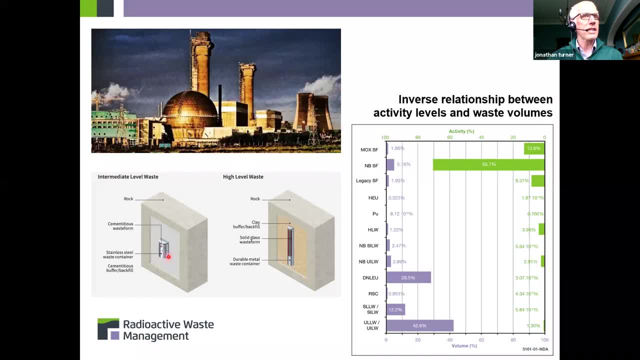 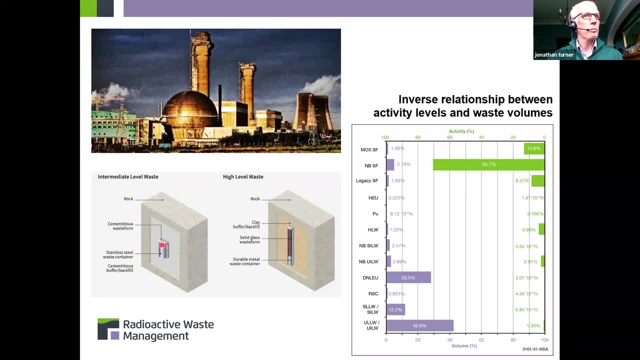 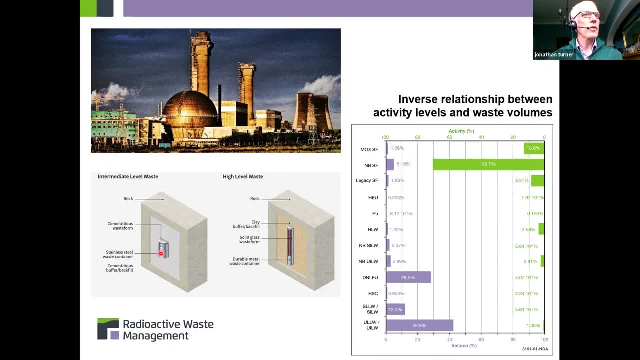 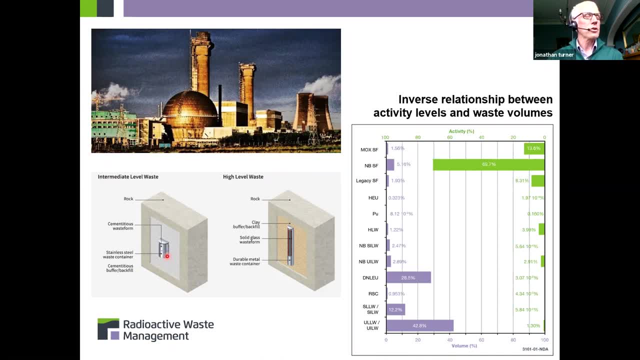 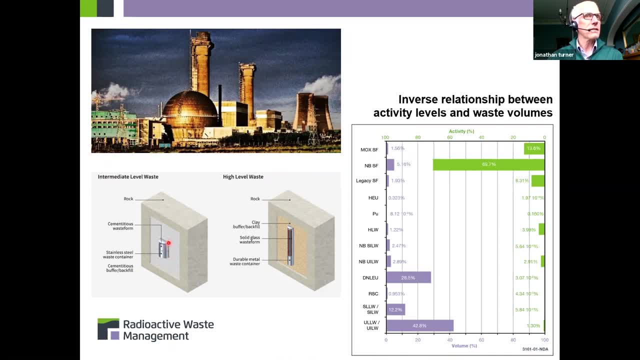 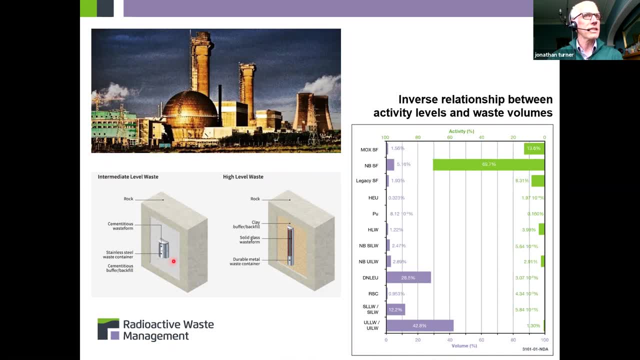 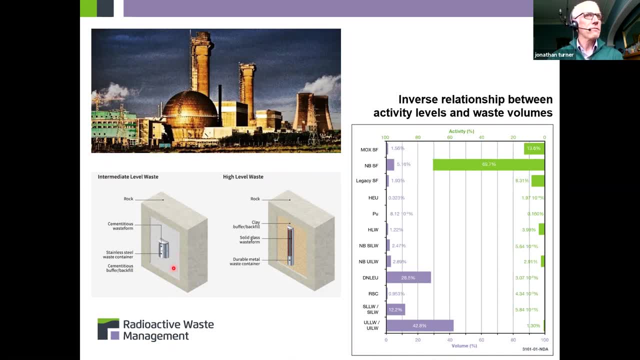 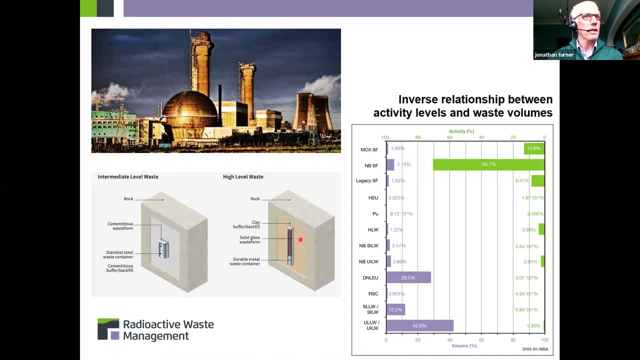 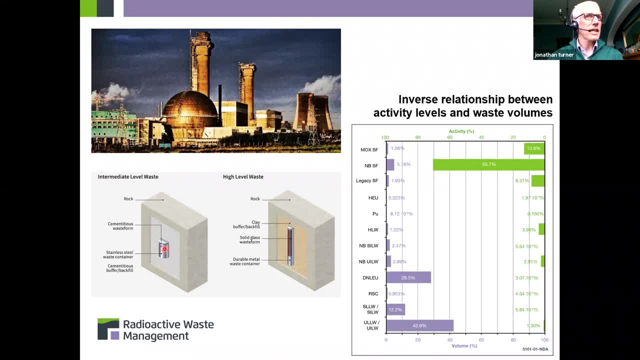 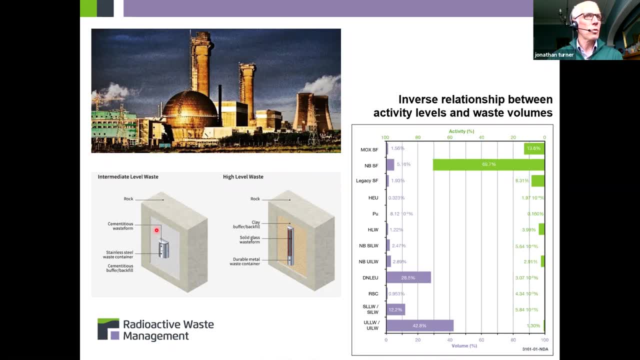 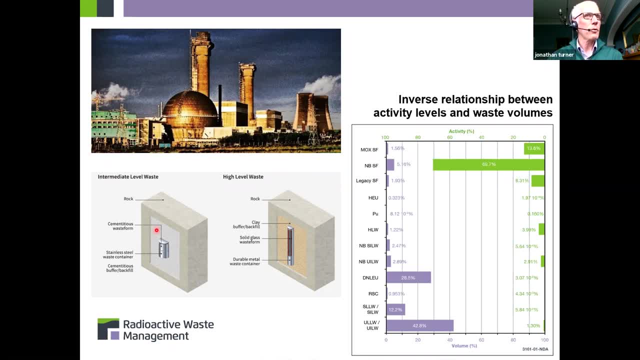 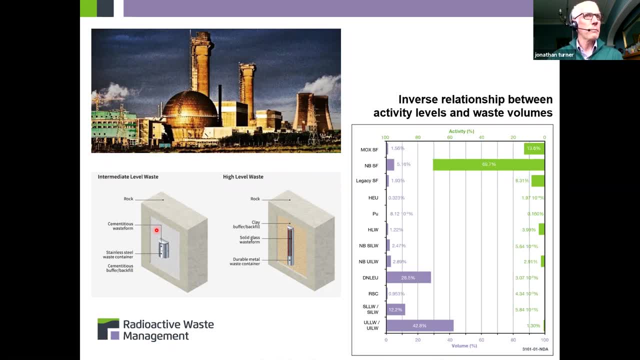 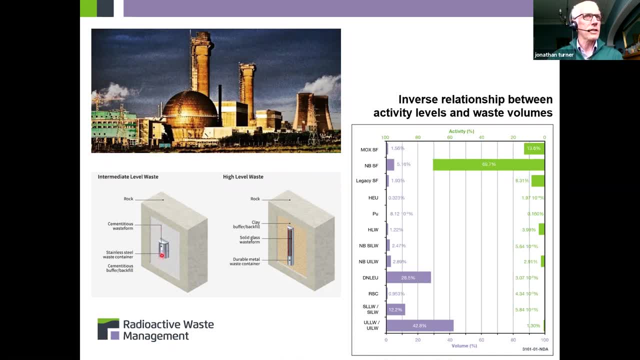 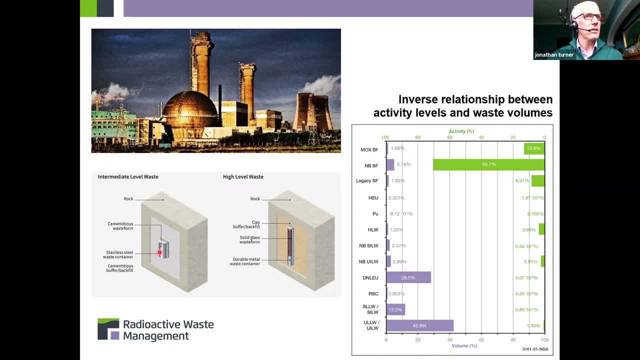 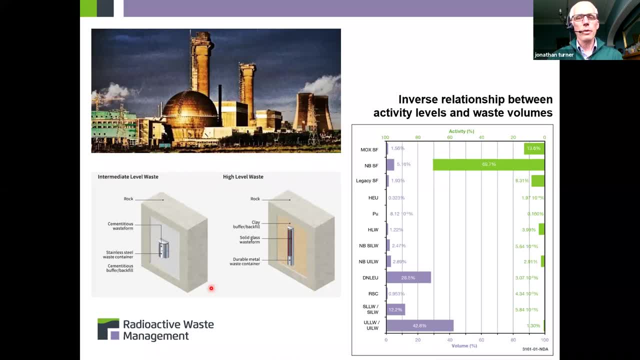 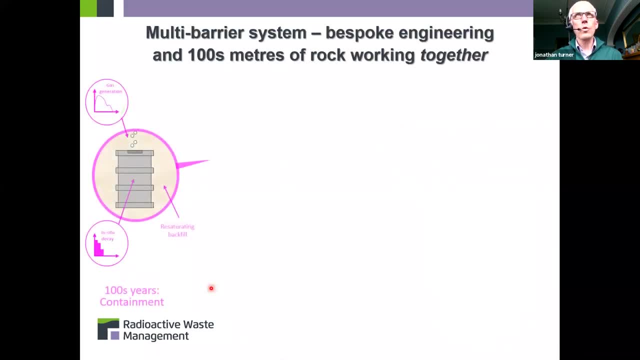 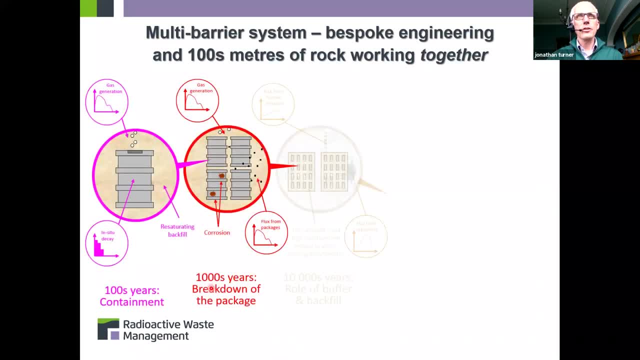 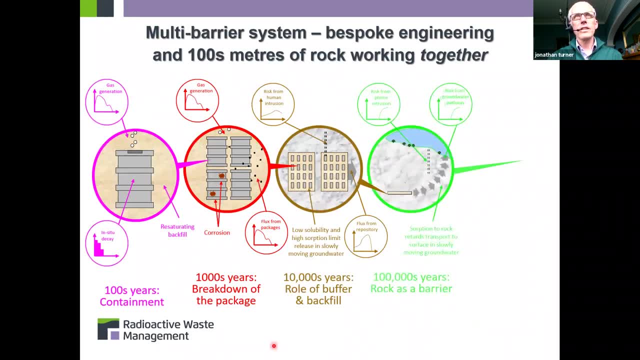 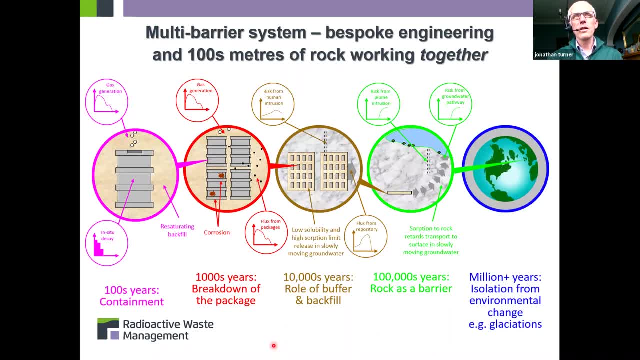 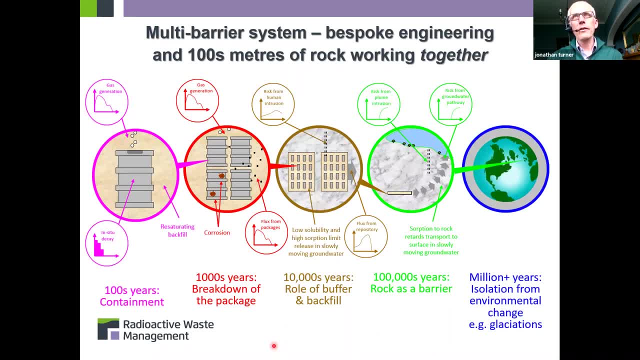 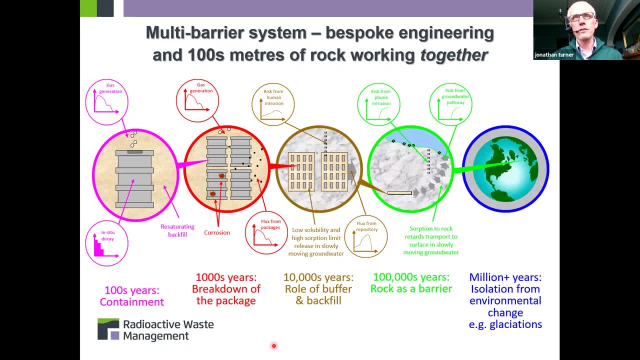 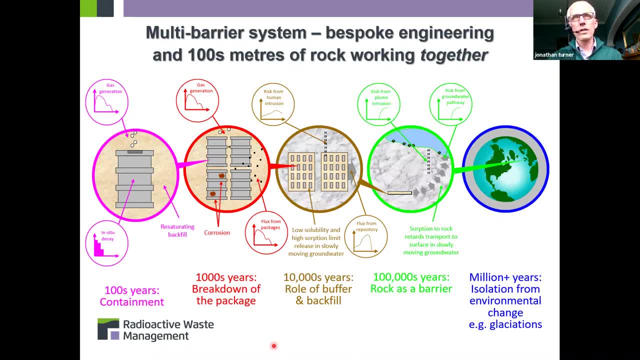 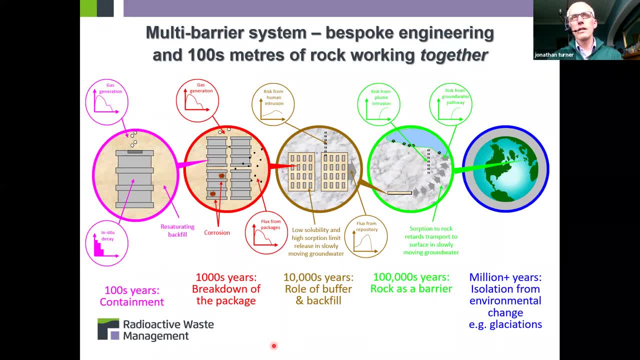 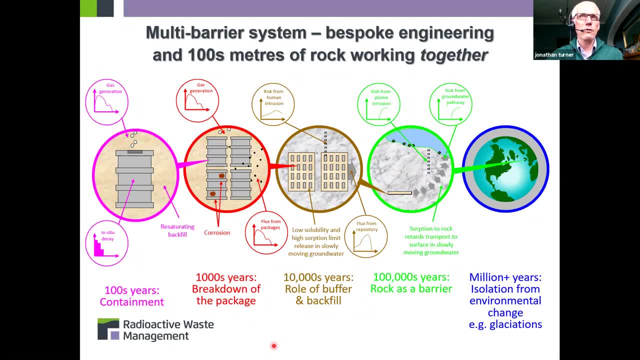 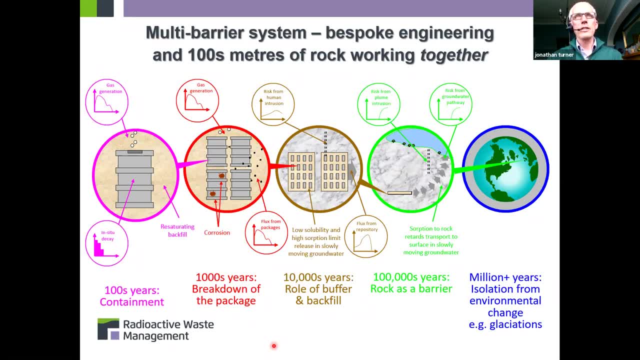 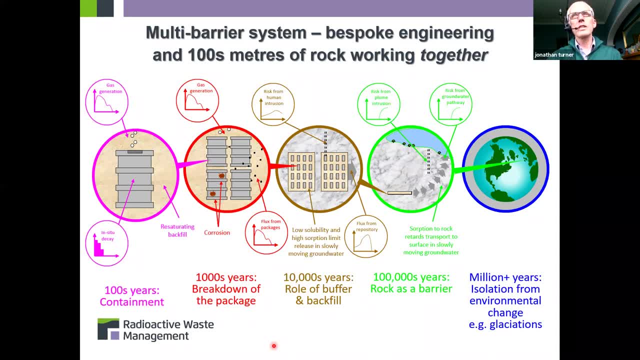 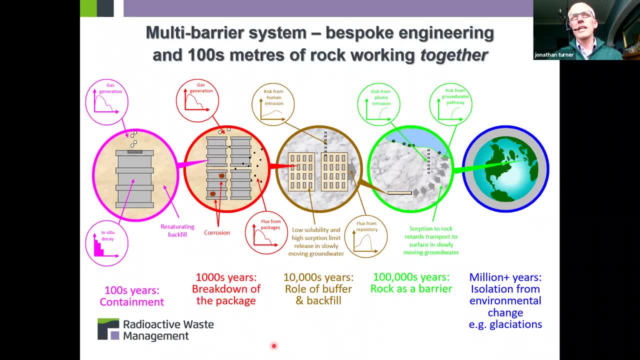 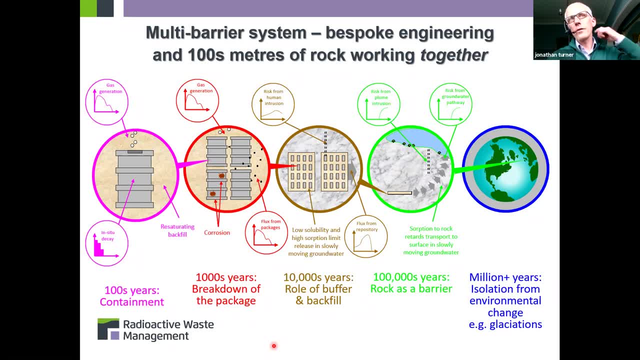 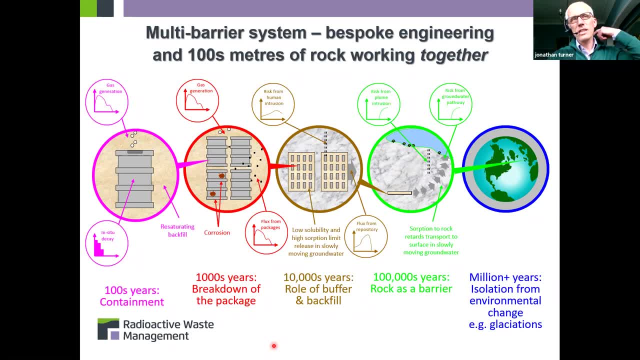 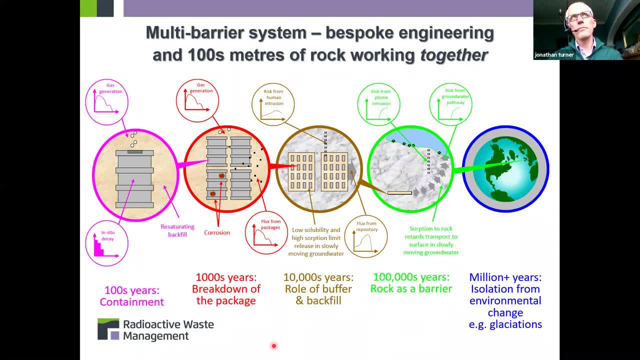 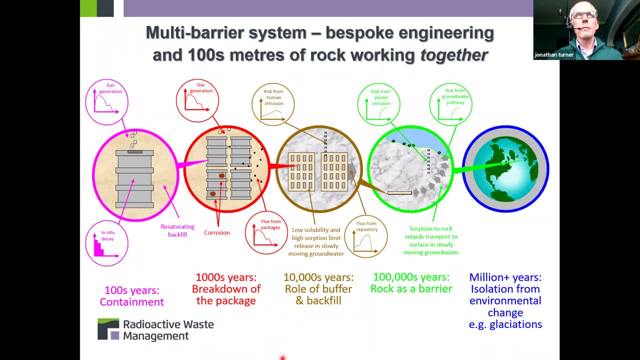 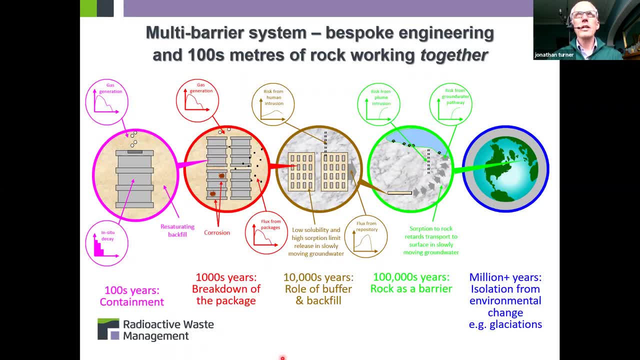 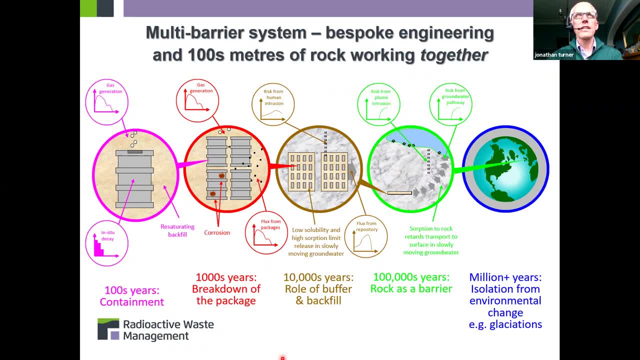 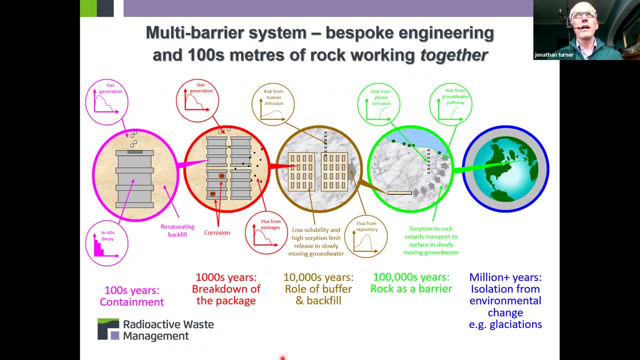 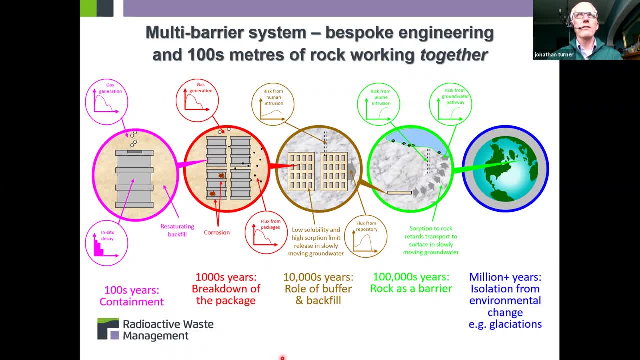 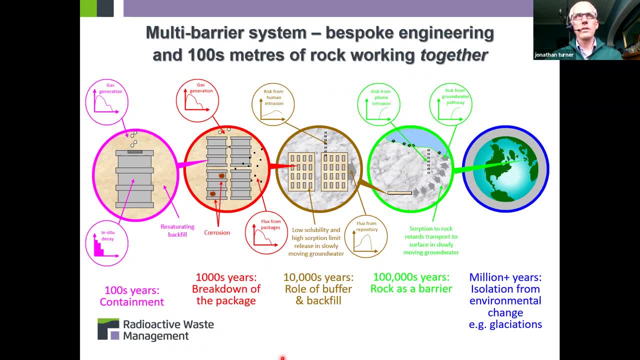 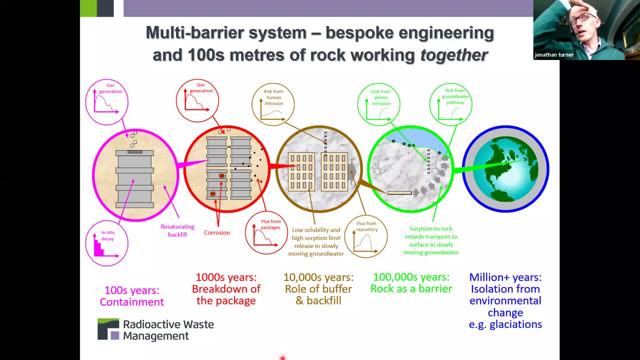 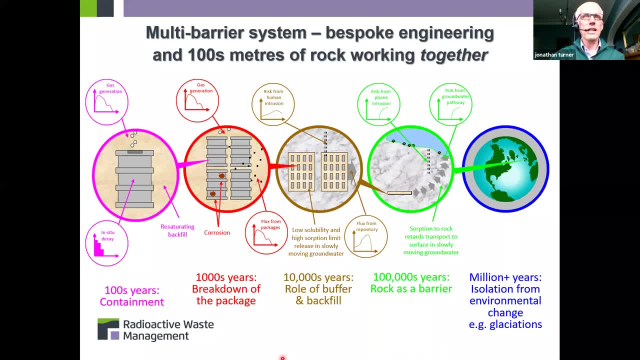 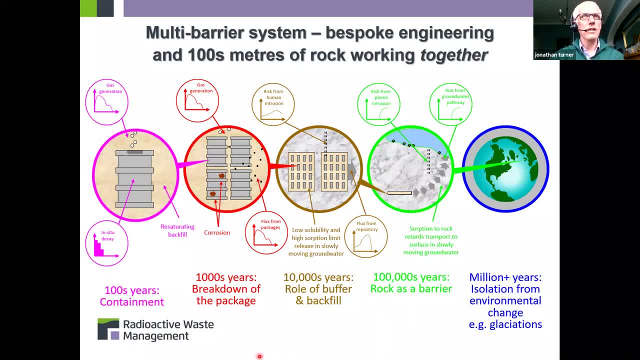 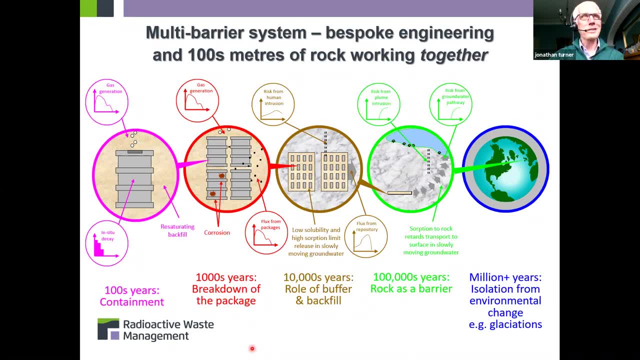 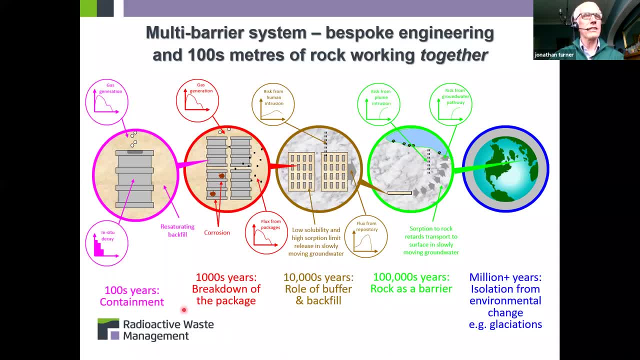 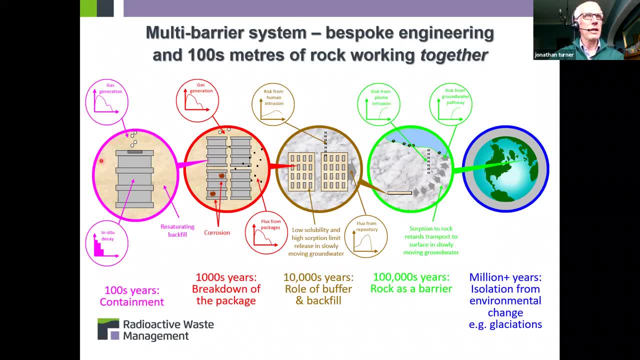 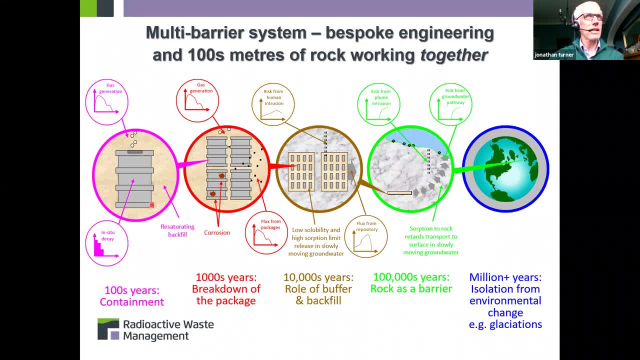 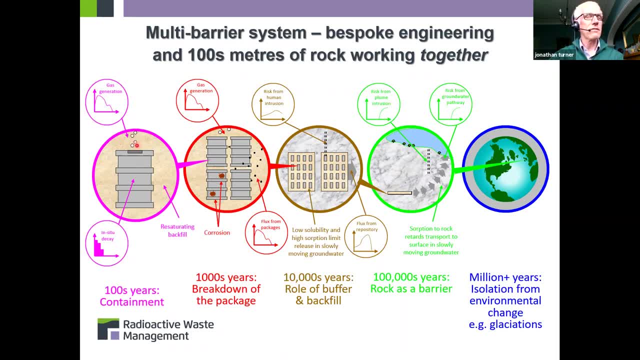 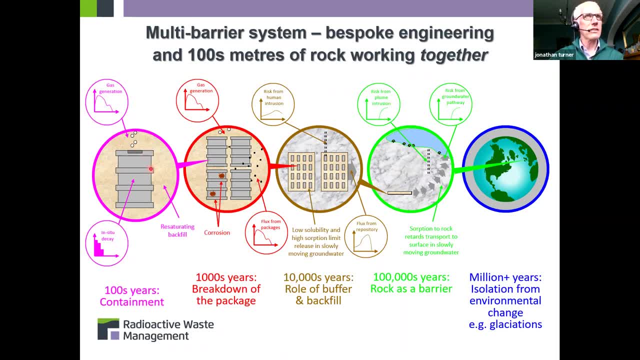 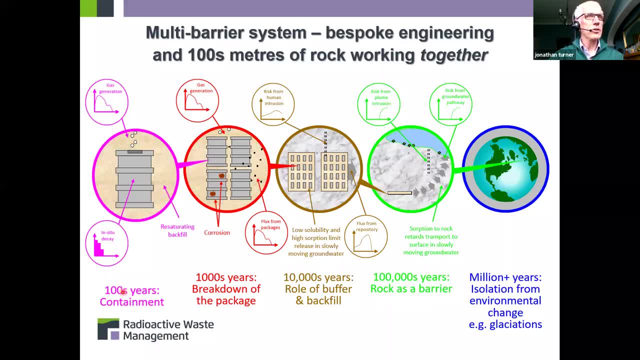 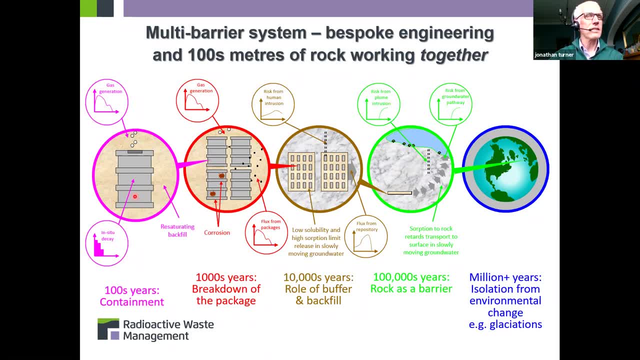 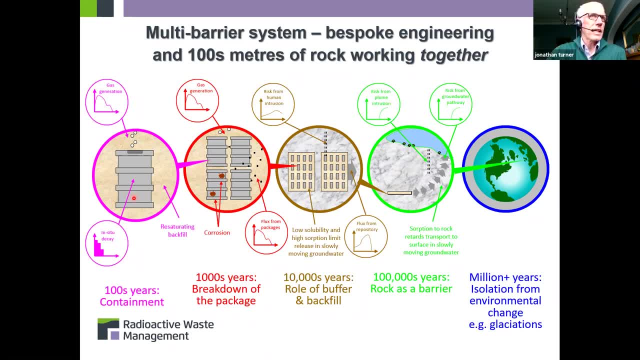 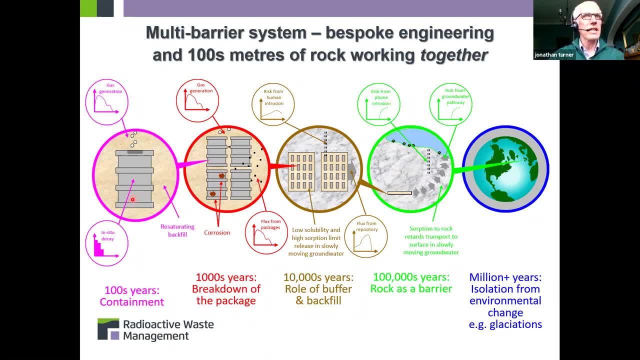 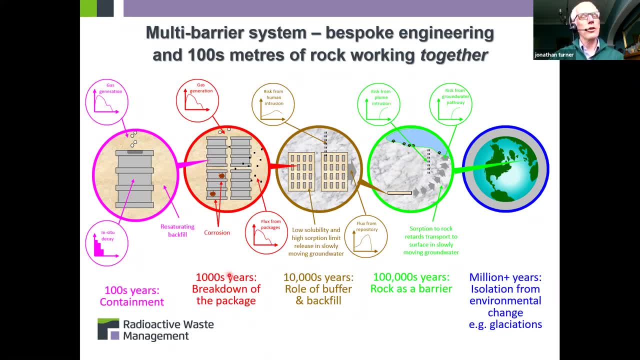 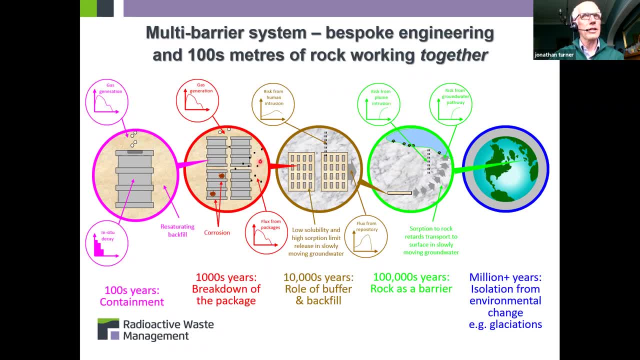 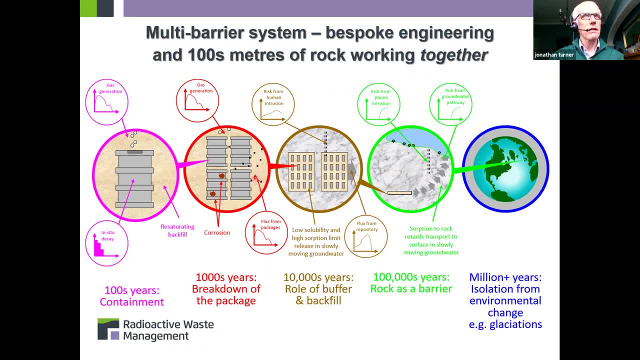 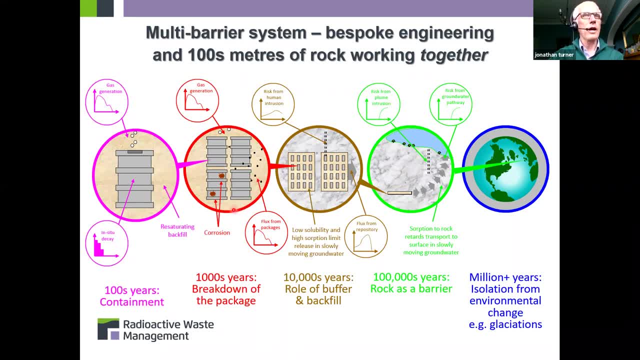 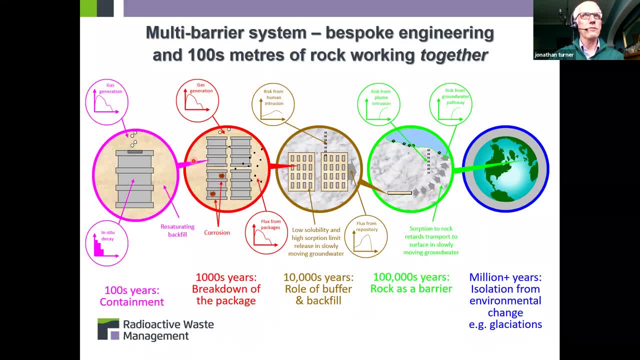 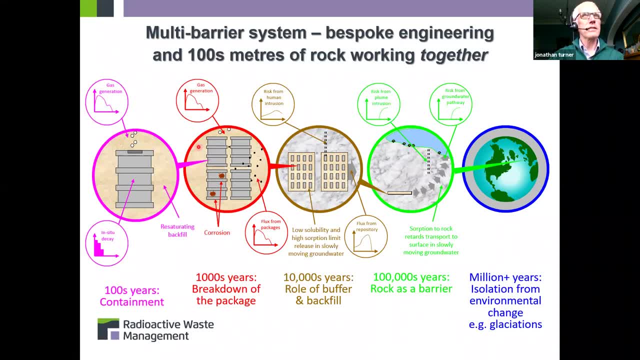 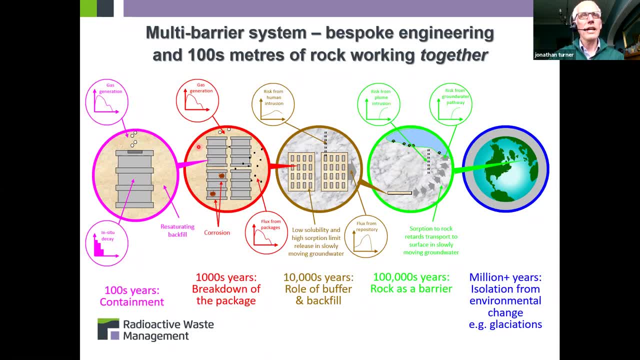 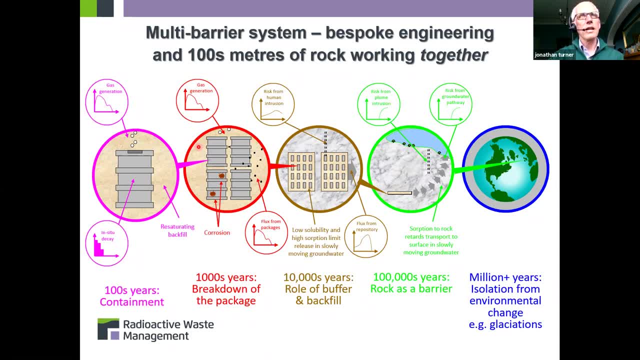 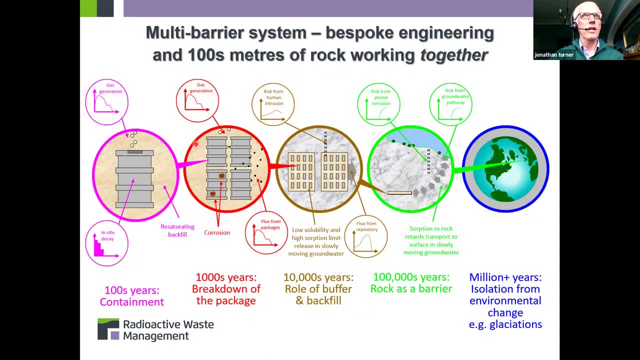 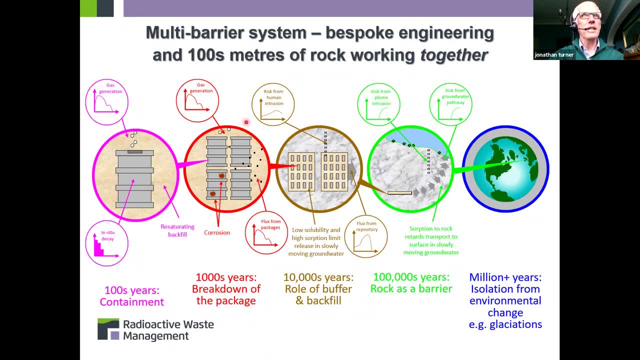 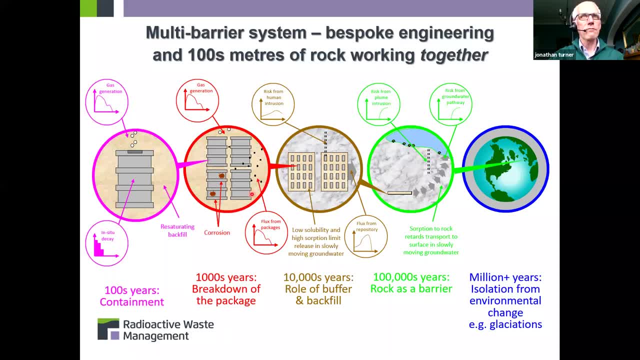 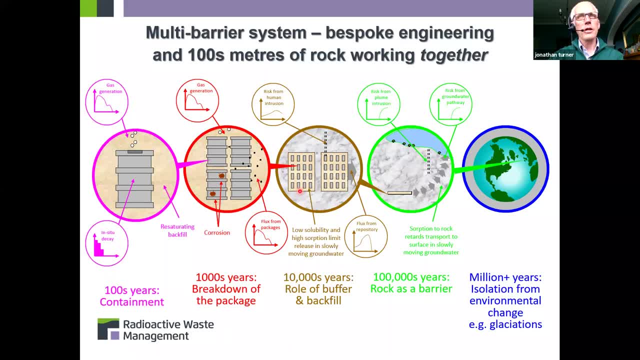 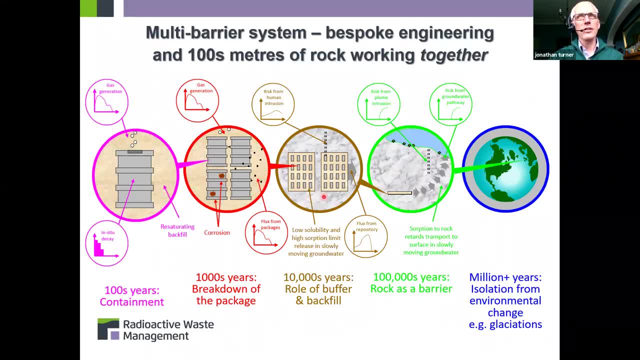 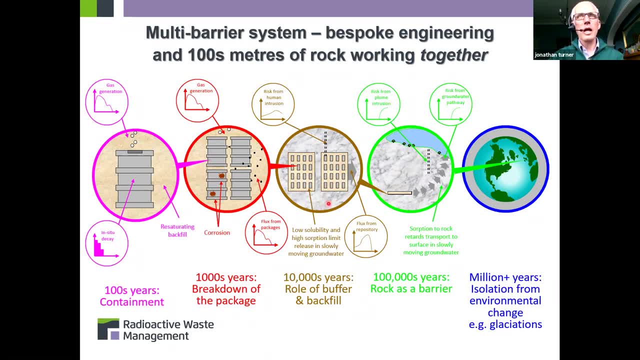 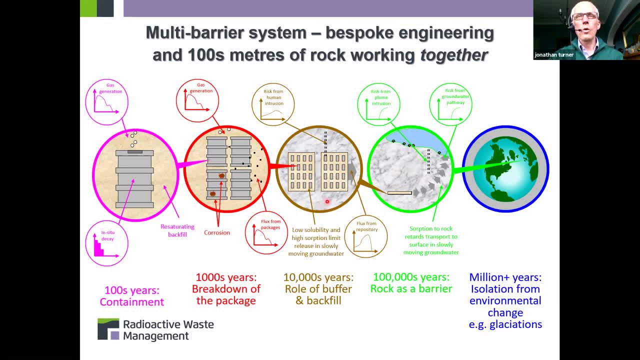 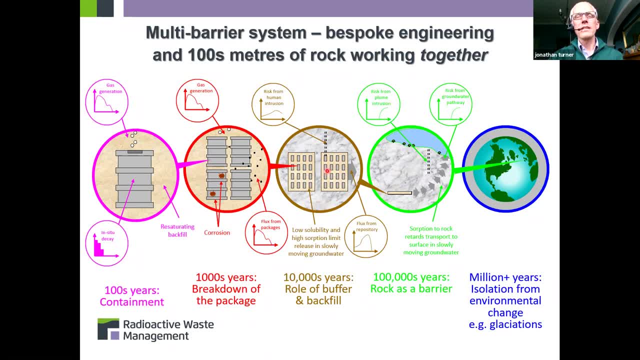 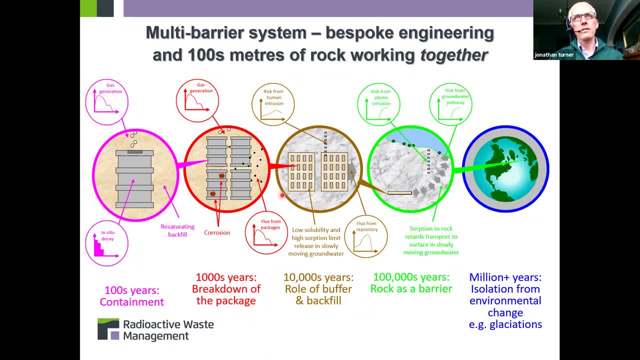 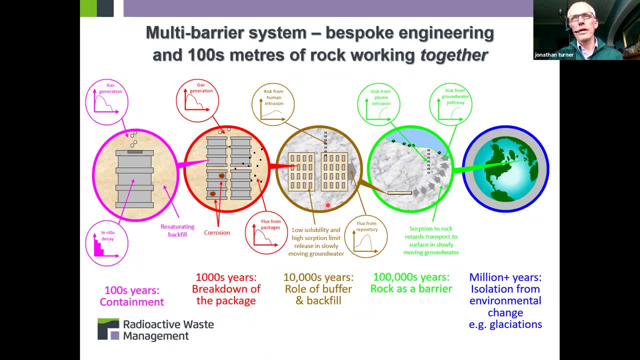 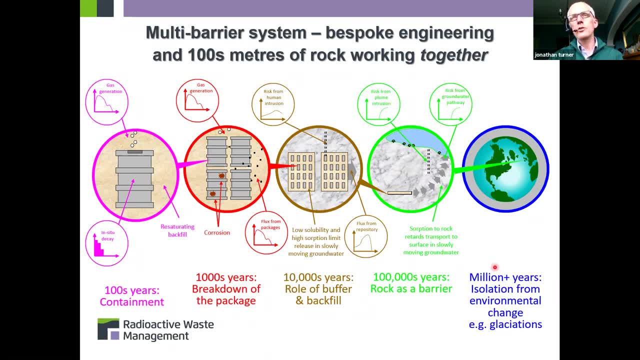 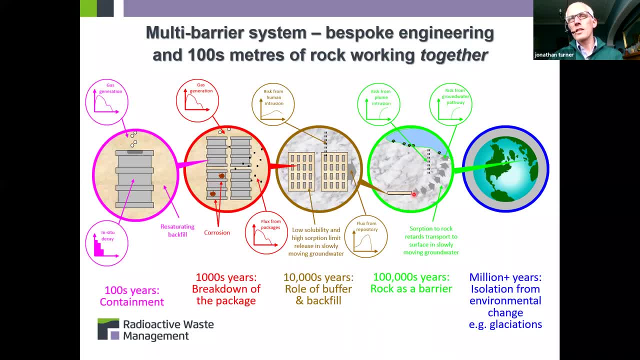 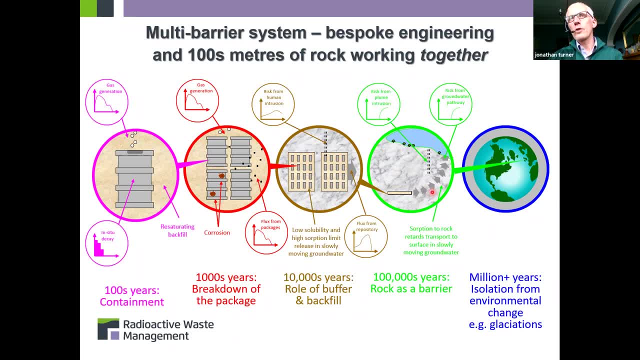 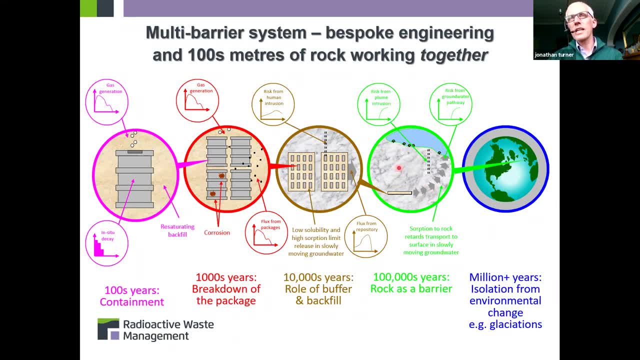 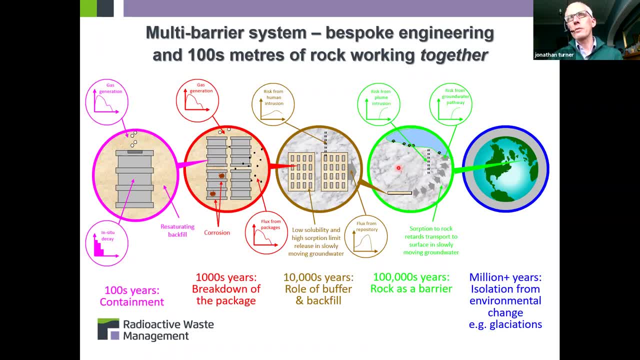 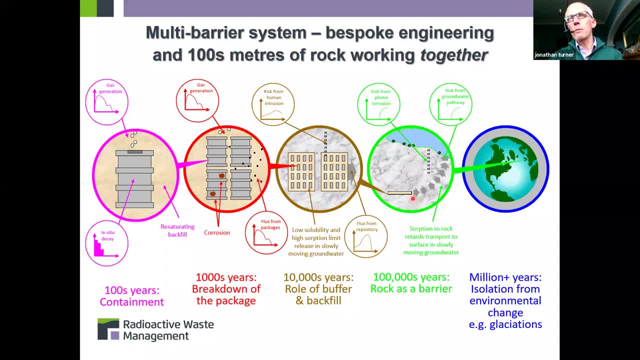 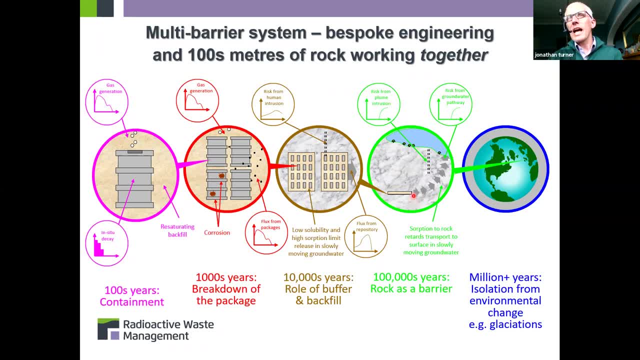 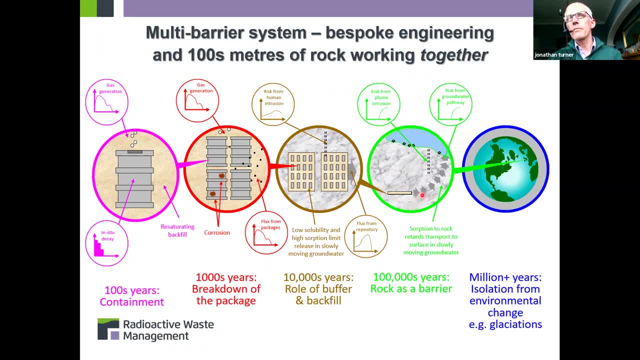 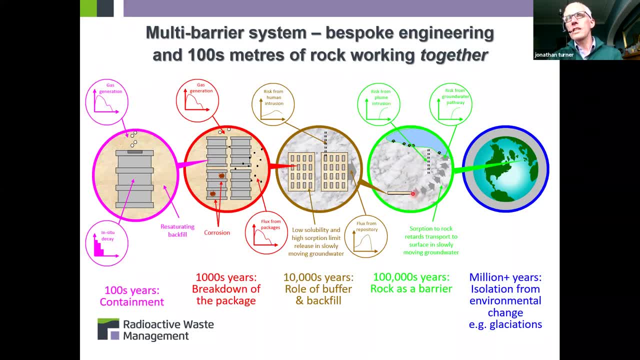 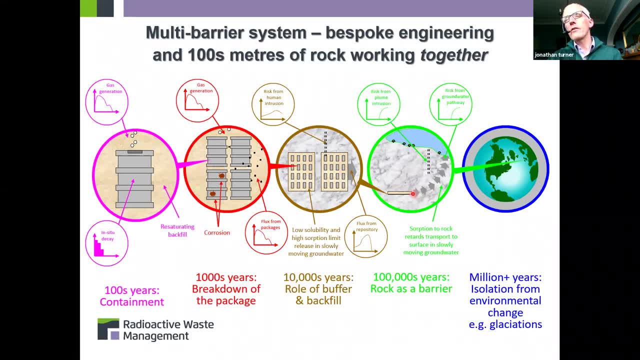 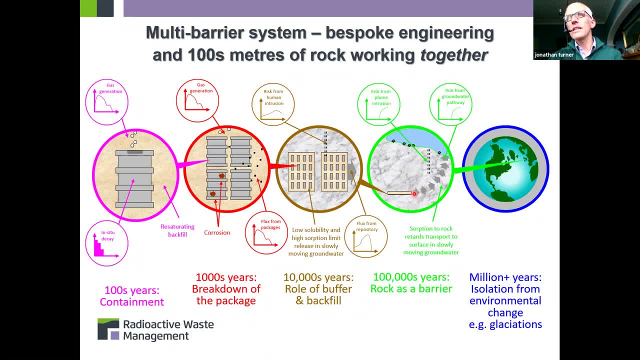 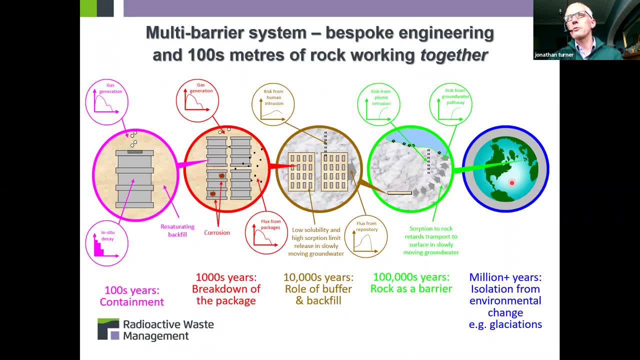 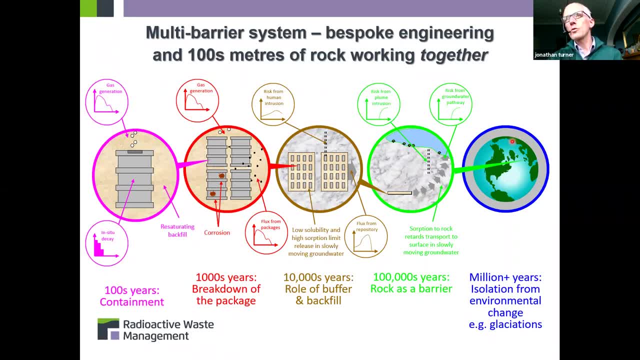 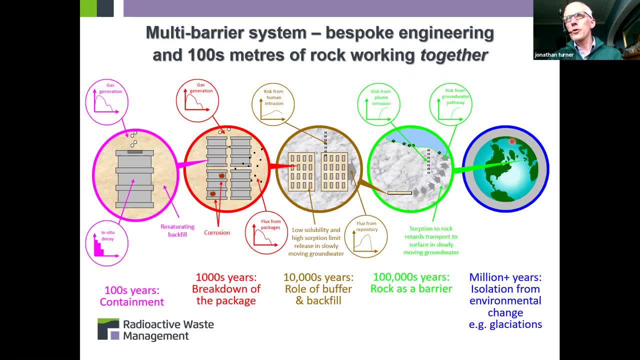 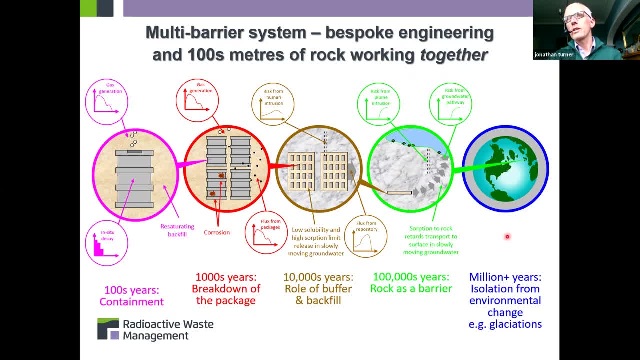 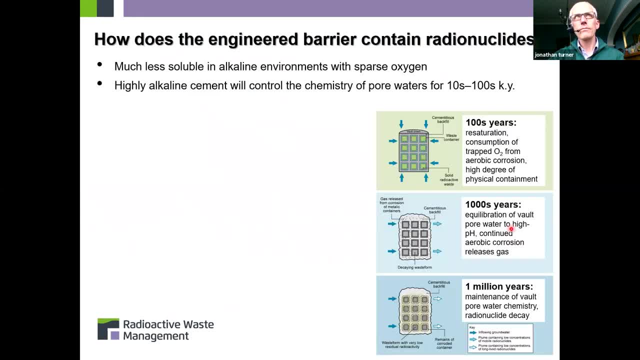 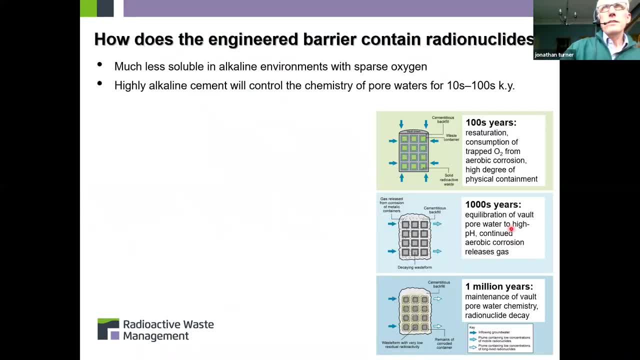 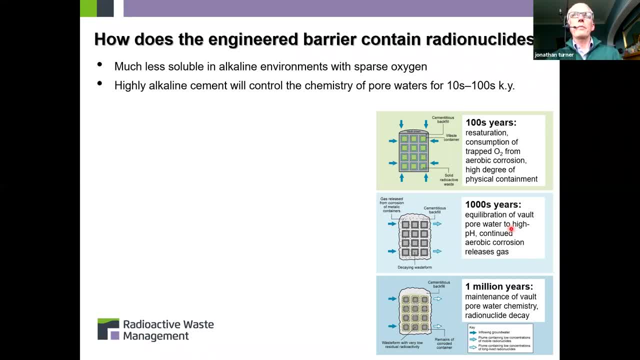 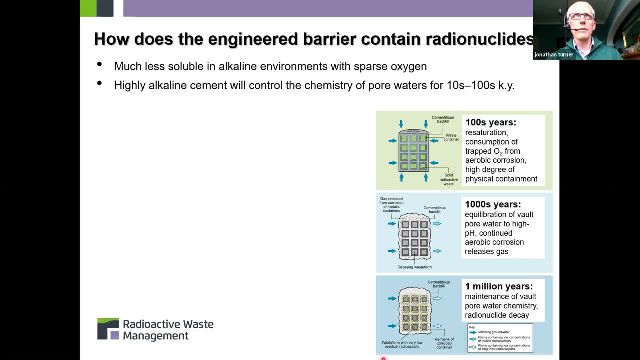 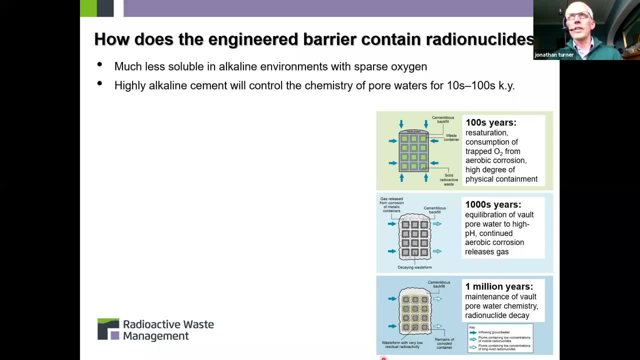 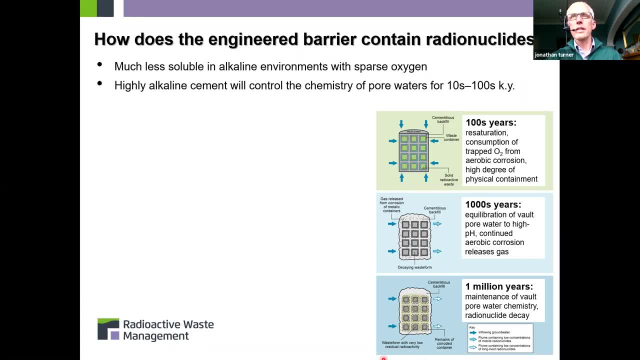 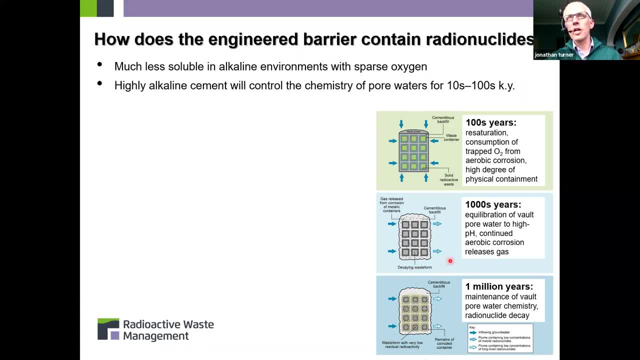 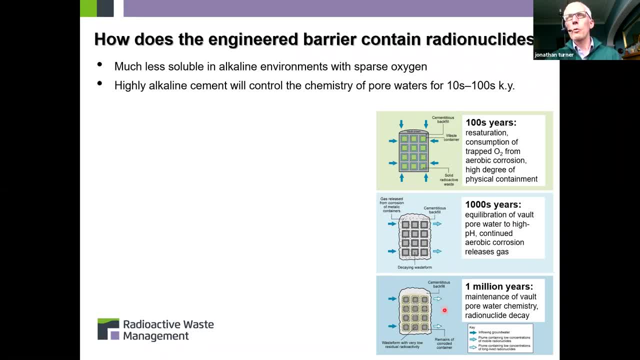 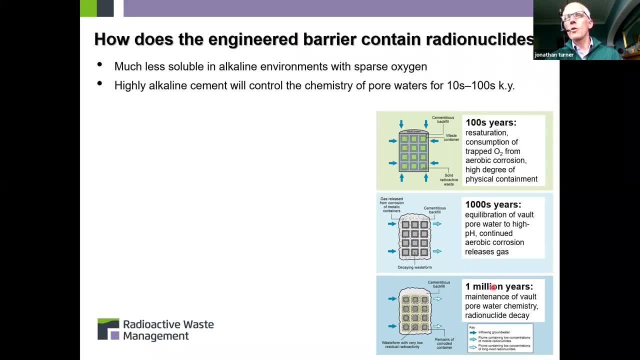 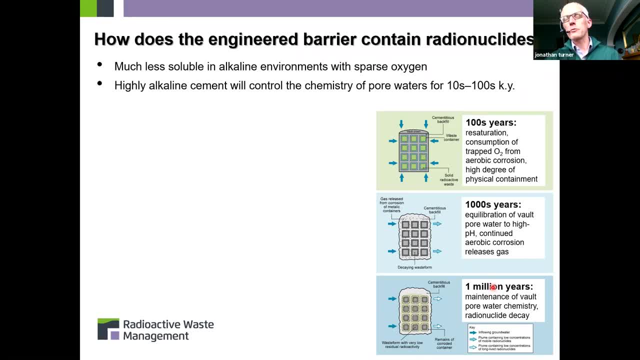 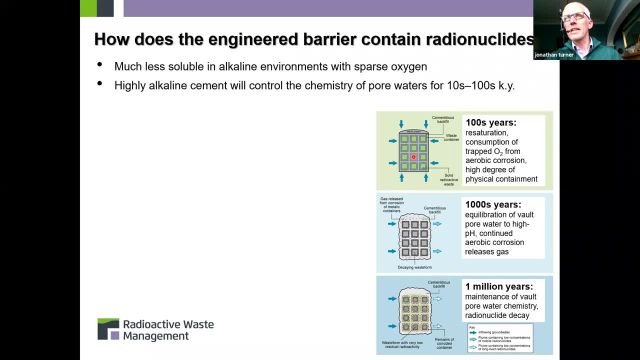 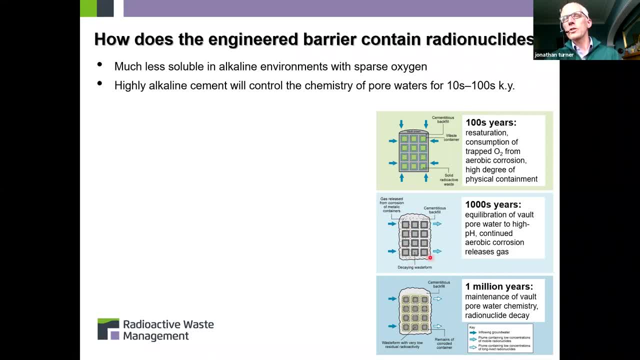 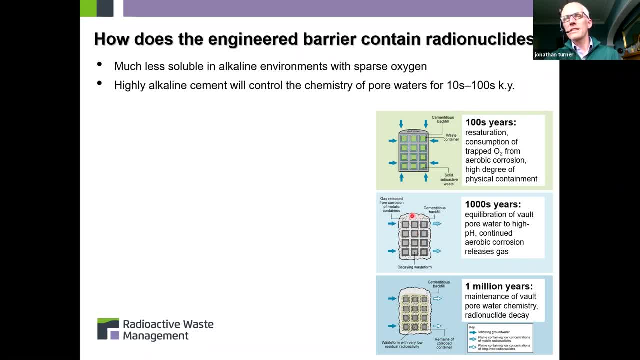 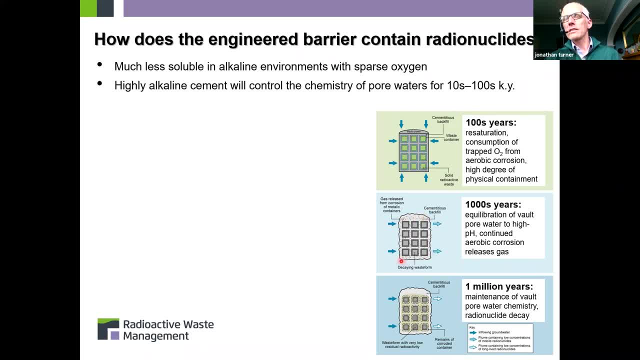 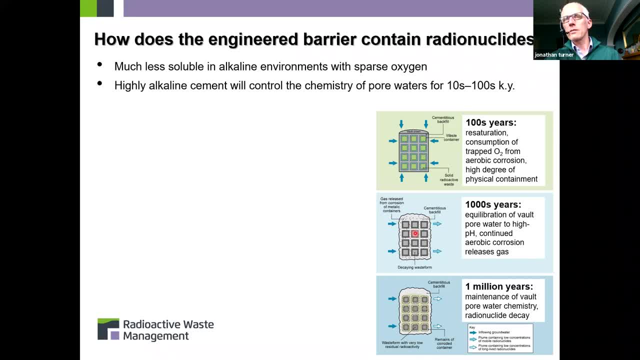 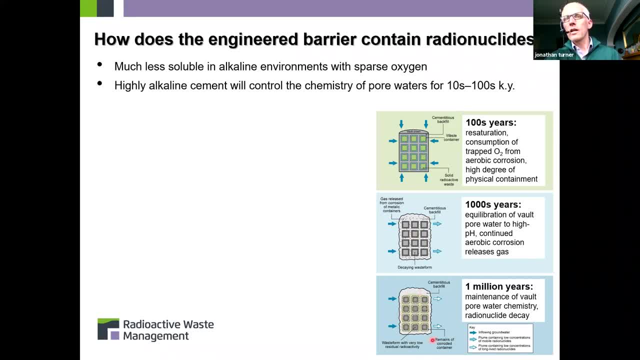 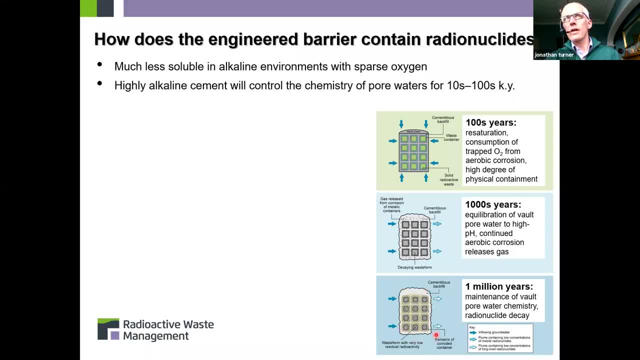 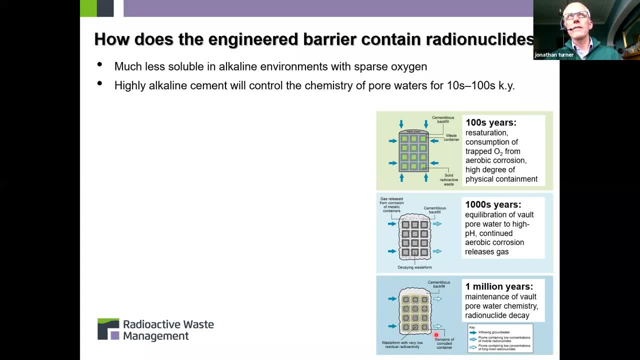 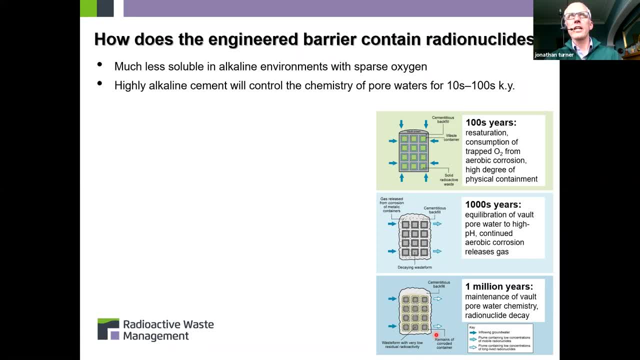 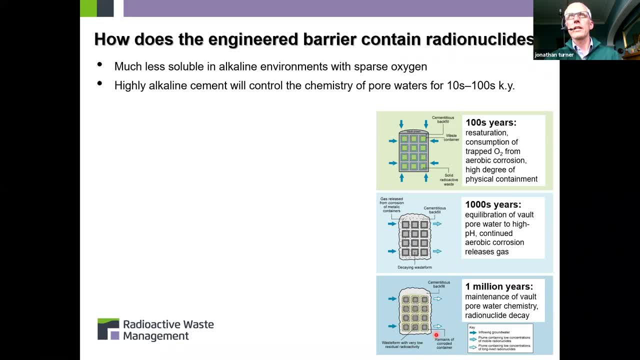 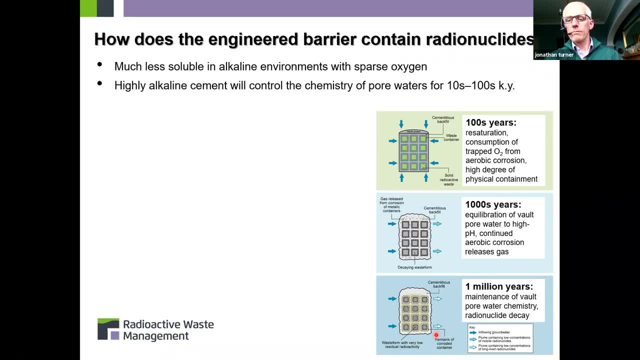 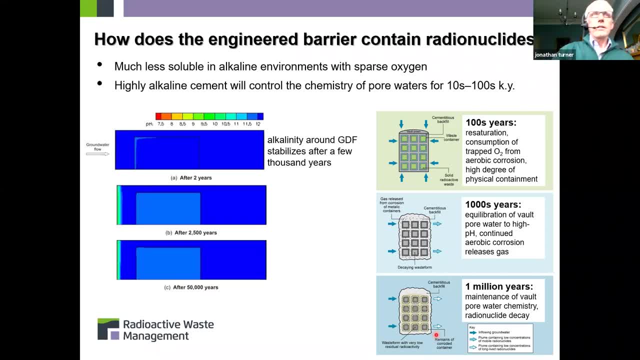 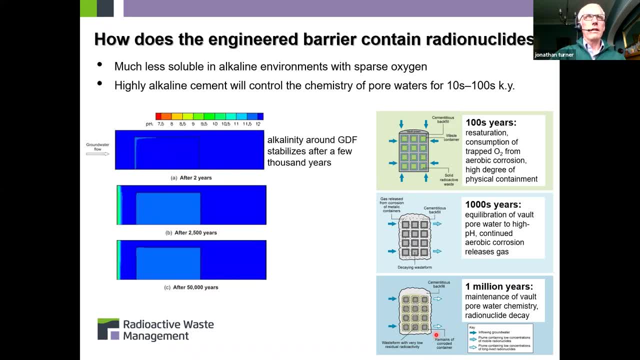 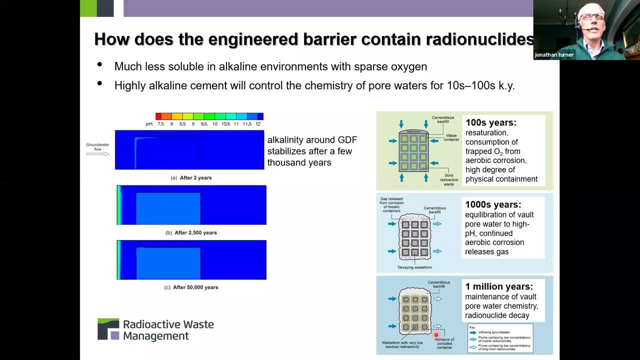 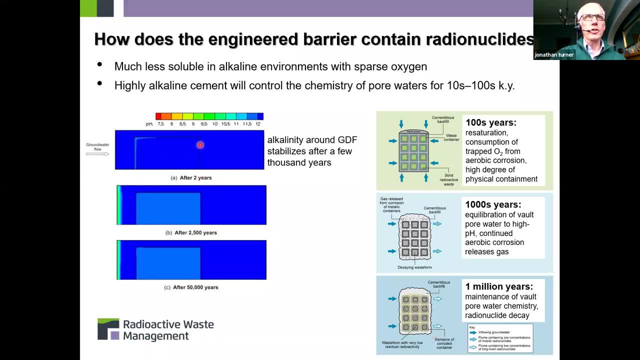 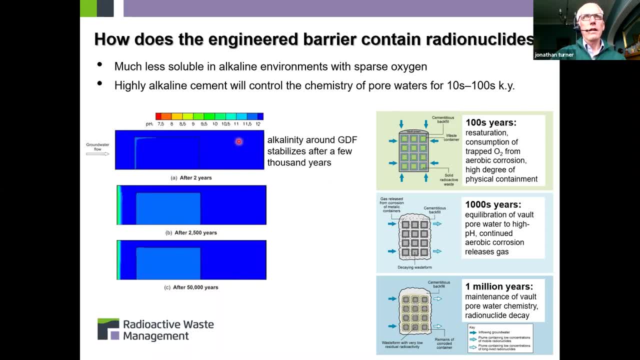 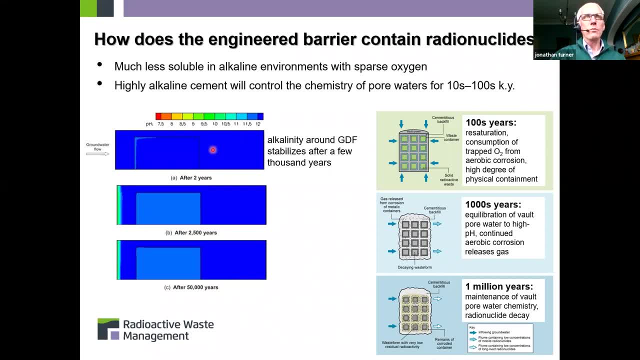 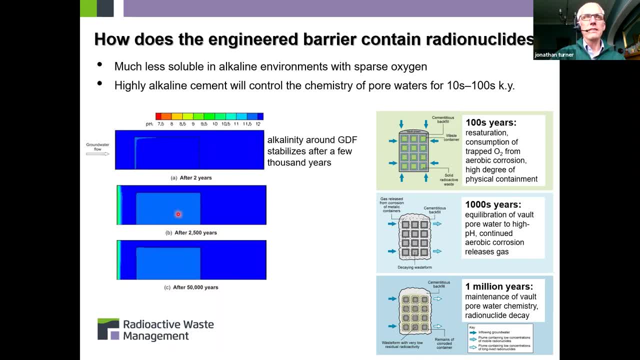 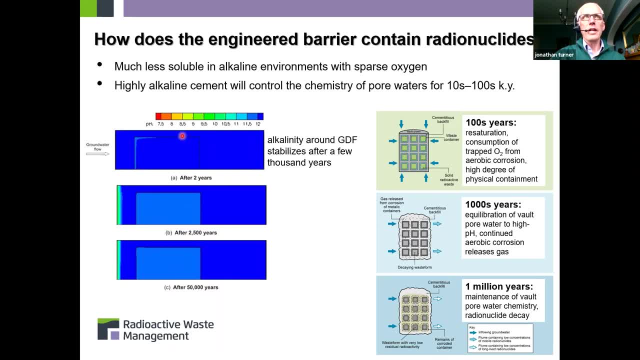 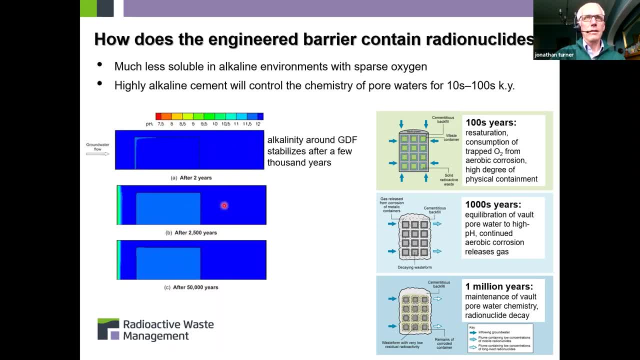 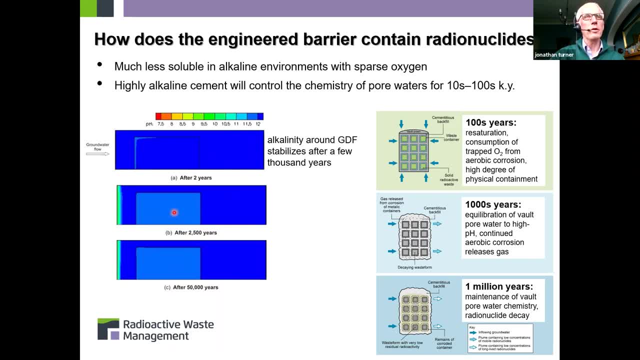 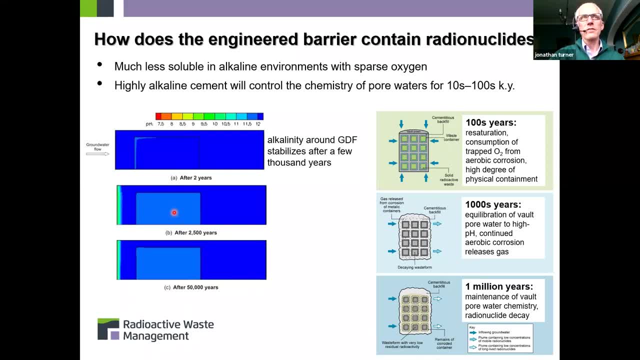 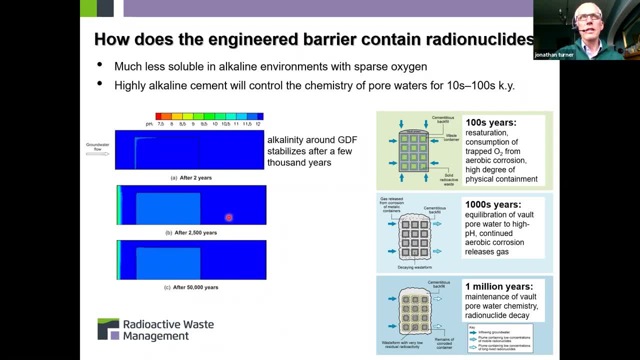 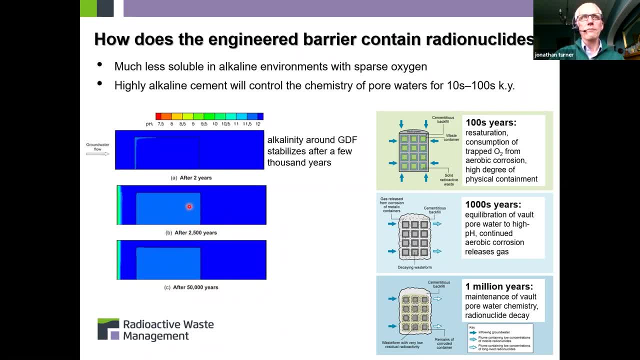 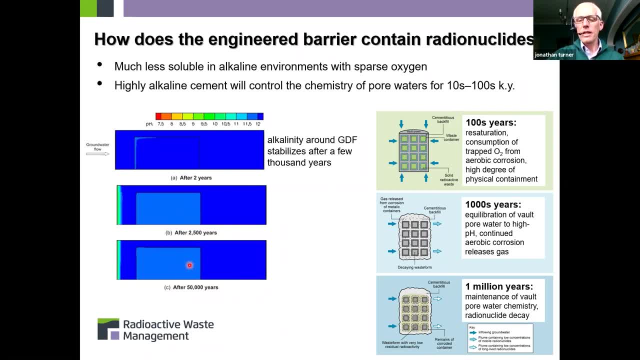 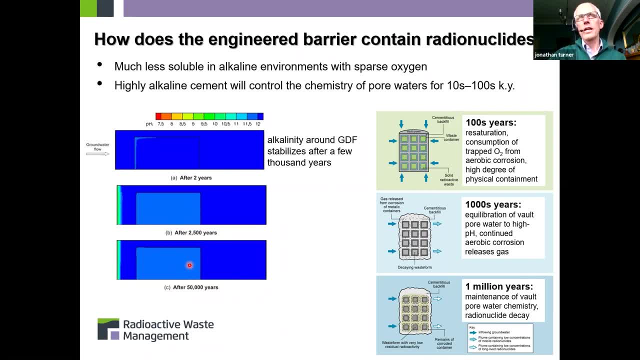 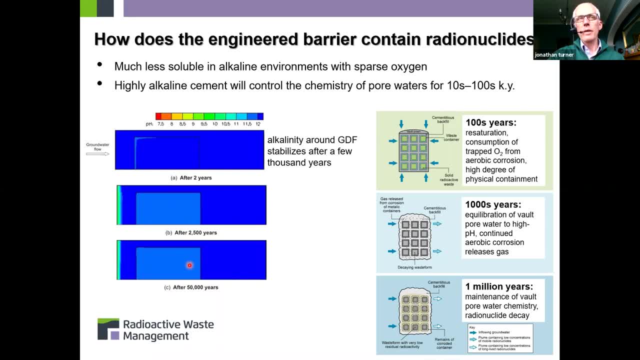 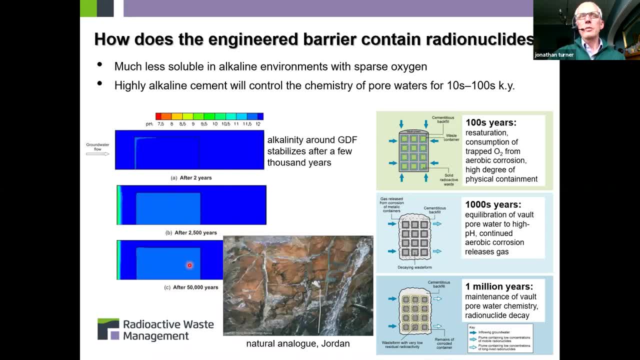 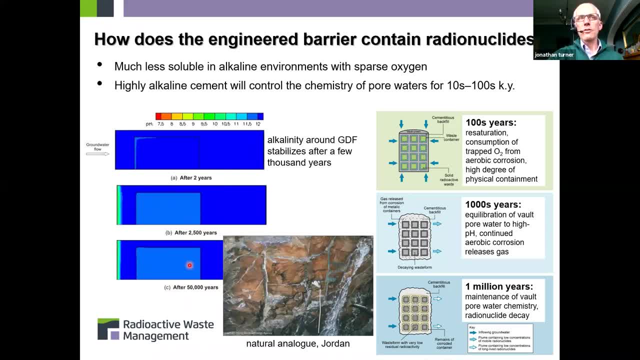 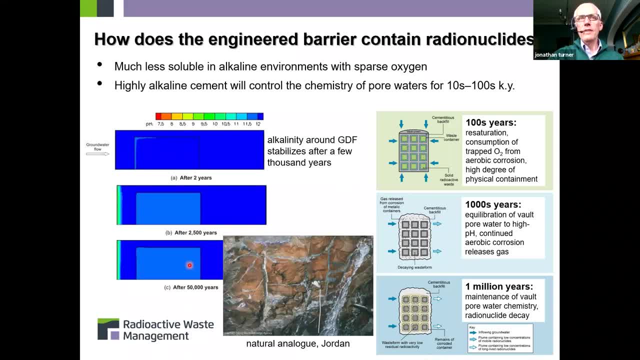 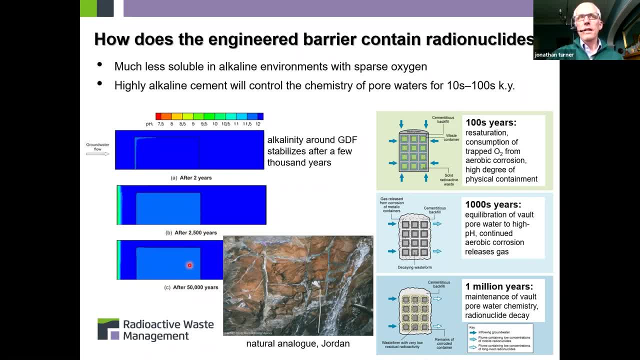 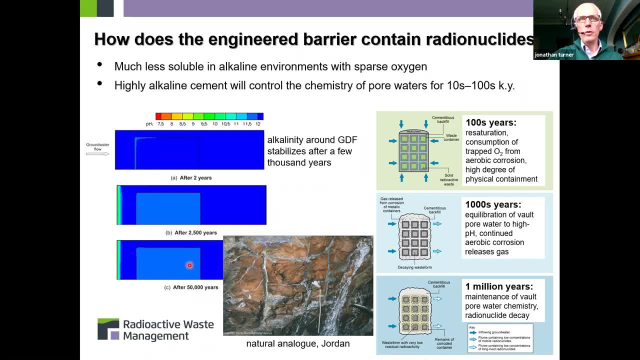 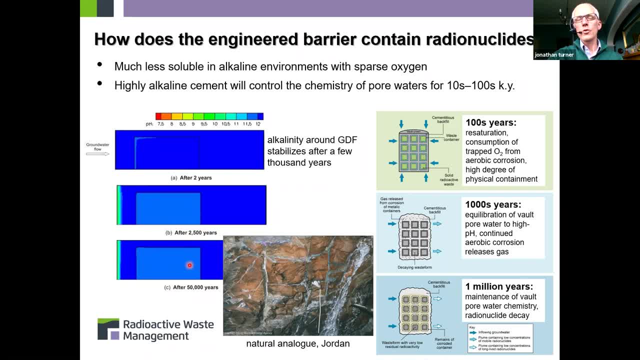 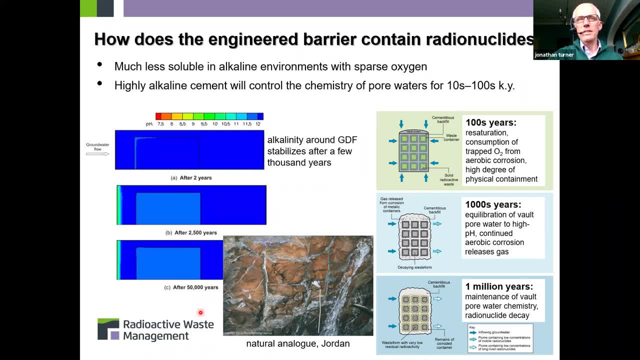 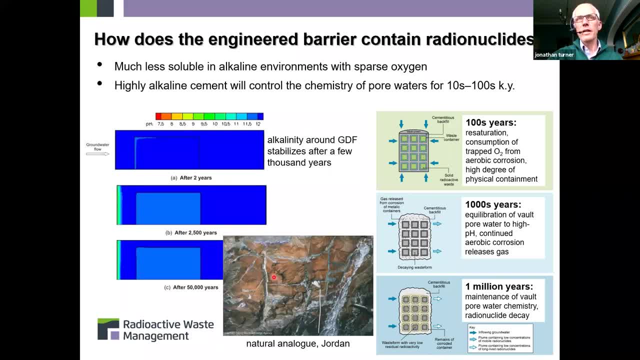 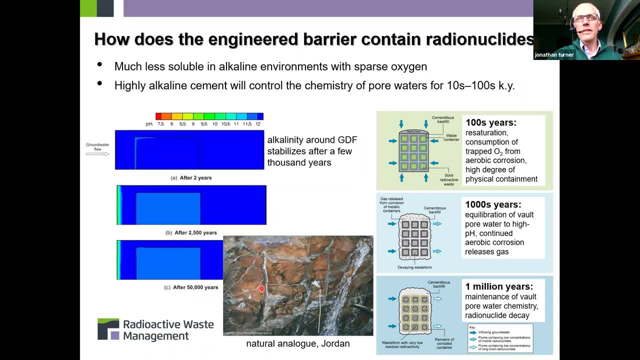 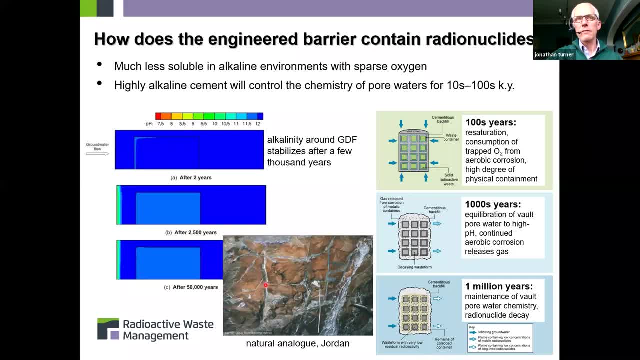 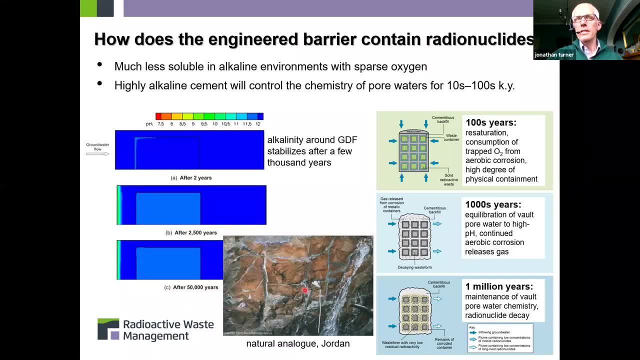 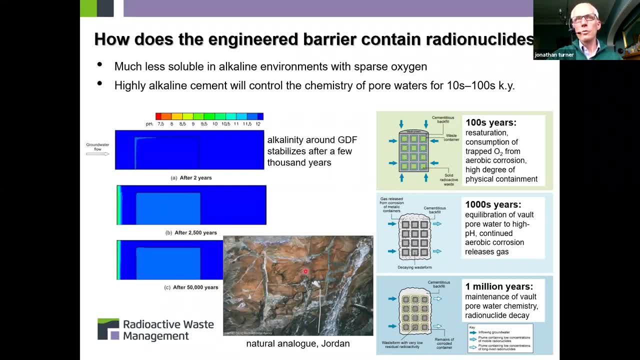 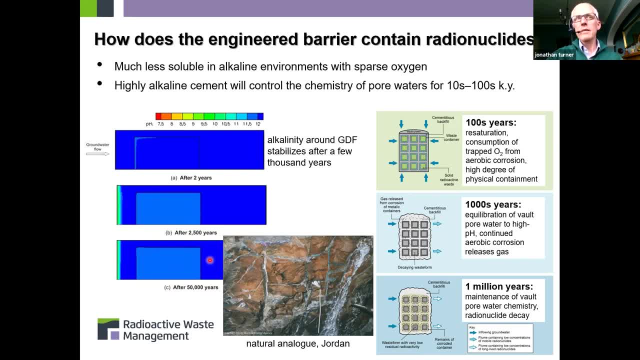 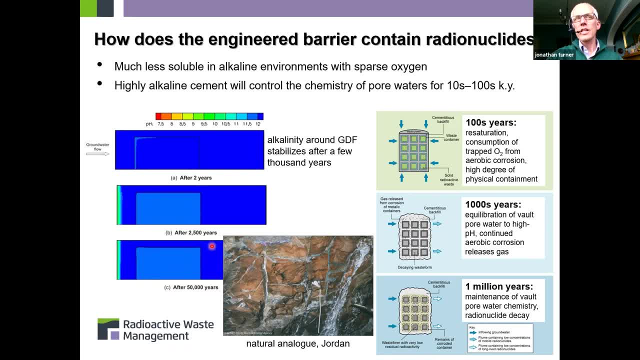 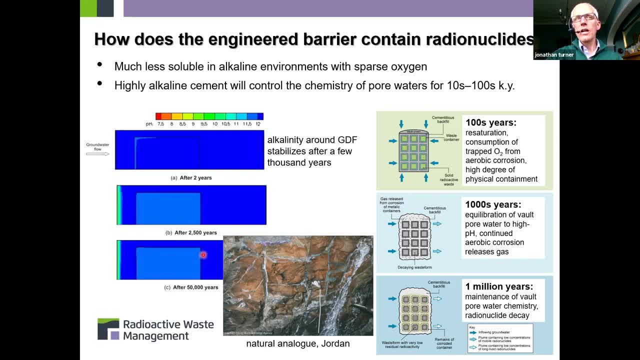 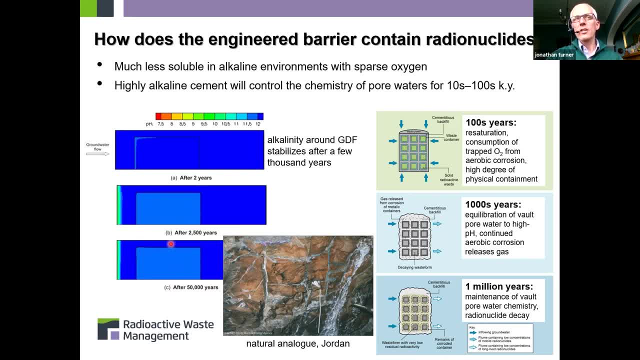 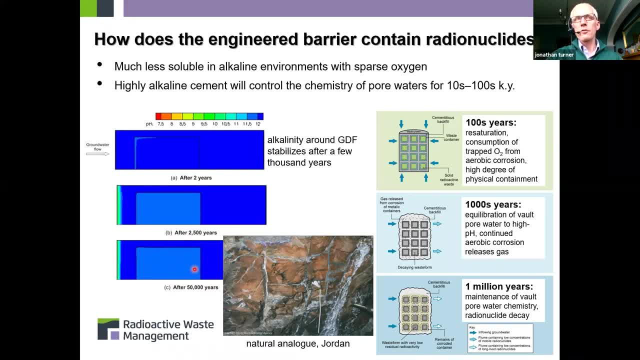 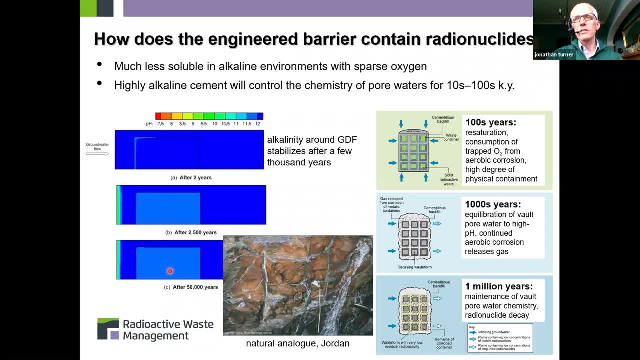 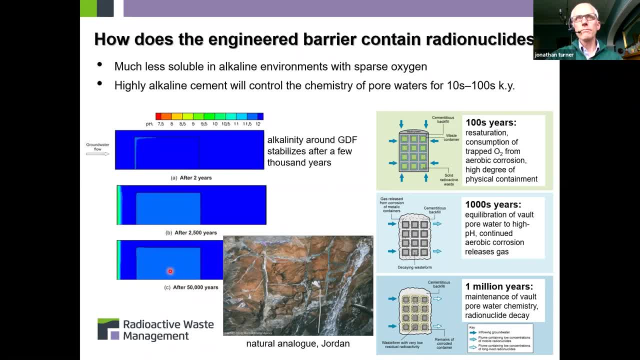 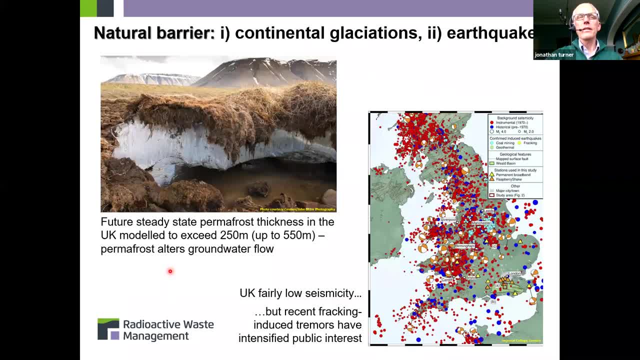 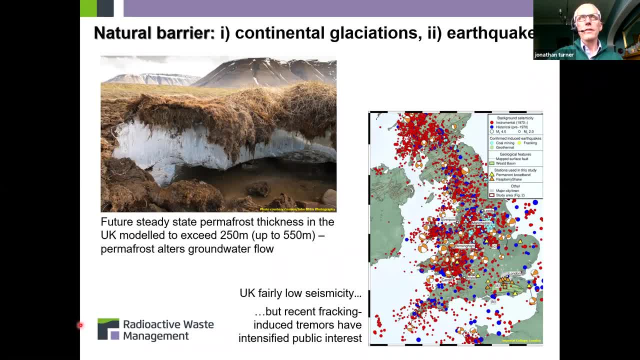 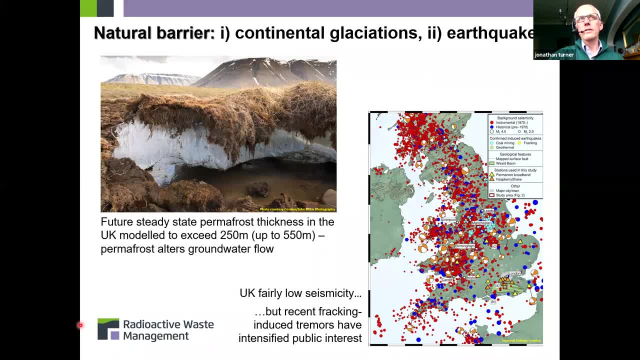 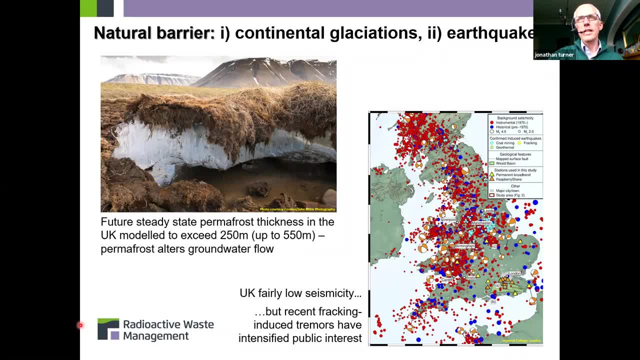 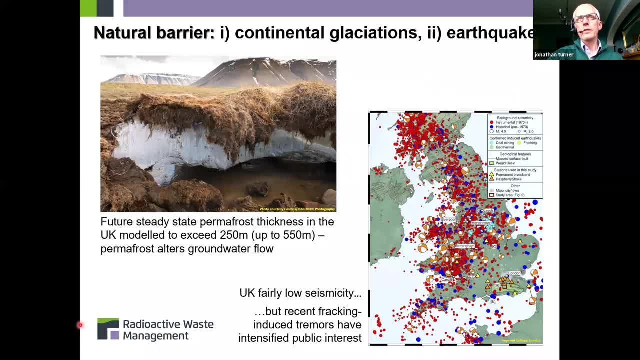 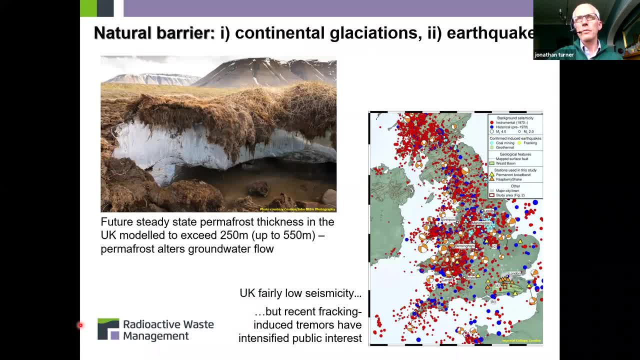 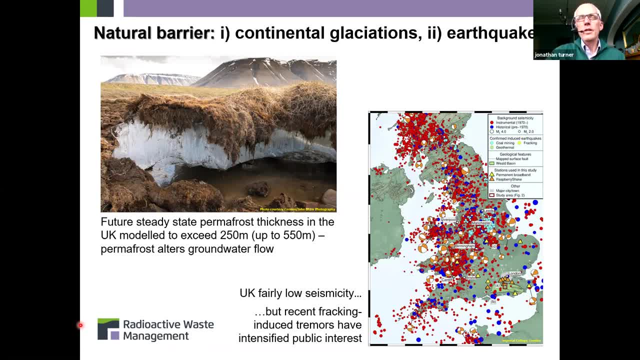 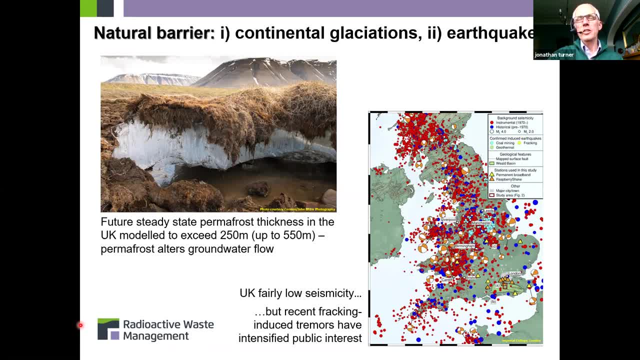 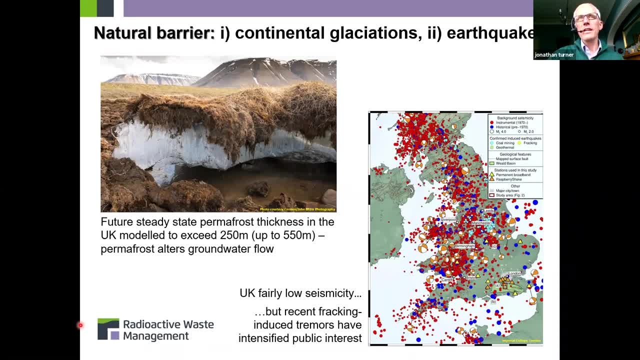 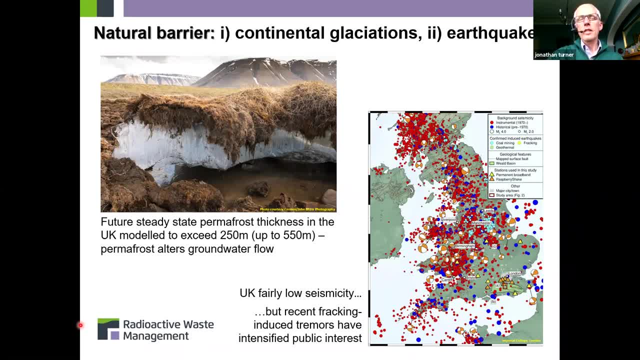 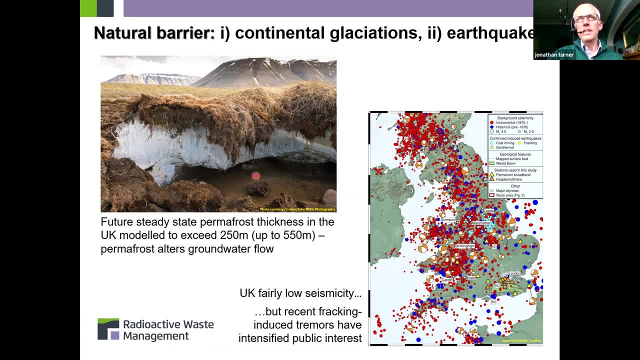 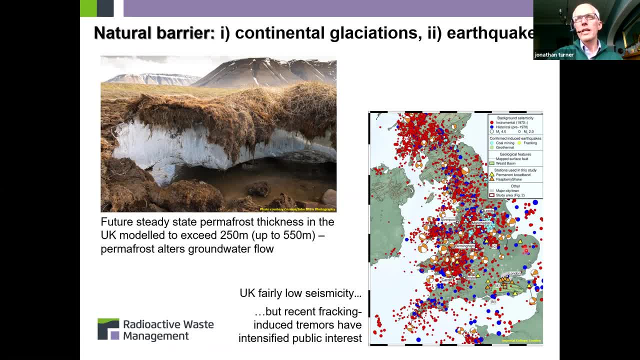 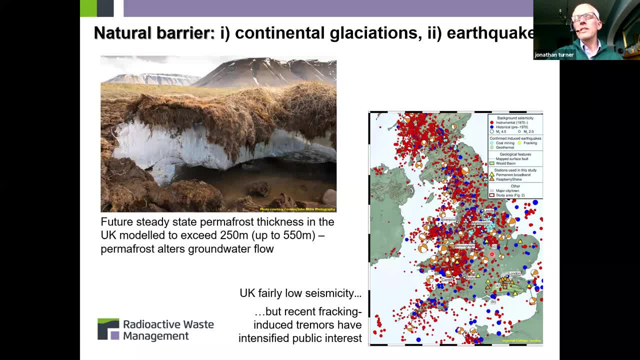 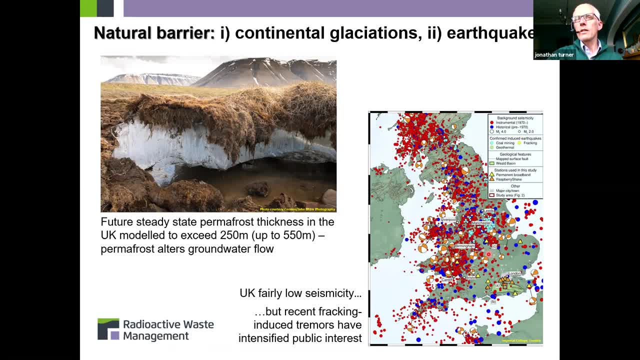 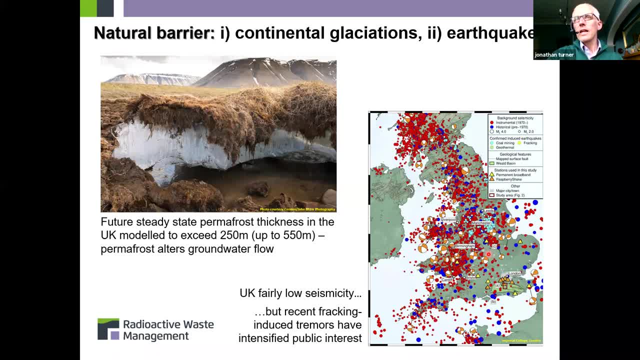 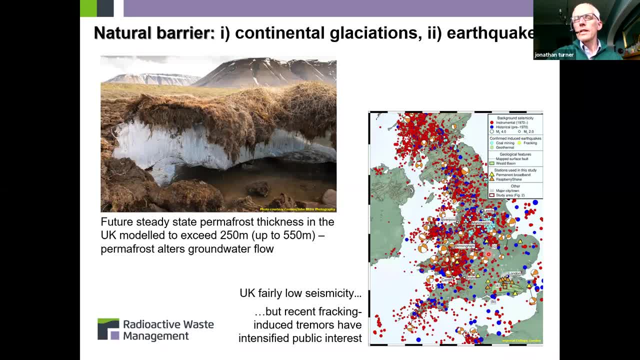 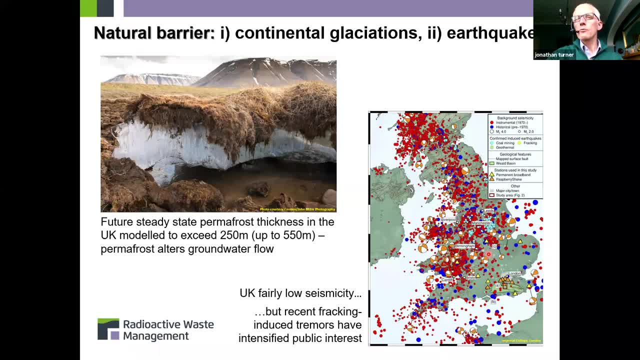 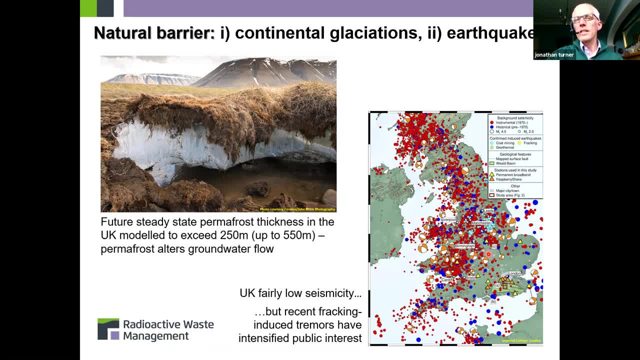 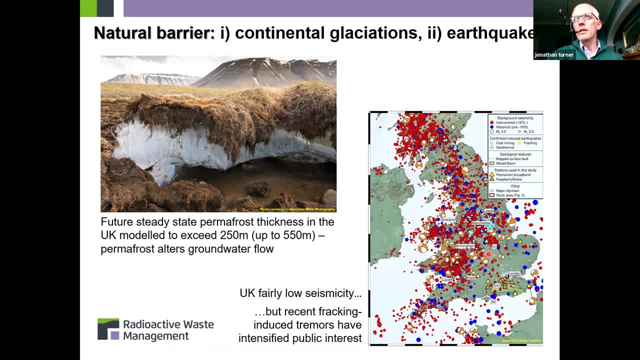 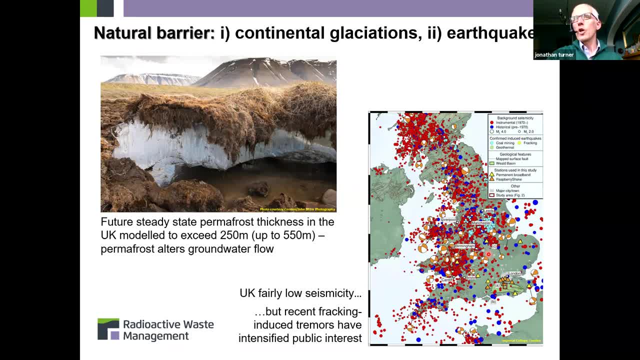 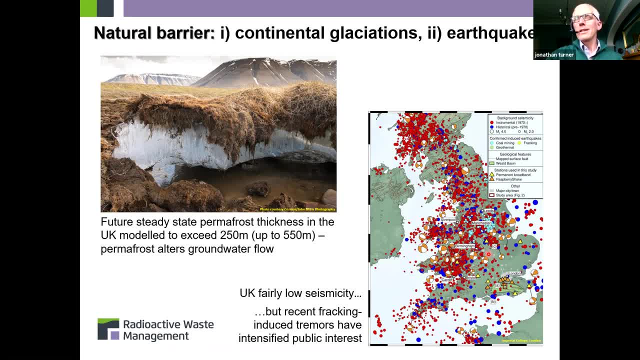 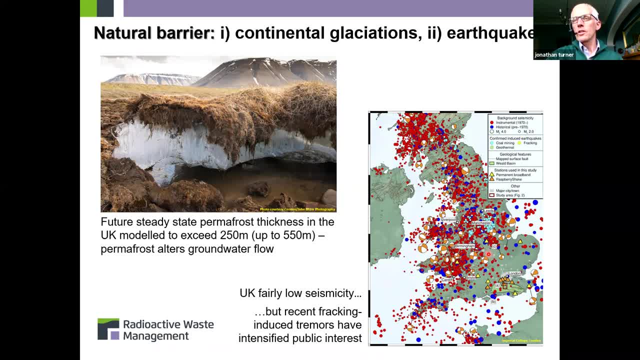 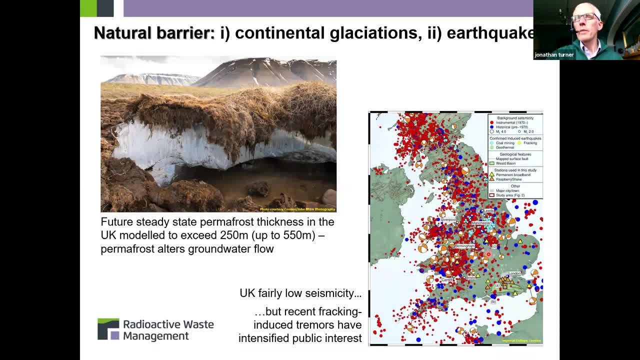 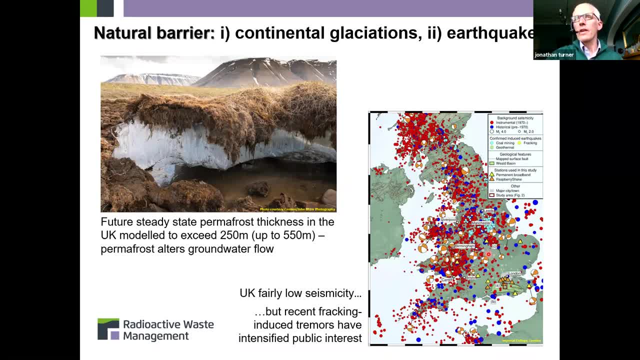 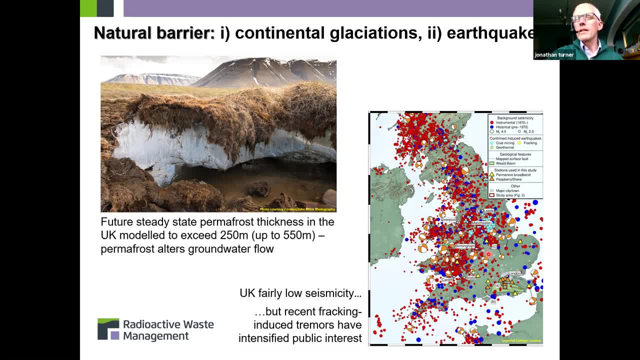 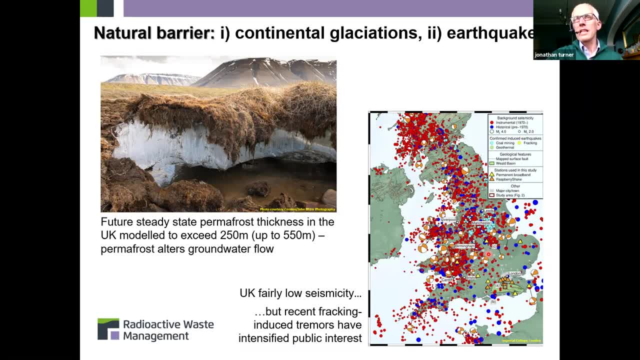 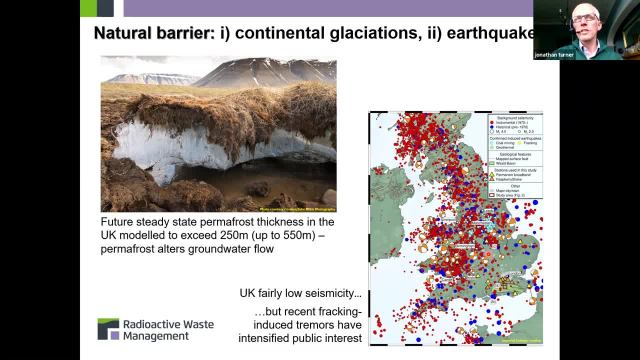 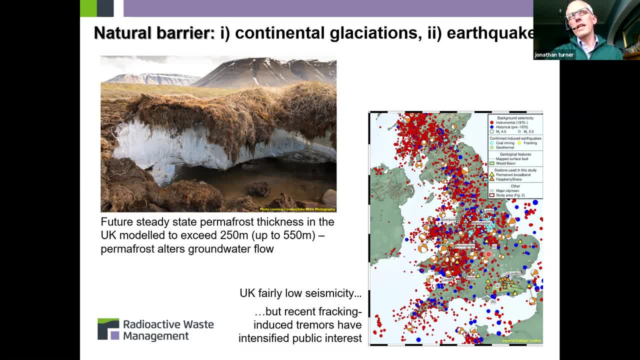 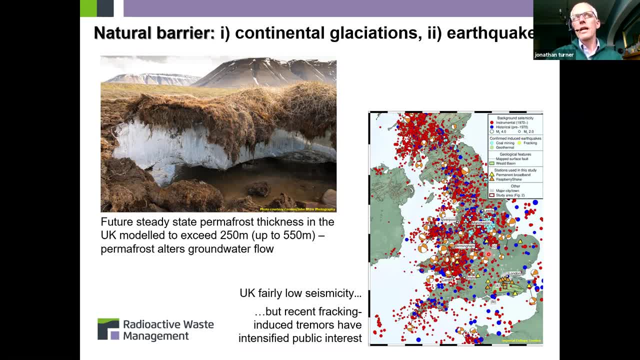 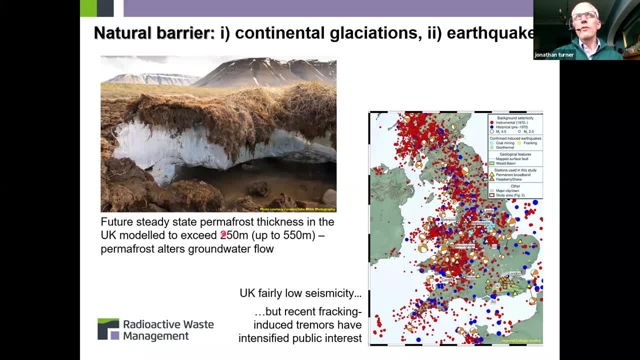 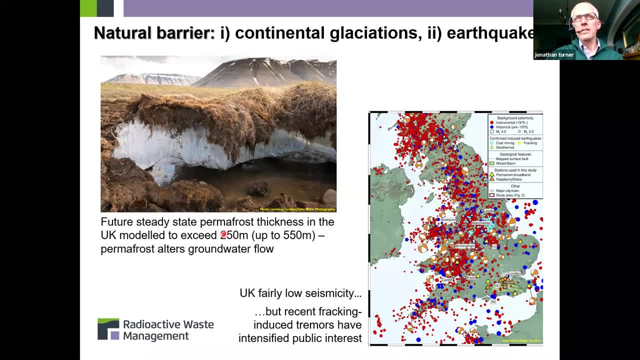 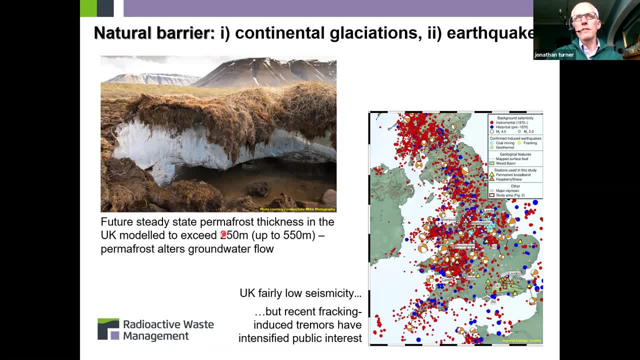 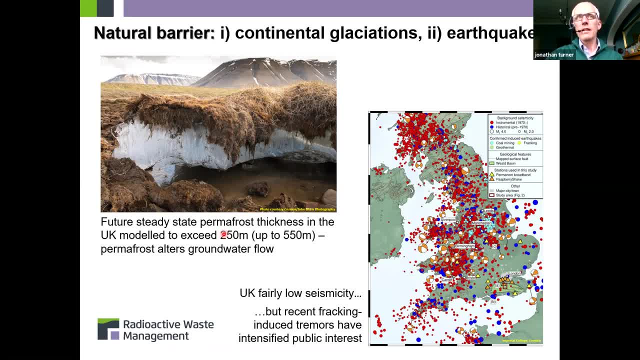 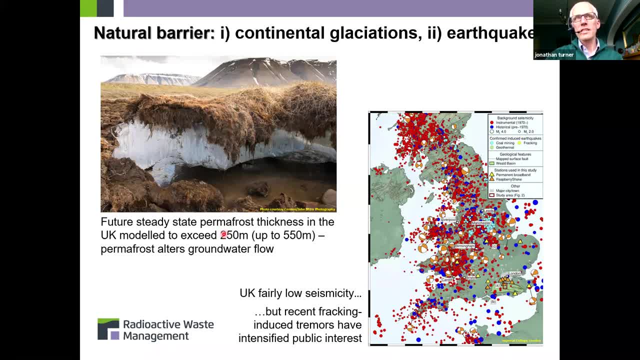 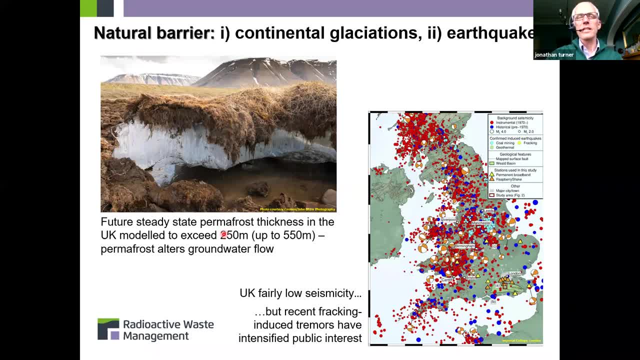 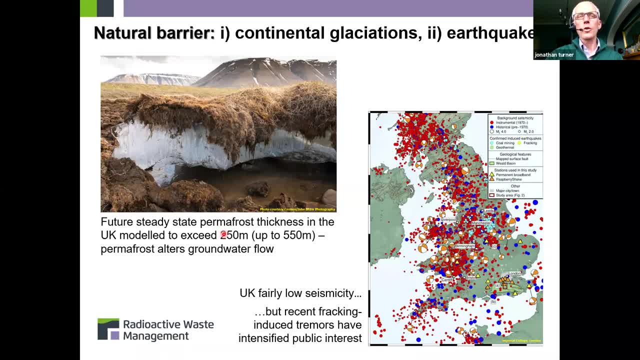 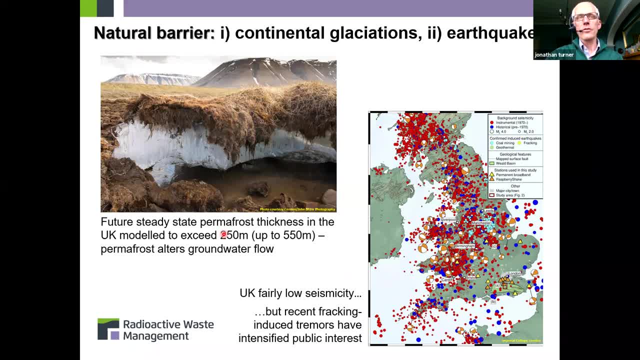 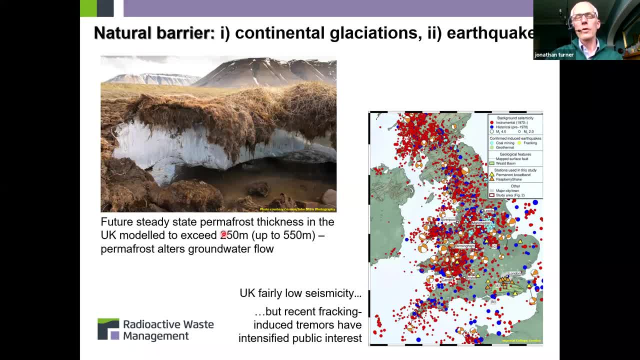 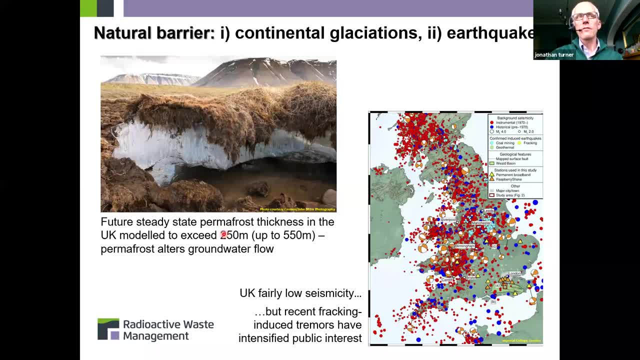 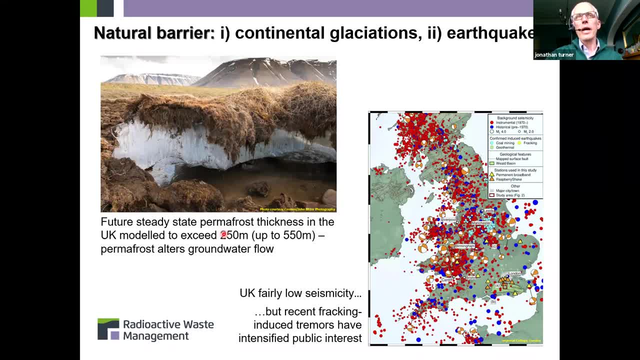 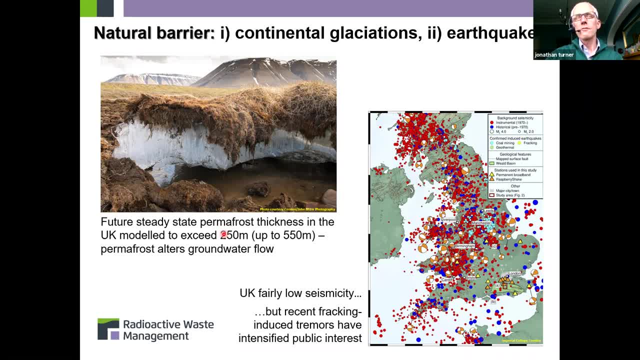 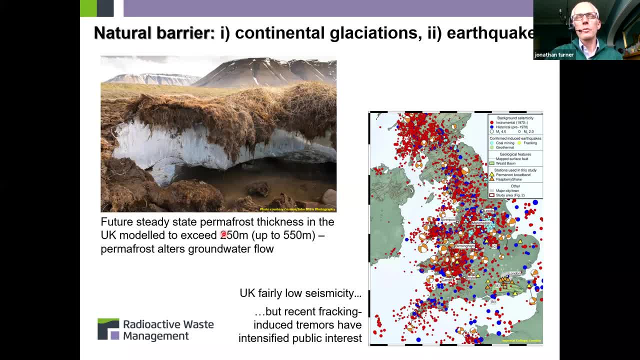 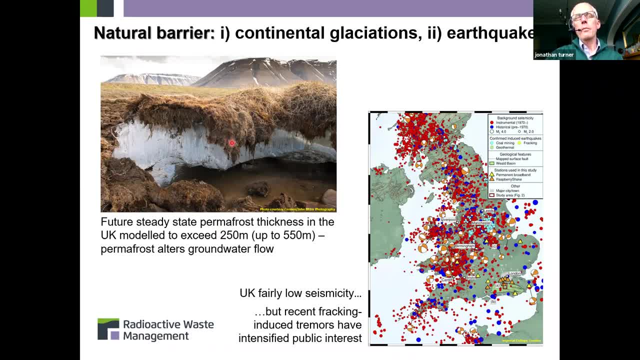 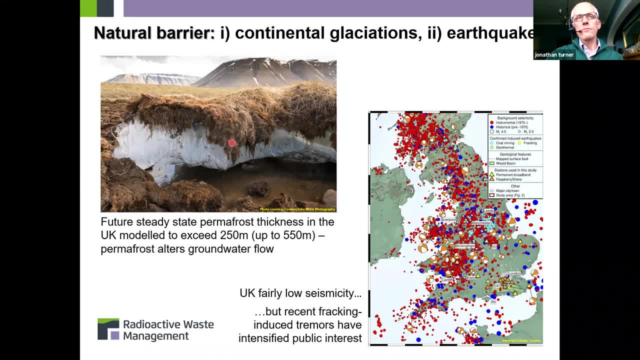 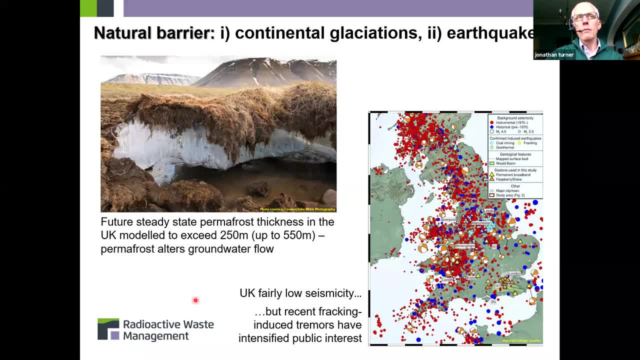 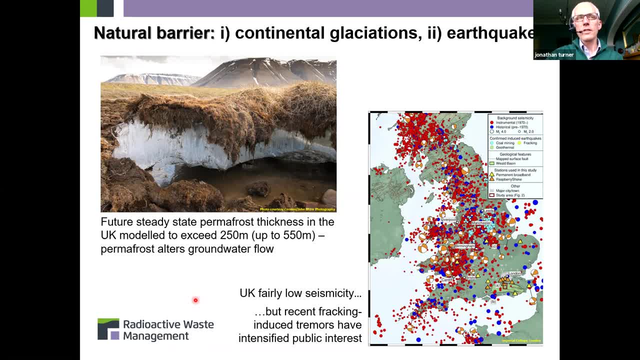 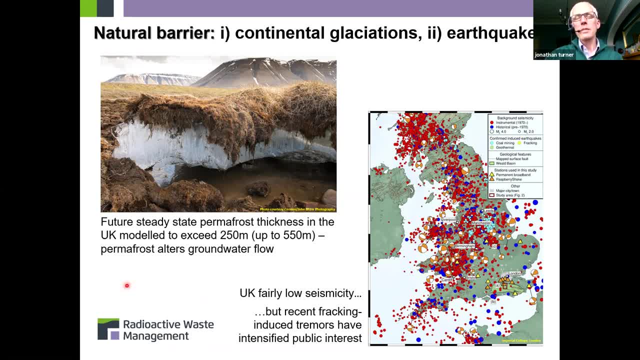 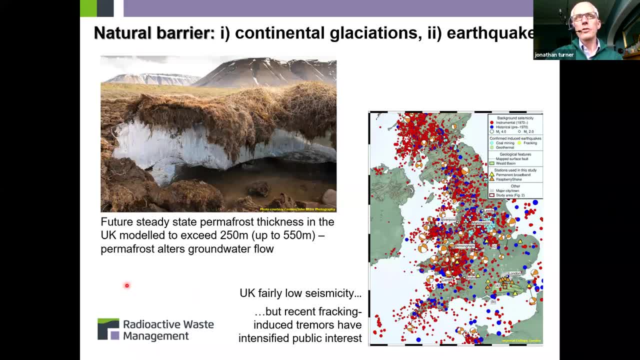 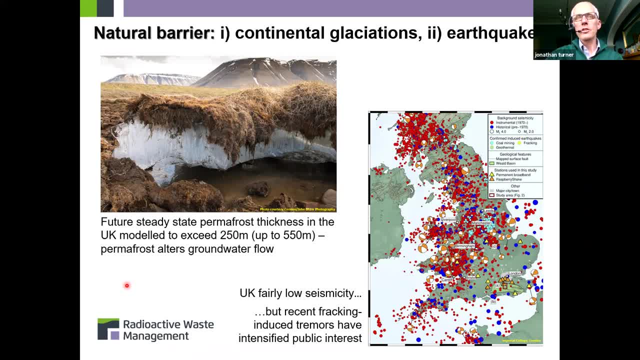 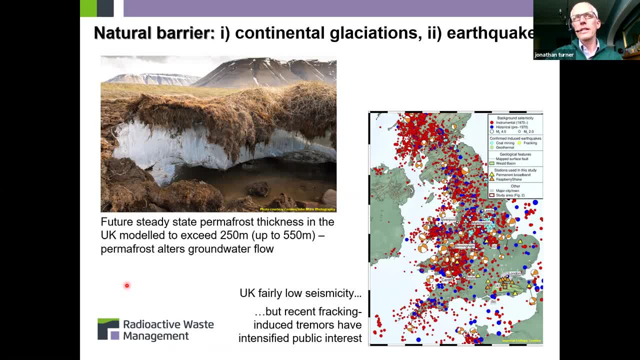 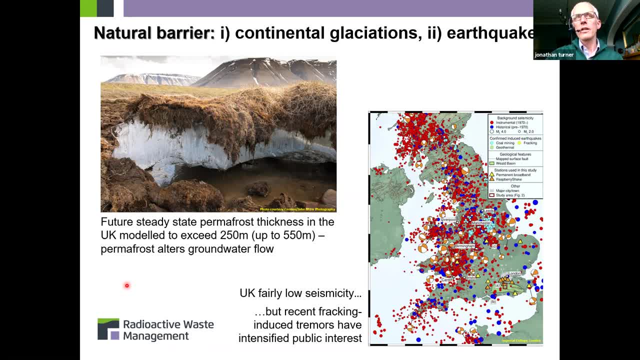 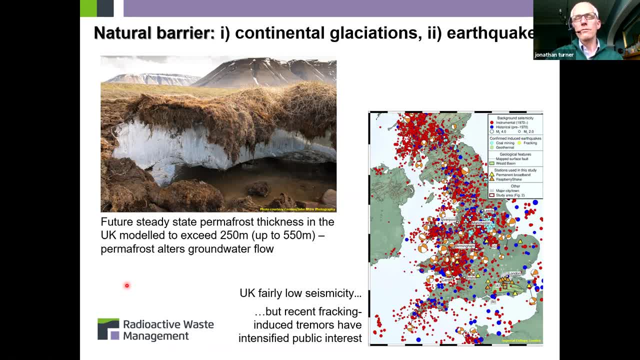 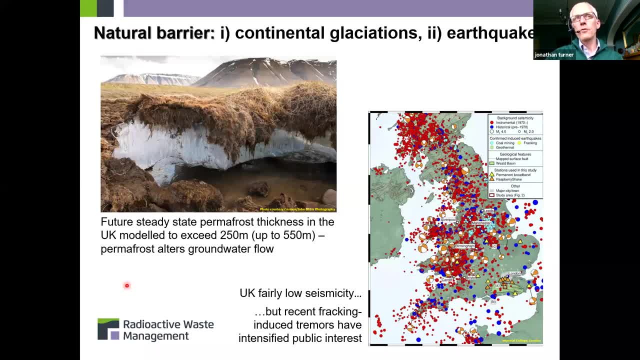 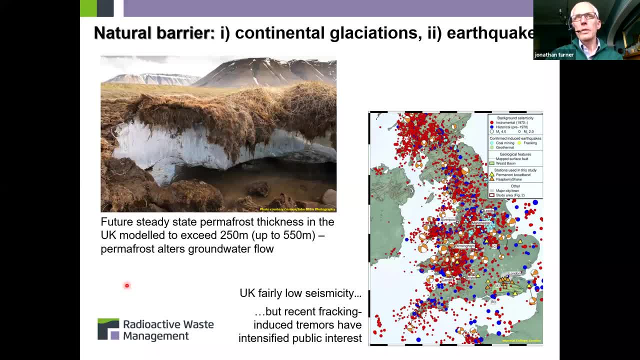 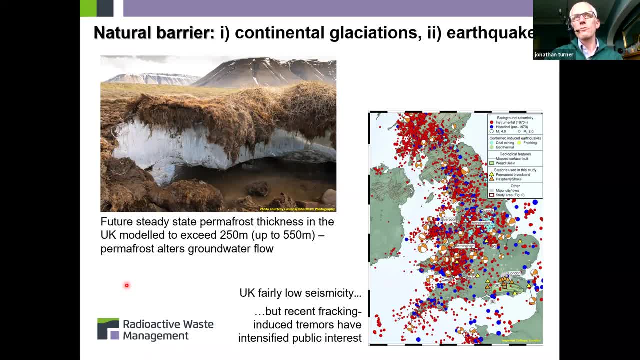 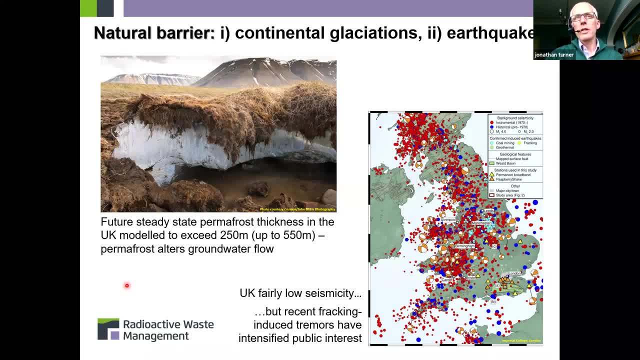 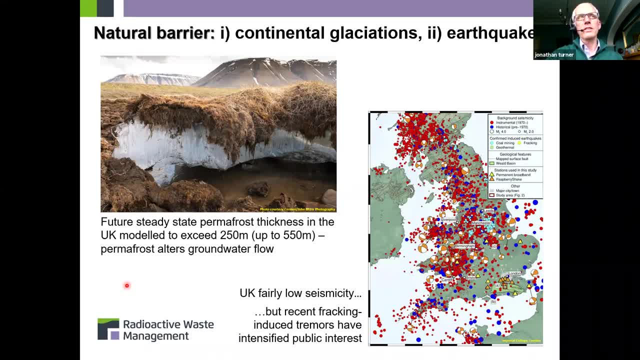 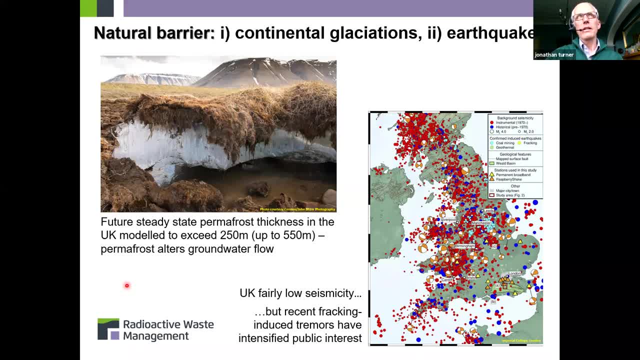 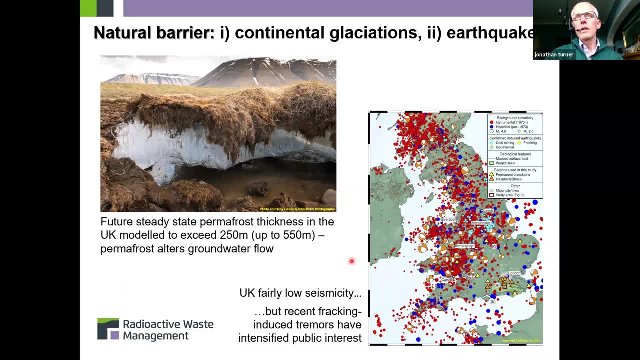 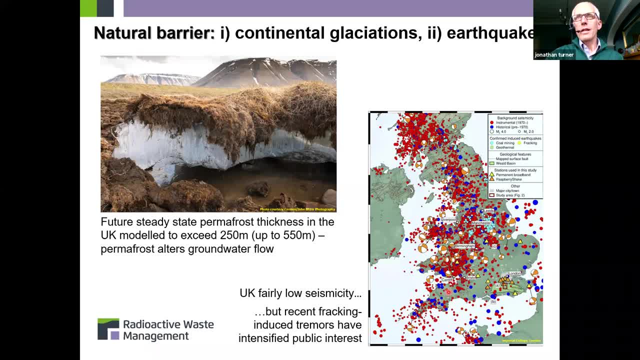 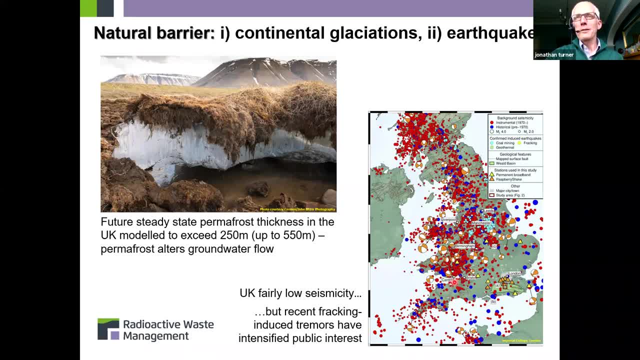 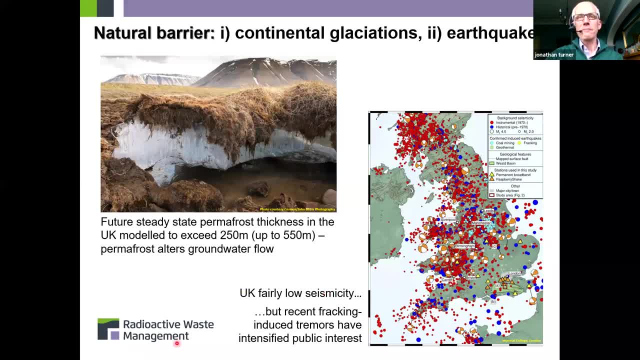 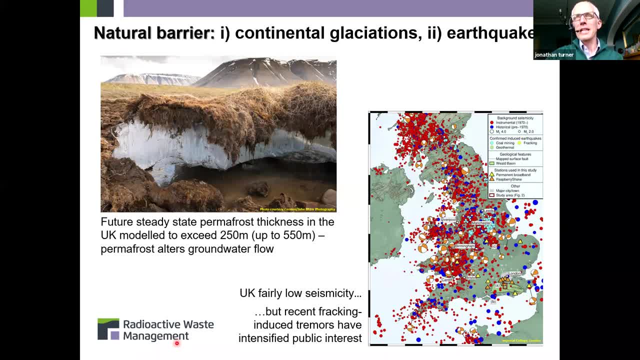 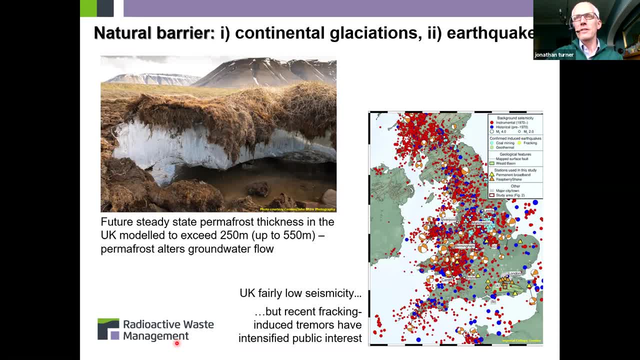 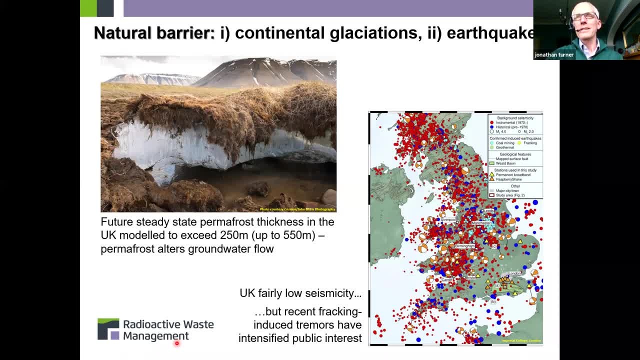 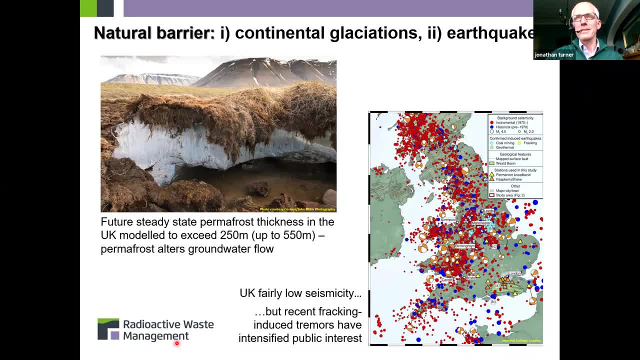 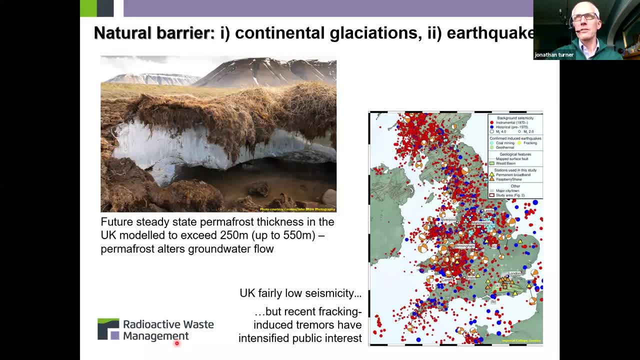 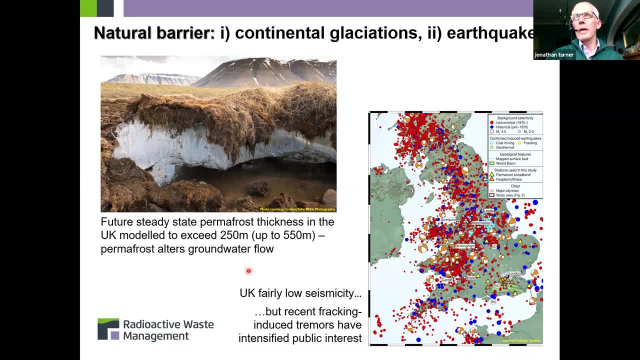 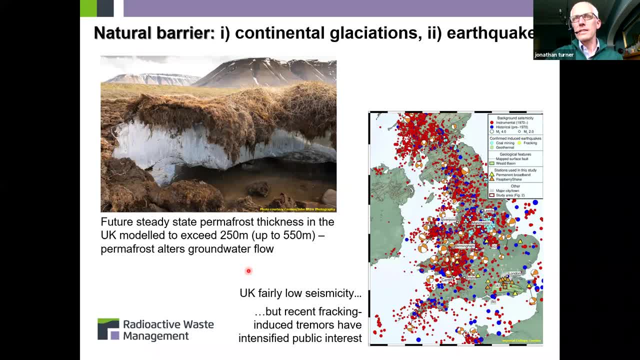 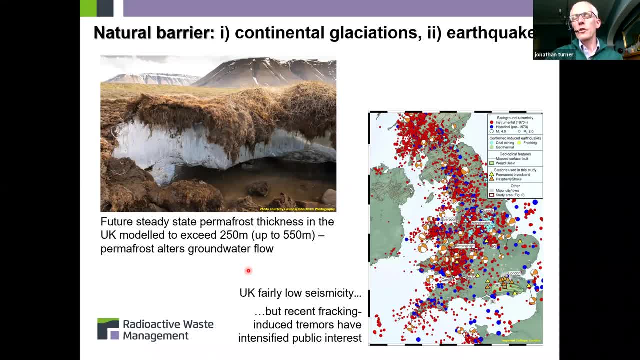 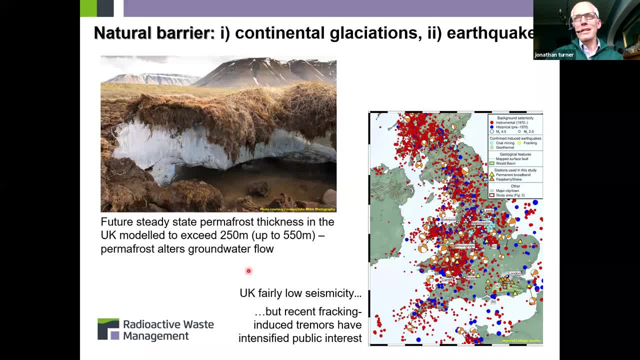 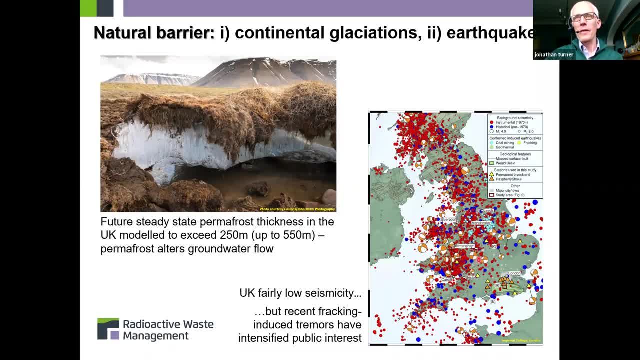 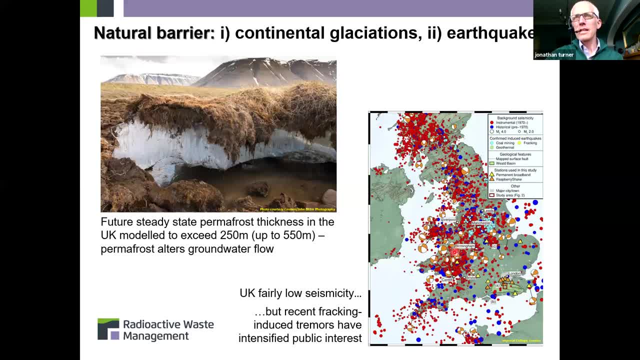 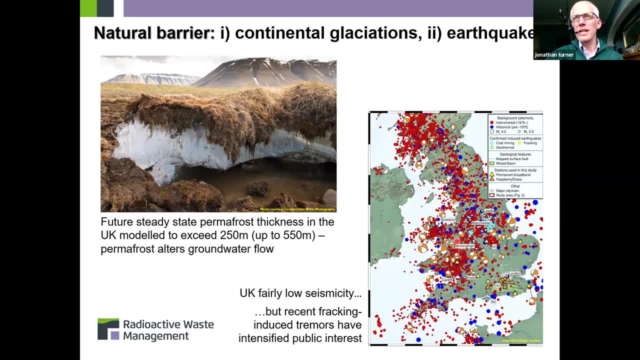 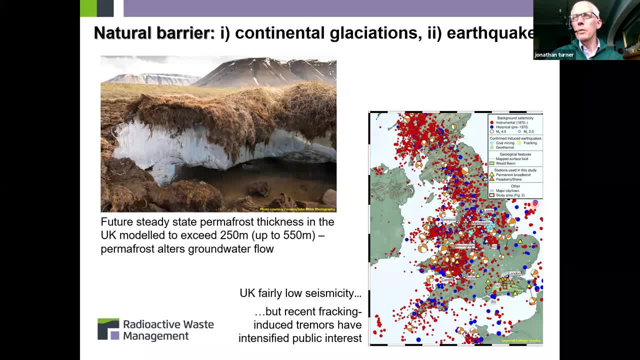 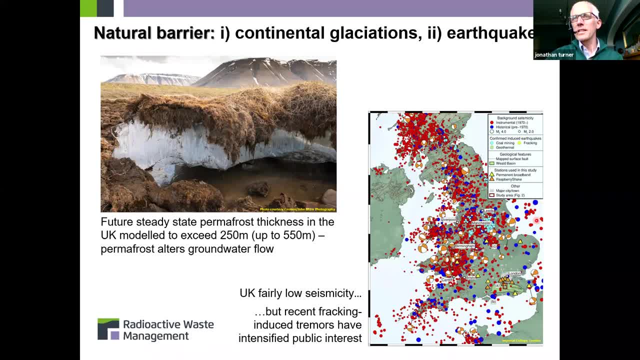 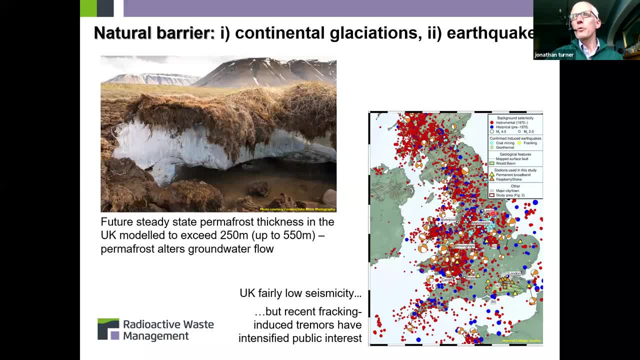 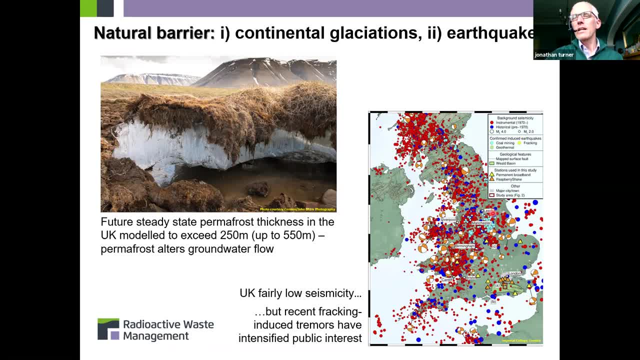 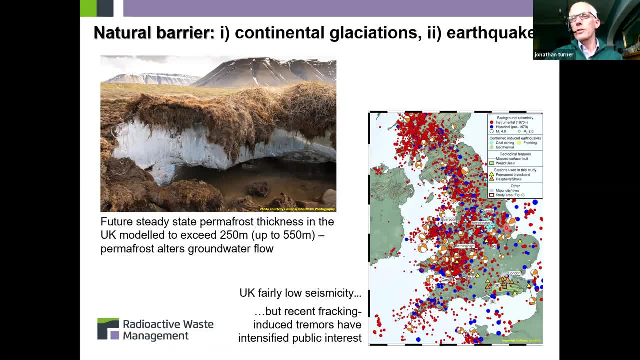 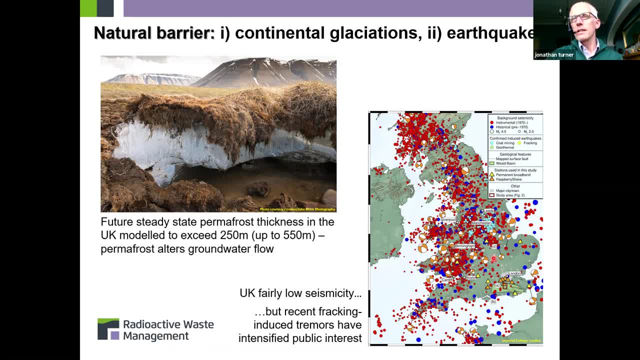 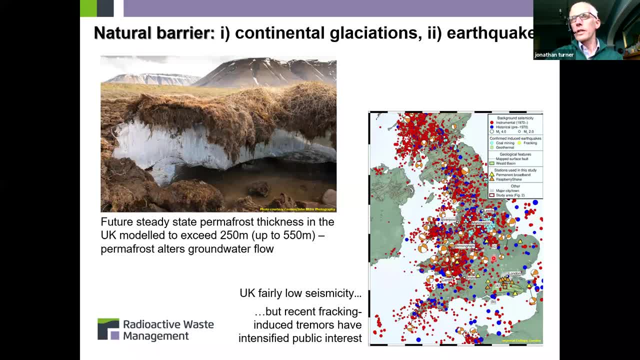 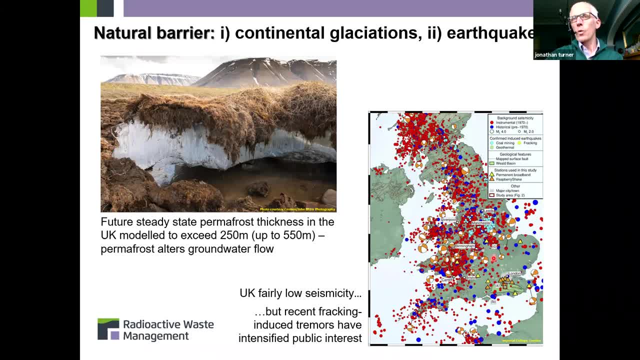 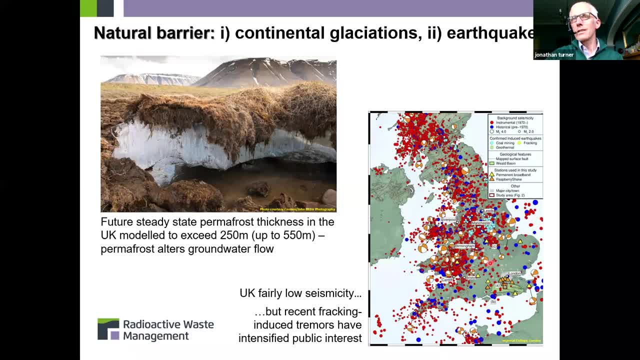 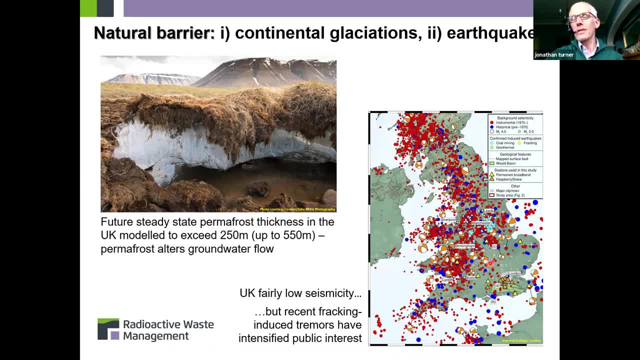 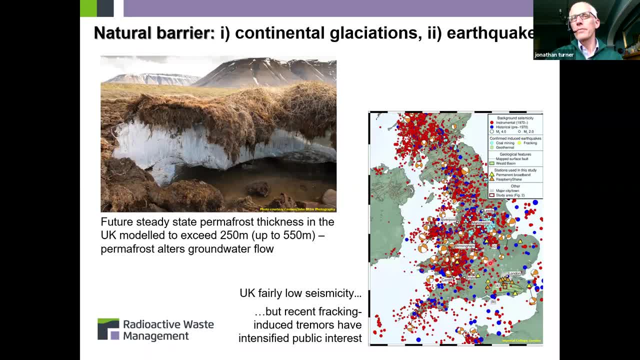 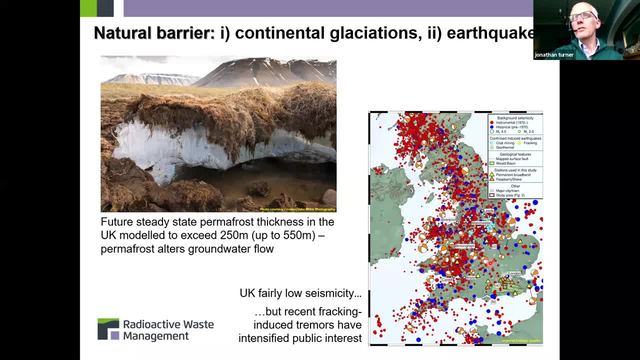 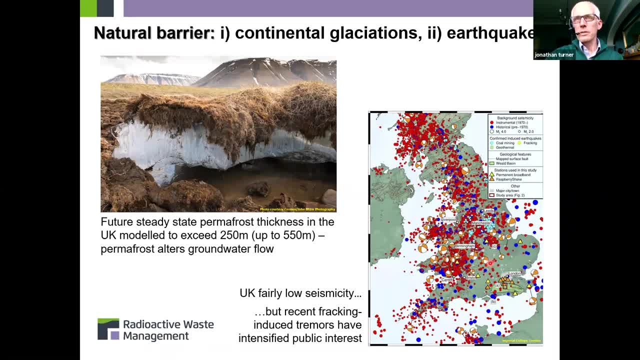 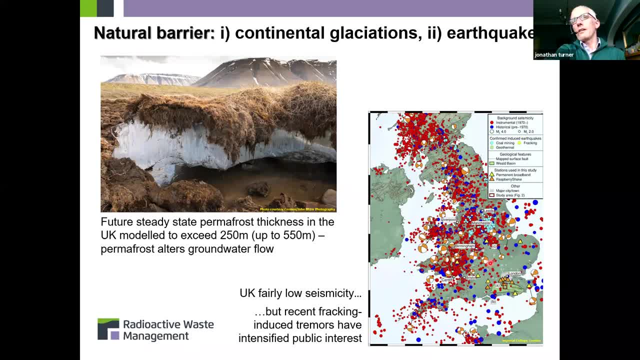 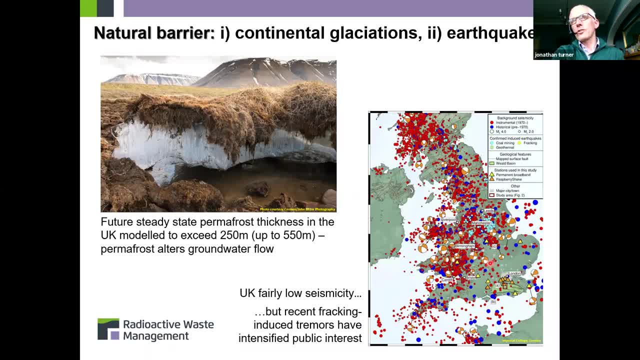 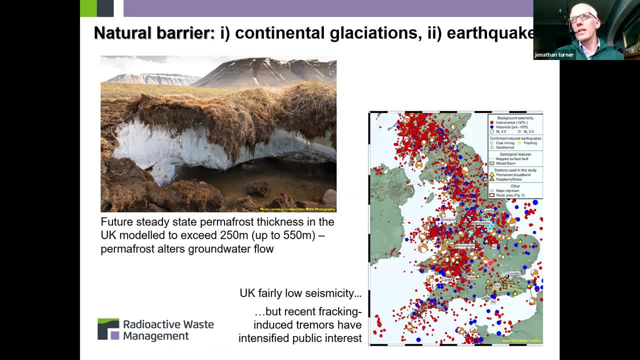 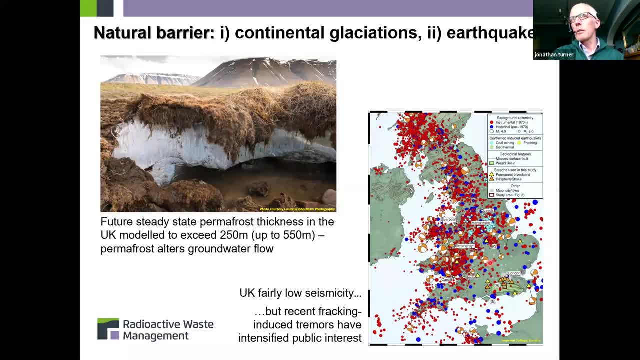 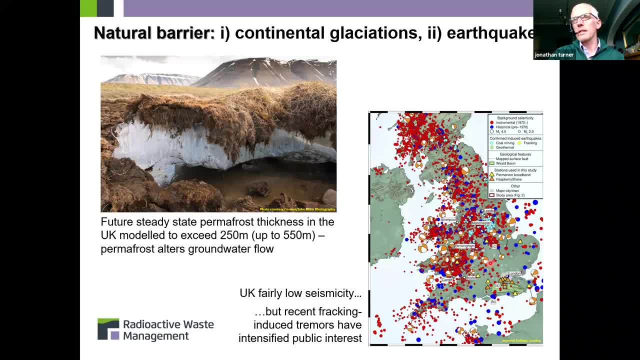 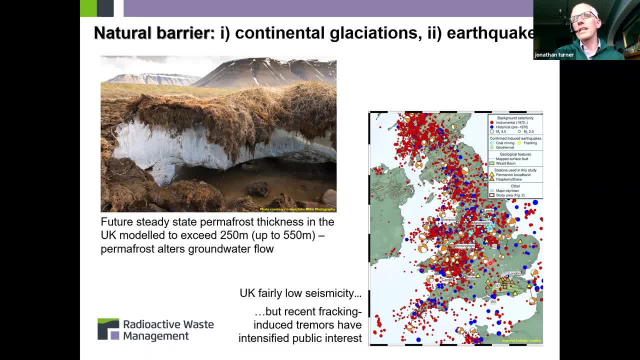 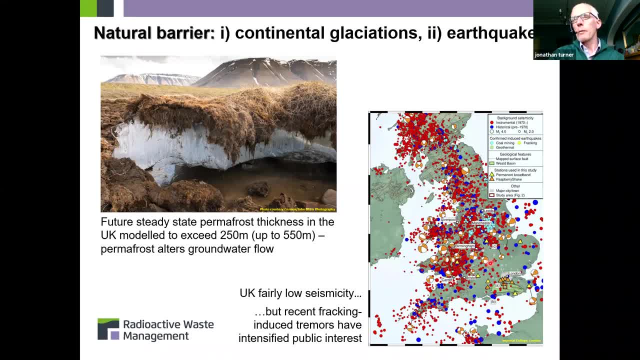 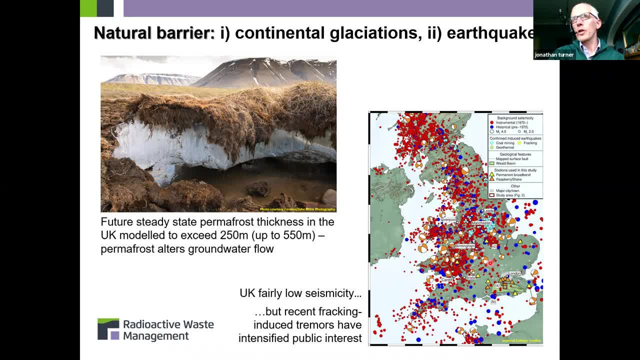 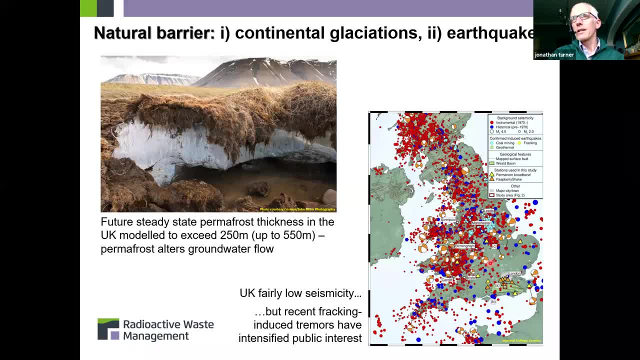 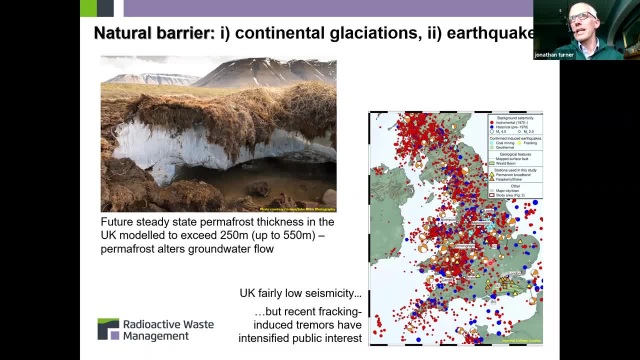 This is called a Hall, which was the world's first gas cooling reactor. This is called a Hall, which was the world's first gas cooling reactor, just to communicate very clearly what a gdf is and also what it isn't, and similarly, the exploration work, the borehole drilling, the seismic work that will go on in order to 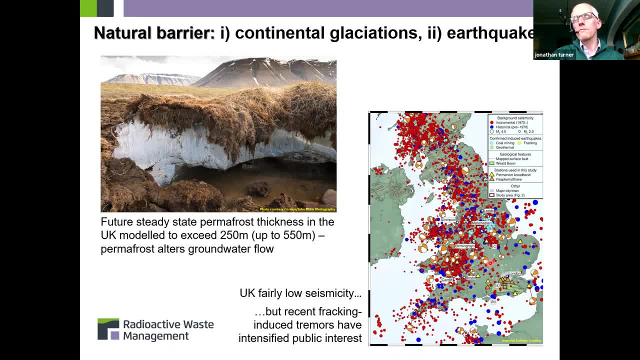 in order to investigate possible candidate sites for a gdf. but i go back to the point i made earlier about one of the key functions of gdf and the key requirements of gdf being isolation: isolation from surface processes like glaciations, but also isolation from from earthquakes. the 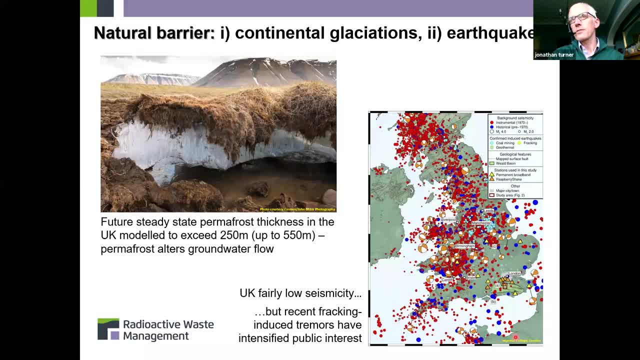 impact of an earthquake in the subsurface clearly very different to the shaking impact that you get on the surface. that's not to say that once we start to converge on real sites and we start to develop bespoke safety cases based on site-specific information, we will need to do an 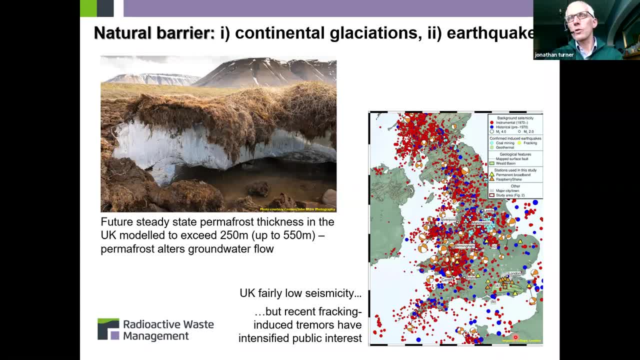 enormous amount of work, including what's often called probabilistic seismic hazard assessment, to understand the likelihood of earthquakes in the areas that we're investigating, the possible impacts of those earthquakes, not just on the gdf but of course also on the surface facilities, which will be open and handling waste for um for something like 100 years. 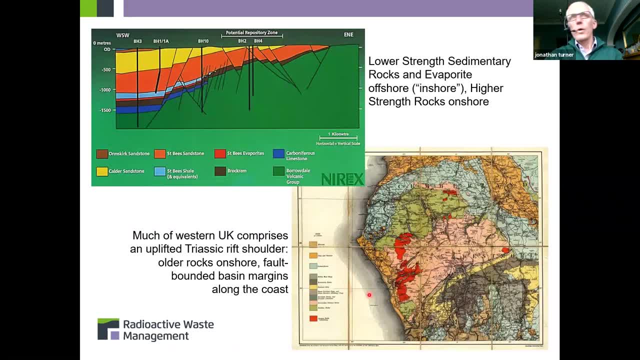 so i'm just going to give you a little bit of time to talk about that and then we'll get back to you with more questions very quickly, because i'm aware of the time. uh, just to say a little bit about the communities that we're presently engaging with. this is all public. so since, uh, september of last, 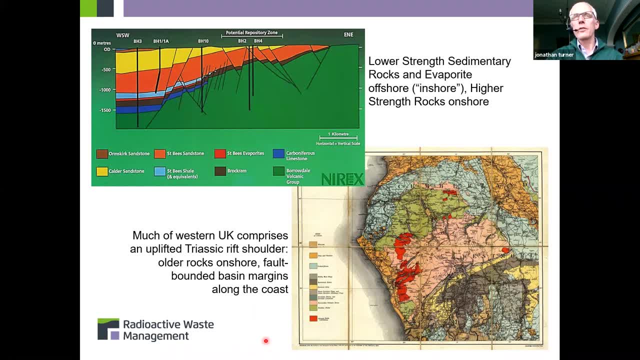 year, last year, we have developed what are called working groups with two boroughs: uh in west cumbria, copeland to the south and allardale. uh to the north um geology of cumbria and allardale to the north um geology of cumbria. 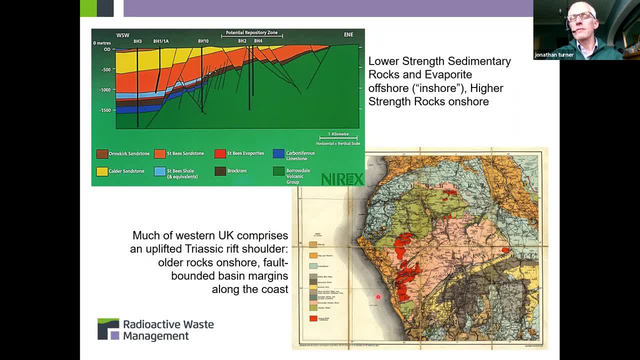 and allardale to the north. um. geology of cumbria, Really summarized by my caption here. very different geology as you step off the coast into the Irish Sea compared to what you see on shore. Basically old, mainly paleozoic rocks that make up onshore Cumbria. contrast that with younger triassic rocks. 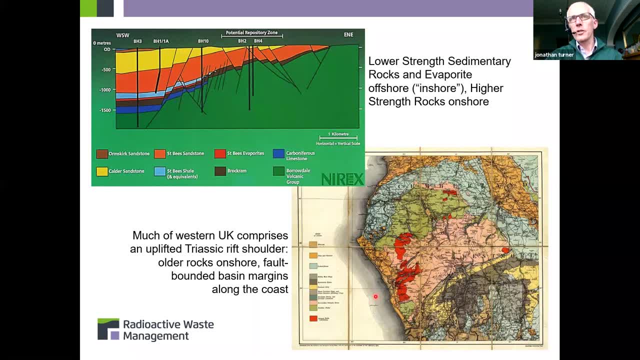 And particularly, you can imagine, we're interested in the Mercia mudstone out in the Irish Sea. I should say that for both those working groups, both Copeland down in the south and Allardale up in the north, from the outset of these engagements with communities, the Lake District National Park has been out of bounds. 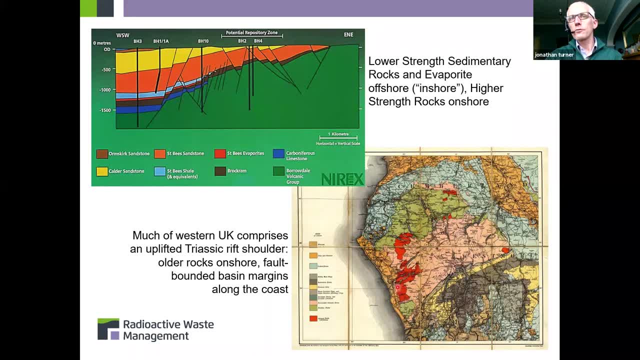 So we're looking just at the fairly narrow coastal fringe. In fact, the Lake District National Park does actually tag the coast down here, So we're looking at the fairly narrow coastal fringe between the National Park and the coast and the offshore area out in the Irish Sea. 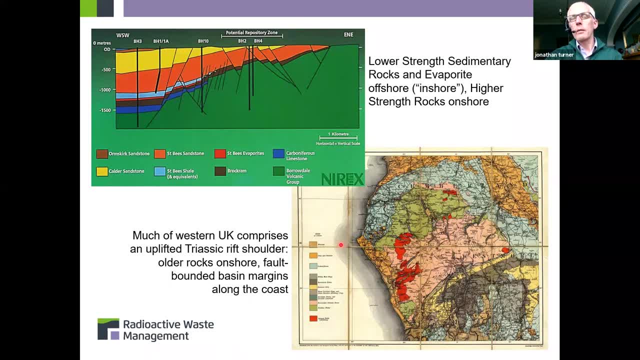 Where the Mercia mudstone dominates, possible host rocks in which a GDF could be constructed, And that kind of geology is shown in this simple cross section here, which I dug out deliberately because it's got NYREX on it. Some of you might remember investigations in Cumbria undertaken by NYREX in the 1990s. 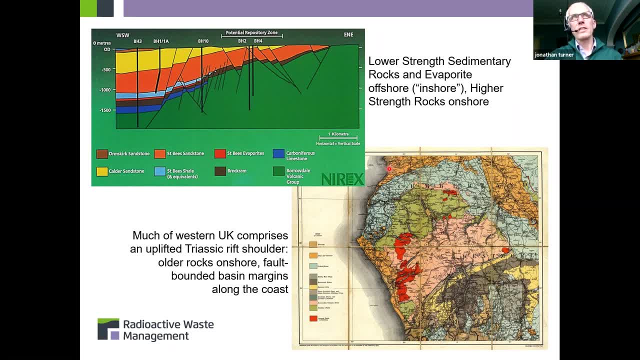 They were proposing to build what was then called a rock characterization facility, essentially an underground rock laboratory, And the Borodeo Volcanics which you can see here, is a rock characterization facility, For example around the old man of Coniston, are shown in the green as a basement here. 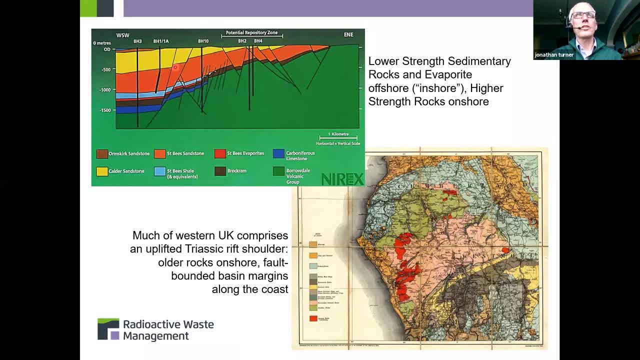 And then, as we progress westward out into the Irish Sea, we can see this younger trisic stratigraphy that is almost absent on the onshore area, except for along the along the coastal plain. I've talked about the Mercia mudstone. 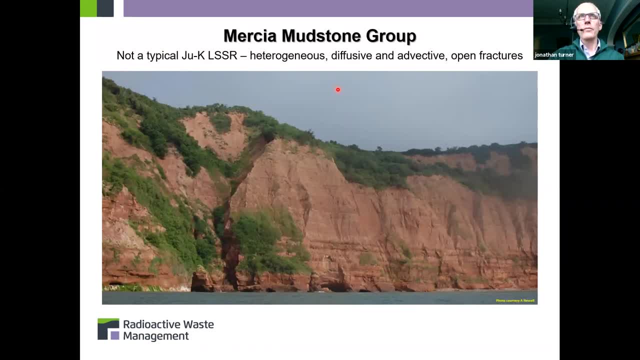 Lots of lessons that we can learn from countries like Switzerland and France, both of whom are building there, are going to develop their facilities In middle Jurassic Oxford clay type lithologies. We are looking in a lot of detail at the potential of the Mercia mudstone off the west coast of Cumbria. 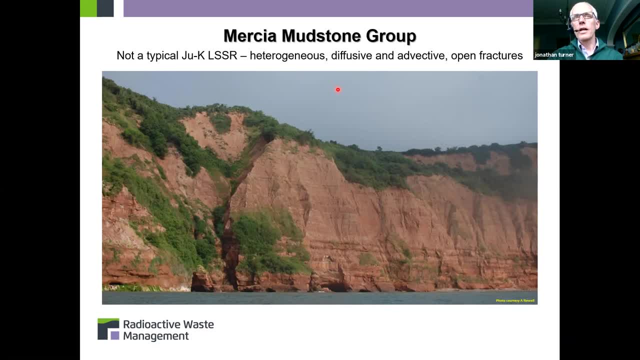 And just make a simple point here that the Mercia mudstone probably, fair to say, more complex than Jurassic Cretaceous clays. It's formerly been buried more deeply and therefore it's more brittle. Therefore it sustains open fractures. 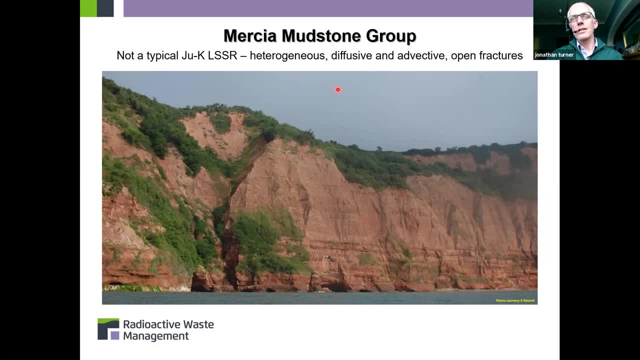 You get open fractures in the subsurface, Unlike fractures in the Oxford clay which tend to heal and naturally seal. It's a lot more heterogeneous than Jurassic Cretaceous clays And, because of what I said about fractures, the potential not just for diffusive flow but also advective flow. 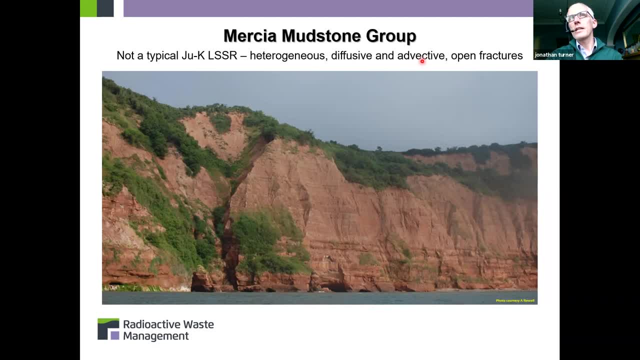 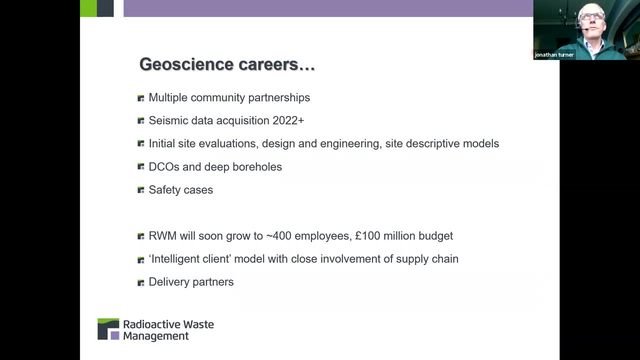 In other words flow of gases and liquids through natural fractures in the rock. I said I'd finish off just with a few words About geoscience careers And you can read the words for yourself here. But just to make the point that in really quite a short space of time things are changing very rapidly, not just for RWM but for the UK Deep Geological Disposal Program. 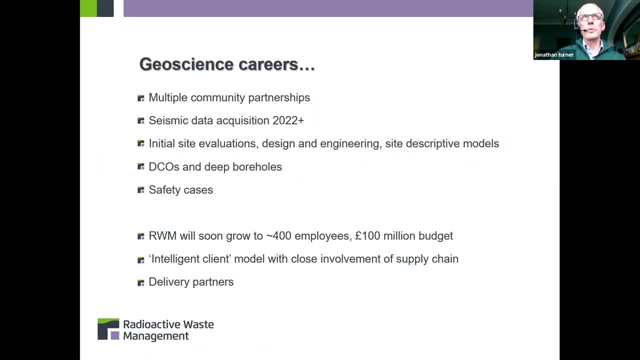 We now have, as I've described, two working groups, Copeland and Allerdale. They will evolve hopefully into community partnerships, which is the point at which we start The government's start Making paying community investment funding into those communities. 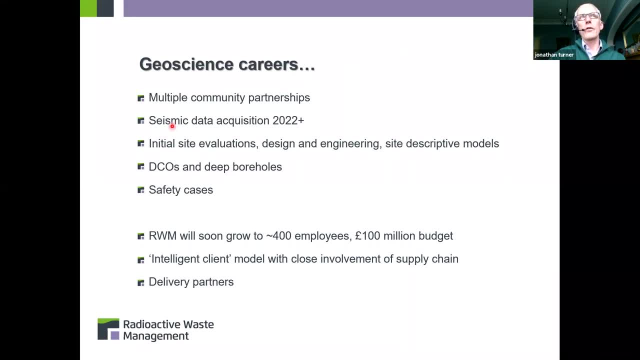 We are likely to be acquiring seismic data 2D and 3D in the Irish Sea of Copeland and Allerdale summer of next year. That will then lead to initial site evaluations based on bespoke site-specific data, Beginning to develop bespoke design and engineering solutions, beginning to think about development consent orders. 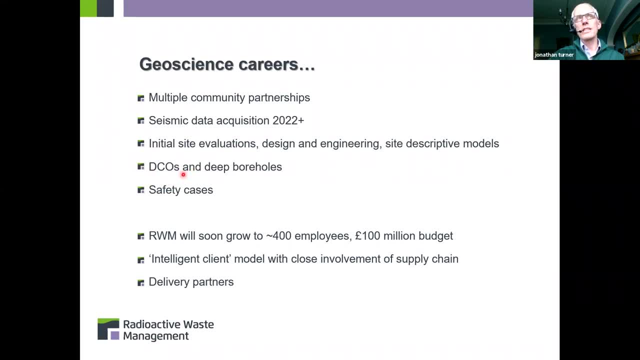 the permitting process through which nationally significant infrastructure projects like GDF are permitted, safety cases and so on. So the overall message from this is things are changing very rapidly for RWM And, whilst we're likely to remain as a company of about 400 to 450 employees- and, as you can imagine, by no means all of those are geoscientists- 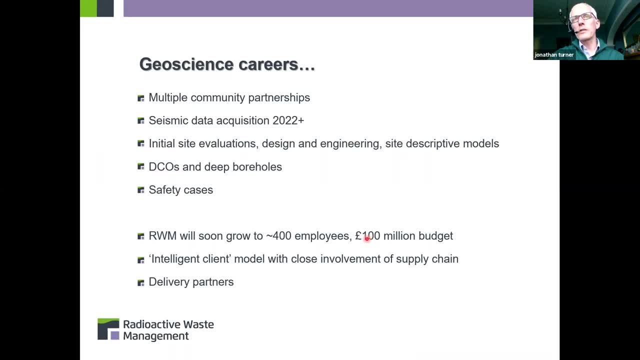 our budget will soon be up around the £100 million, And that's going to mean that we're going to have a small army of people out in the supply chain, including in strategic delivery partners, who will be doing a lot of this work for us. 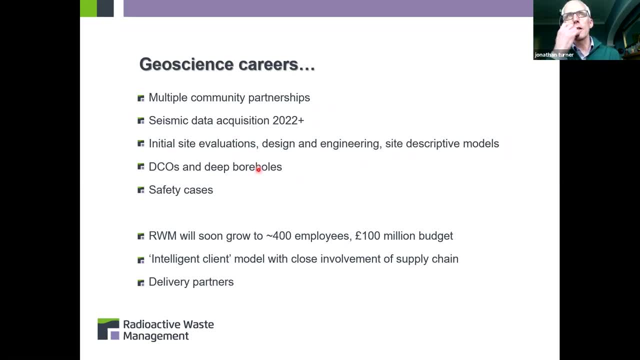 So I think there's going to be a lot of opportunities for geoscientists with the deep geological disposal program going forward, And I'm happy to answer questions on that. So I think my last slide is just making the point about. you know, keep an eye on our website. 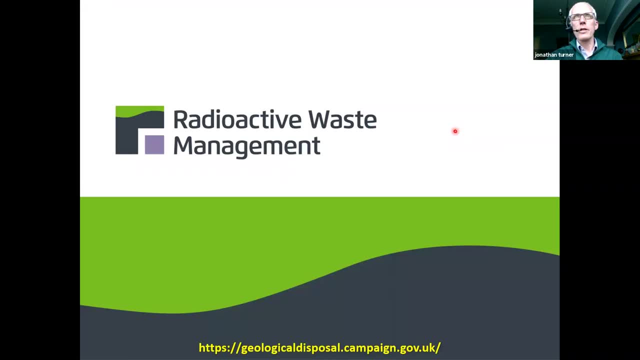 about how the campaign goes. It's a very dynamic picture at the moment. Watch this space this year in terms of further working groups that we're hoping to announce, And I think that pretty much wraps up, Ray, what I wanted to say. 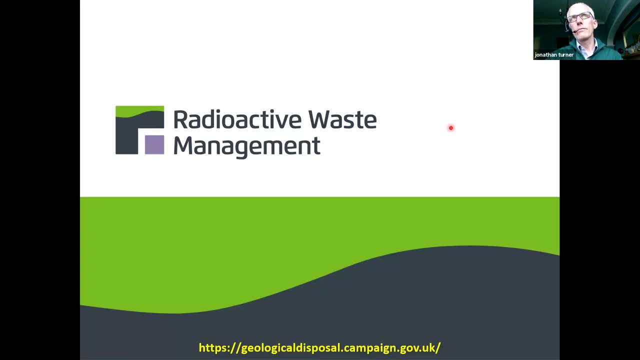 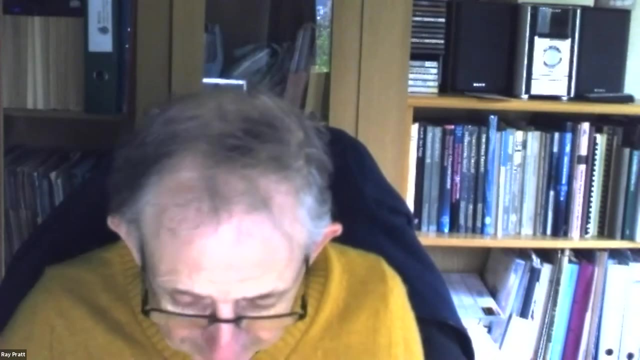 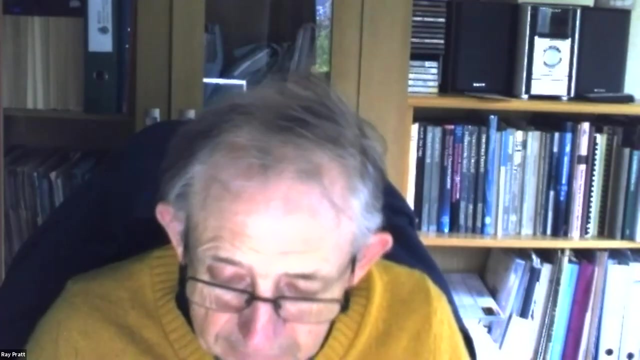 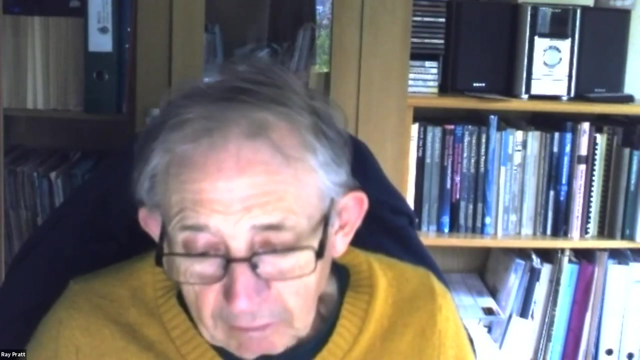 And happy to take any questions. Okay, well, that's really great. Thank you, Jonathan. We haven't had any questions typed into the chat Just yet, But I'll start off. How many do we really need, A to deal with our current inventory of waste and B forecasting, let's say, for the next 50 years? 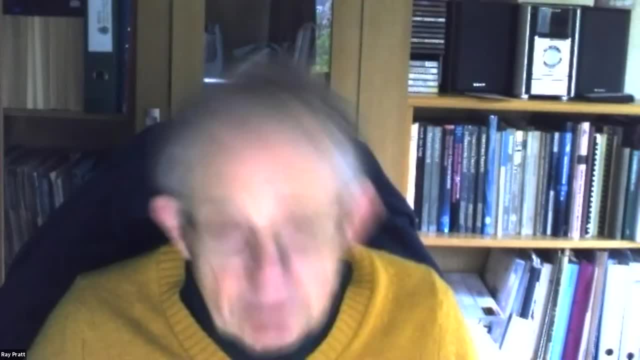 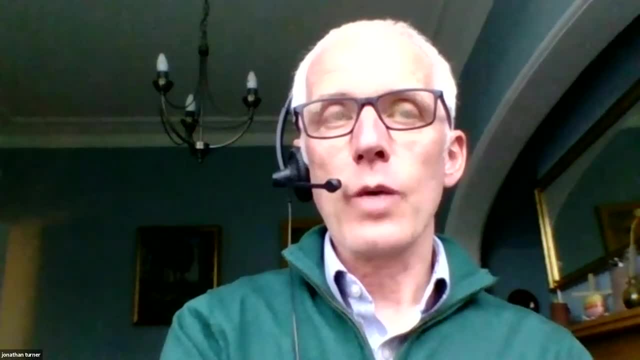 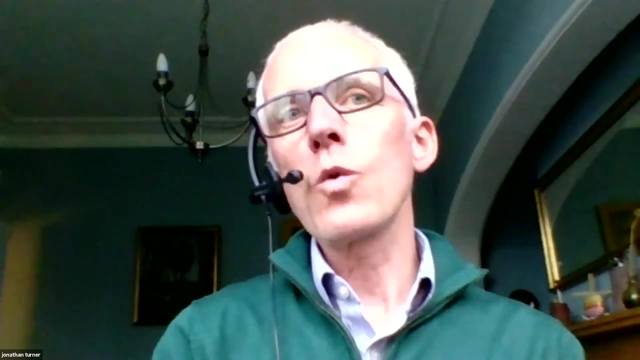 Yeah, the surface facilities are up to 2 kilometres squared, But that's that sort of artist's impression, as I called it, of a single GDF If we were to accommodate all of the inventory, which is about 750,000 cubic metres in terms of package volume. 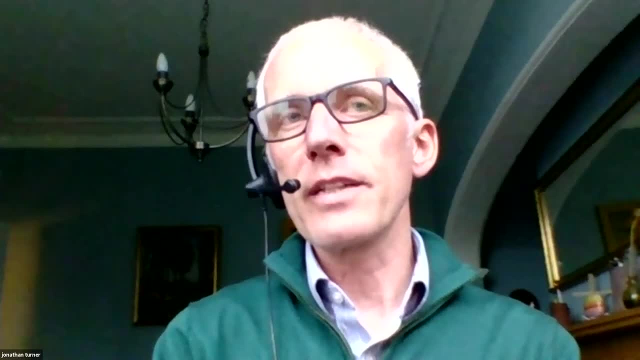 if we were to accommodate all of it in one GDF then it would be about 20 square kilometres. But I think you know I go back to the point that I made at the start. But I think you know I go back to the point that I made at the start. 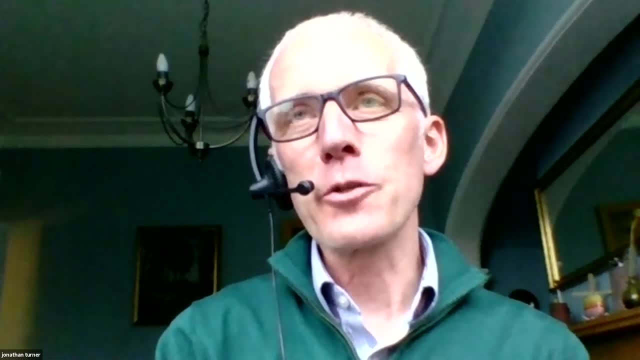 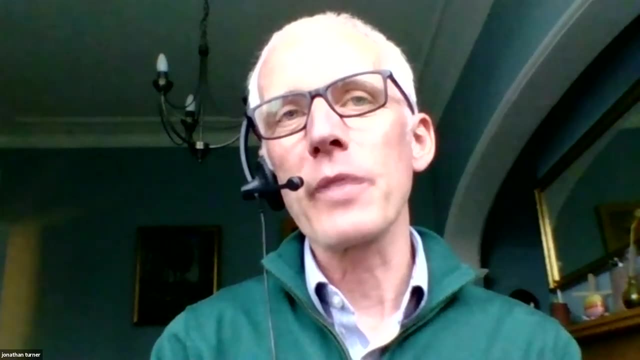 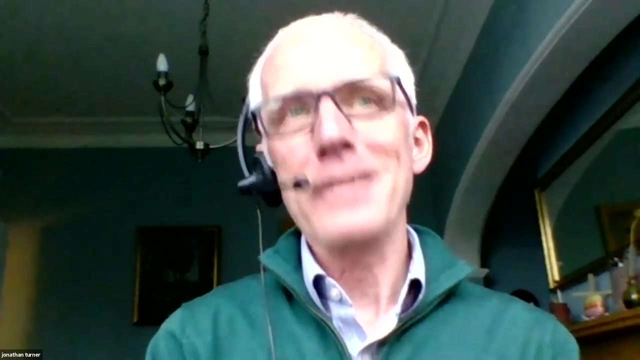 start until we know a community and therefore geology and surface conditions, onshore, offshore, etc. we're keeping our options open And among the options that we need to keep open is the possibility that we might need several GDFs. The government and we would like to have 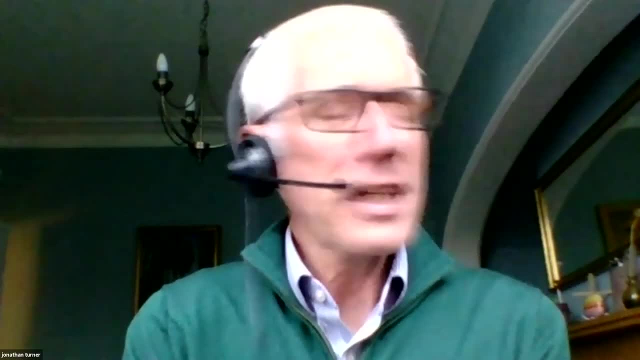 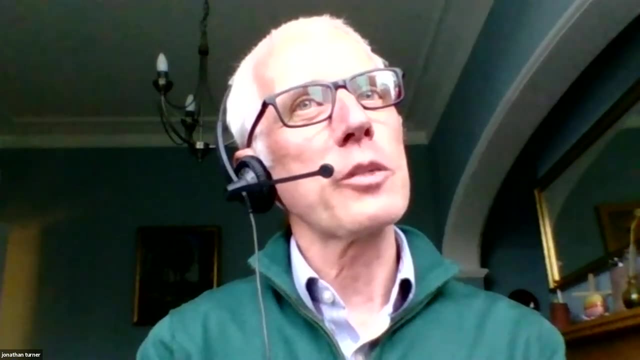 one GDF. but for example, I mean just completely hypothetically- what if we were engaging with a community whose geology wasn't particularly suitable for the intermediate level waste, should we say just for example, but worked for the high heat generating waste? I don't. 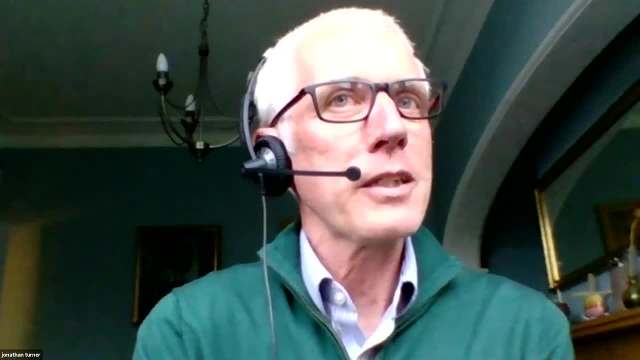 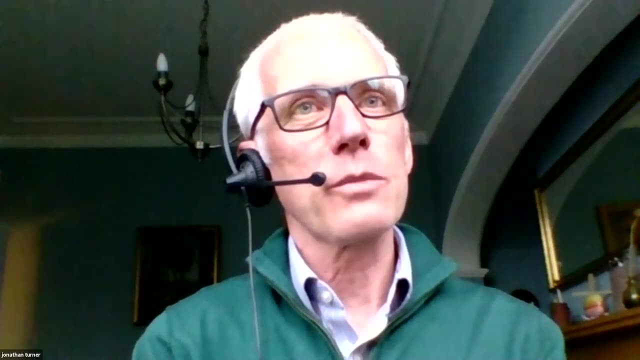 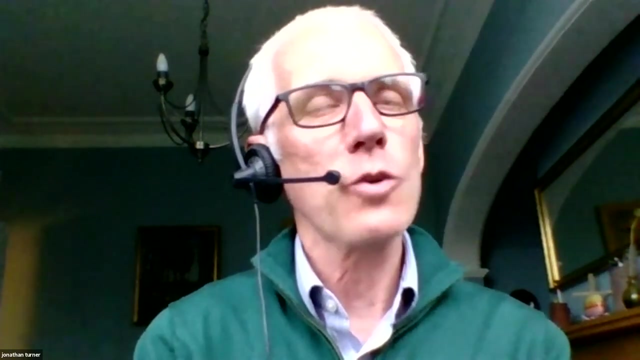 think we would walk away from that situation because the bird in the hand is the willing community, So everything is open. but certainly in terms of national expedience and value for money, I think one GDF would be much better. But the one to two square kilometres was just. 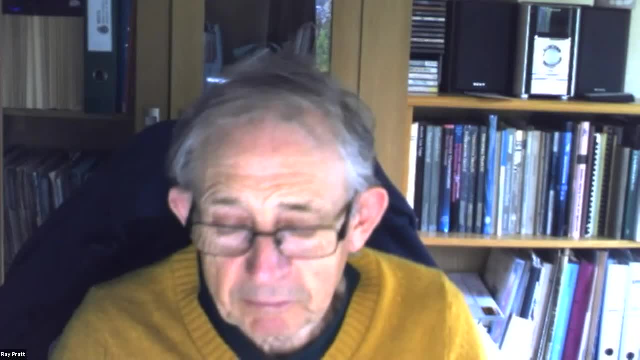 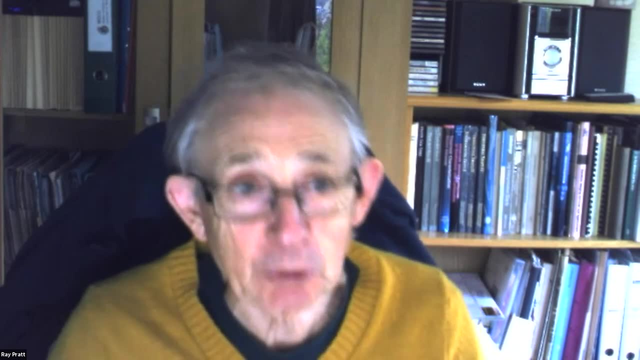 for the surface facilities. Thank you, Right, But I'm thinking you know 20, a 20 kilometre underground facility is huge, About four. by yeah, I mean 20 square kilometres. so about four by five, Yeah. 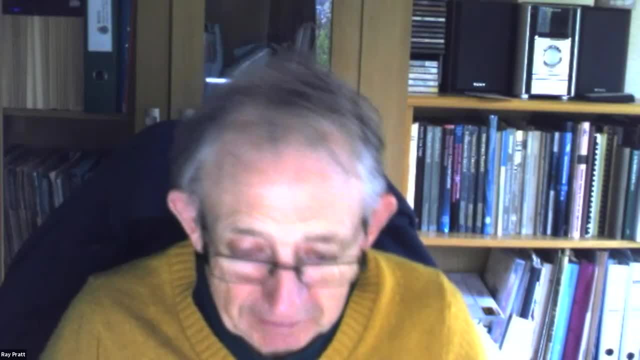 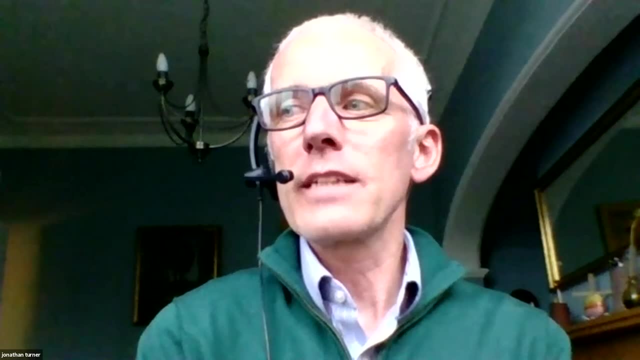 Okay, But it's still a huge hole you've got to excavate and engineer. Yeah, yeah, Oh, yeah, Yeah, And that's why there's there is now, and it will only increase a strong push on ensuring that the only material.